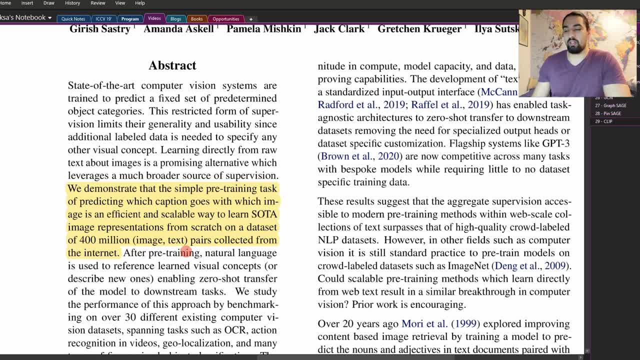 on a data set of 400 million image sex pairs collected from the internet, And so they also introduced this new data set, because all of So that's open AI. They really are bullish on computation, and all of the existing data sets weren't leveraging the scale as much as they could. 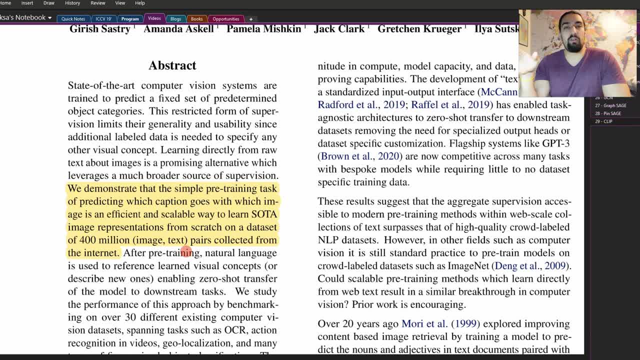 And especially since mostly most of the computer vision tasks are benchmarks. data sets like ImageNet are only associated with a simple structured label, and they just want to associate images and text, so they had to create their own data set. So, without further ado, let's jump into the method itself. 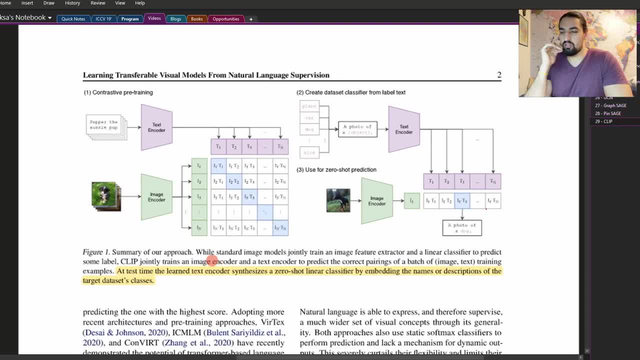 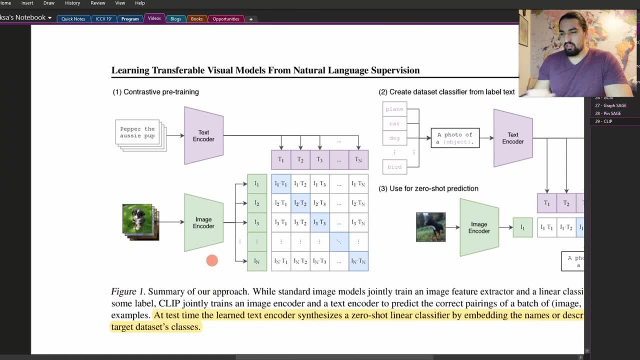 And I'll explain it in depth. I'll start doing some high-level explanation and we'll slowly dig deeper into the method. Okay, So this is how it looks like. Basically, what they do is the following: So they have, as I said, associated. 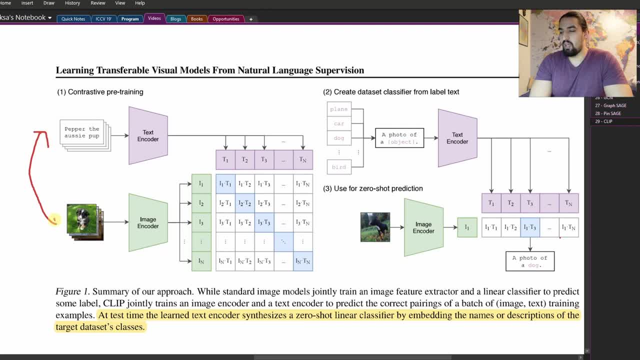 They have associated image text pairs. And the way The thing they do is they first do some data augmentations here for the image part, and then they have image encoder and they have text encoder, And here they just used ResNet and the newly introduced vision transformer. 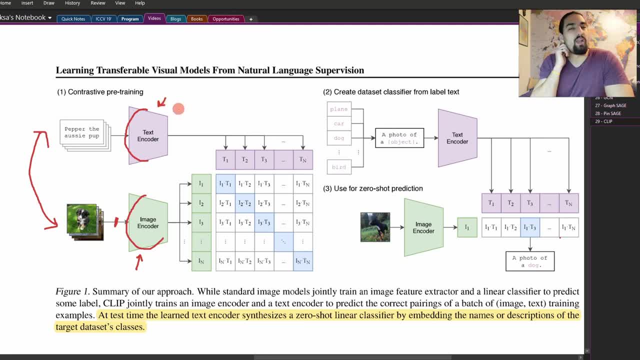 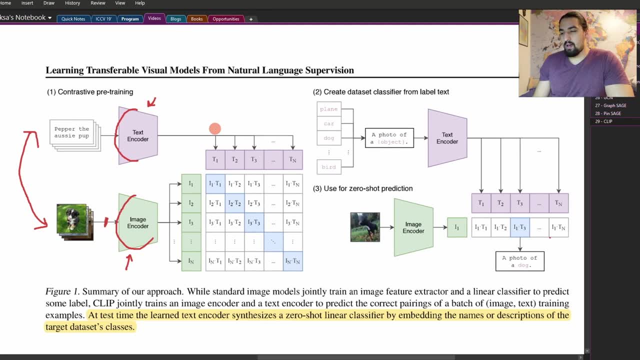 whereas for the text encoder, they just used the original Vaslany transformer with certain modifications. they did for the GPT family of models as well. And once you have that set up, what you do is the following. So you take the text sequence and you just encode it. 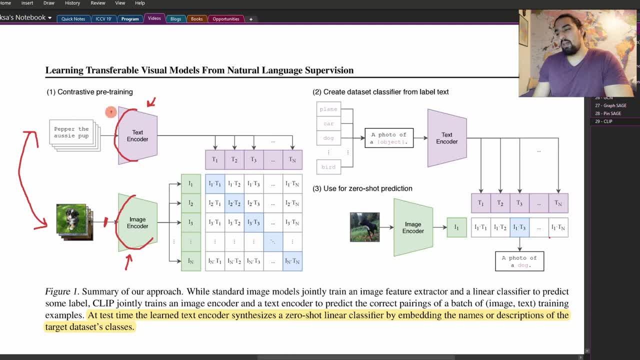 And how do you do that? Well, because this is transformer. so you basically just embed the text sequence here and you just take the start of sentence token and you take the end of sentence tokens and you place them. You just bracket the text sequence using those. 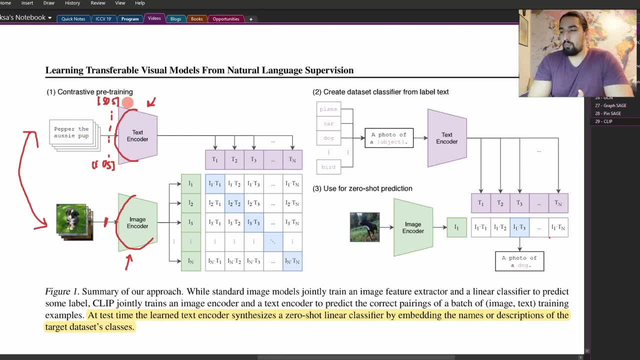 And now, if you know how the transformer works- and I hope you do so- you just have the forward pass through the transformer and whatever comes out from the last layer of the transformer above the EOS end of sentence token, that's the representation they're going to use. 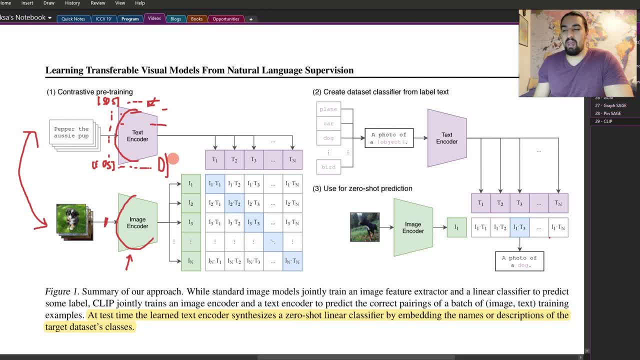 So they just do some simple layer normalization here and they project this using some linear projection layer into the embedding space. and we're here. So 1 through n is just the size of the batch. So these are the encodings we get for the text, sentences, sequences. 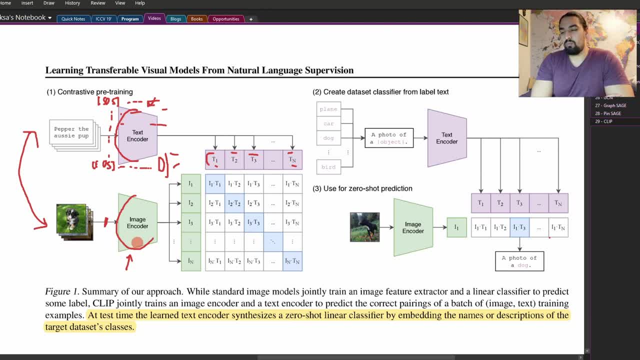 On the other hand, image encoder is pretty straightforward: You basically feed through the image and you get certain representation at the output. So if this was resonant, you'd probably just take the output at the after the average pooling part. 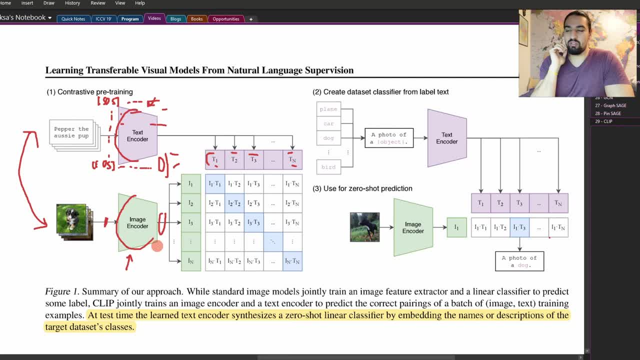 whereas they did some modifications with resonant. I won't get into those details right now, But yeah, you can imagine, you just take out some certain representation after that pooling part and you use that as your image representation. You also do that linear projection. 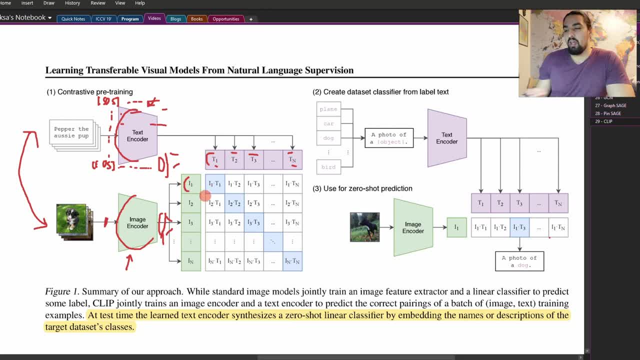 and you're finally inside this contrastive embedding space. So once we're here, we basically on the high level. we just want to make sure that this image- image 1,, has the highest cosine similarity with this text embedding vector T1.. 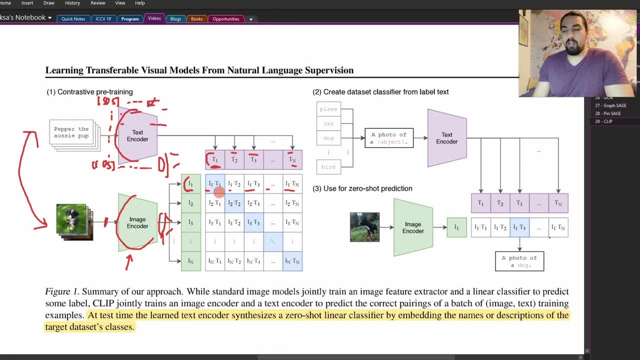 And you want to push all of these down to 0. And you want to do the same thing along this column. So you want to make sure, because we have asymmetric setting here, We have on one side, we have textual information. 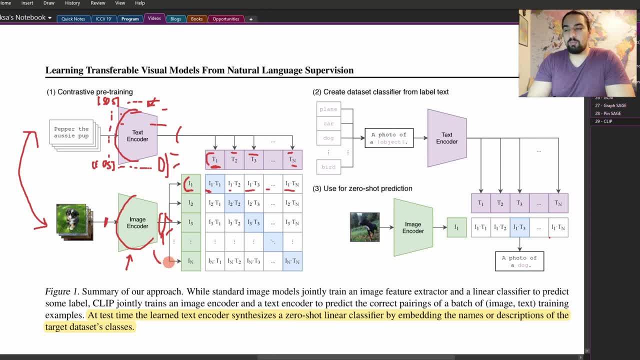 and on the other side, we have visual information in our embedding space. So this is a multi-modal embedding space, And so they do it both ways. So they want to also make sure this one goes up to 1, and all of these are pushed down to 0.. 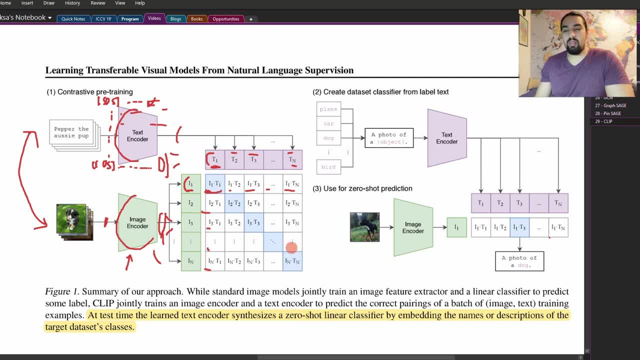 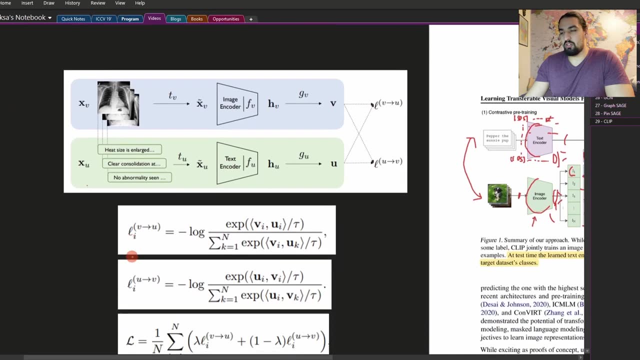 And you just repeat all of that across the batch and that's it. Now let's get one level deeper and see how this exactly works. So this paper was heavily inspired by this Convert paper that was working on medical images, and they actually achieved some really awesome results. 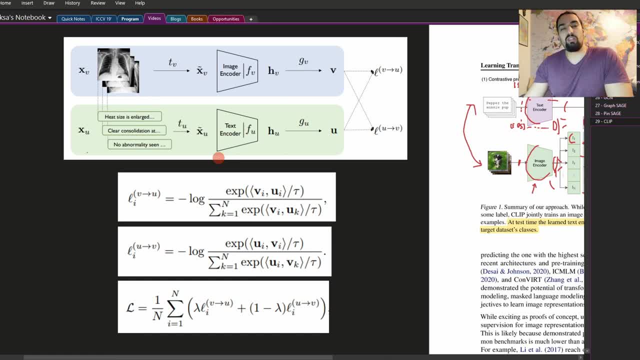 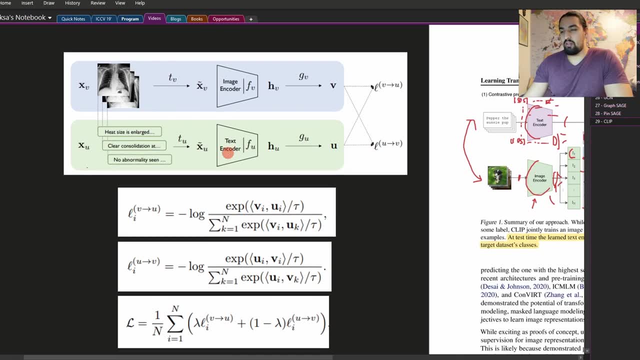 So the visual features they trained using their method proved to be really good at some downstream medical tasks. So you can see how the pipeline looks like and it's the same thing as I just explained. So we have a sequence of images. 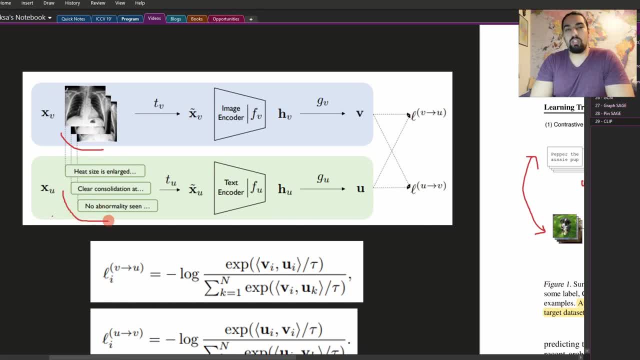 and sequence of associated textual sequences. And basically what they do is they do data augmentations, which is a really, really popular thing to do in these contrastive learning methods, And they did some textual augmentations, So just extracting single sentences. 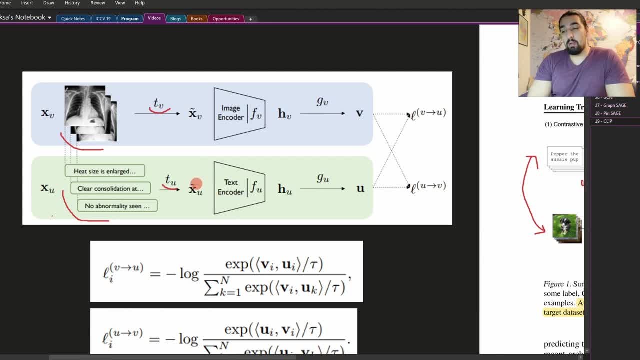 from their text sequences. So this paper, on the other hand, ditched this thing here, because most of the images they had had only one single sentence associated with the image. So they can't just remove the sentence, Otherwise they'll lose the supervision signal. 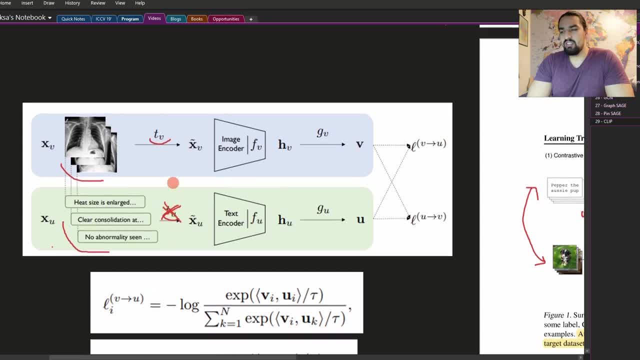 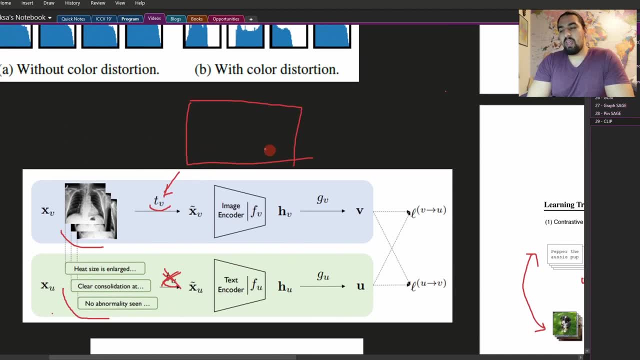 So they just ditched this away and they simplified the segmentation part, where the only thing they do is basically they resize the image and they take a square root. That's their crop, That's everything. No color jitter, No blurring. 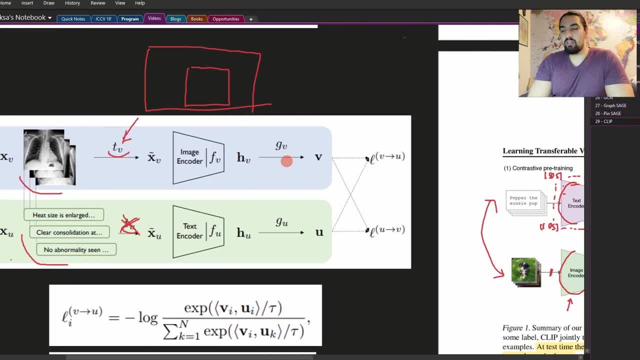 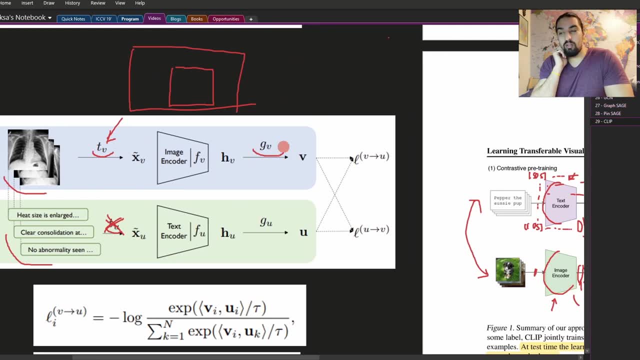 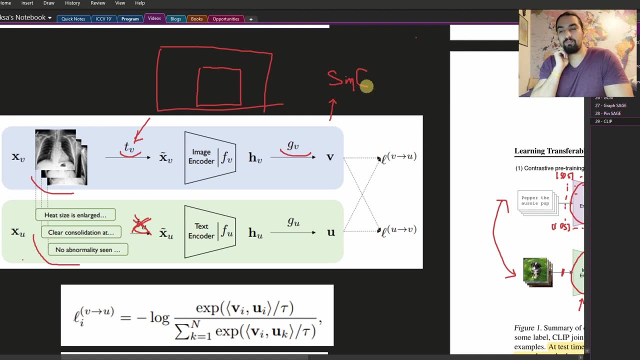 Nothing, So that's everything. Now, the second thing they did is So they modified, as basically, This was MLP in the previous work And also So, by the way, this work, this convert paper, was inspired by SimClear framework. 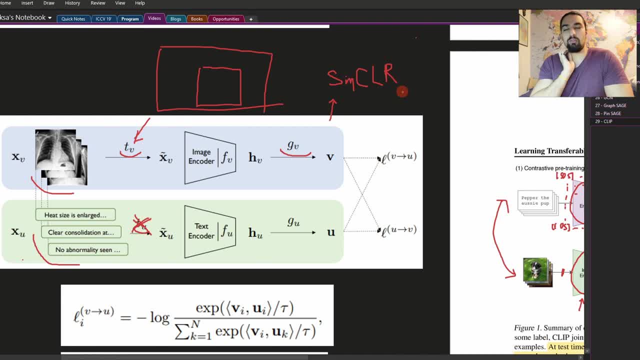 which you probably heard of, which achieved really nice results on self-supervision, visual representation learning, And it introduced this concept of using MLP between the embedding space and between the contrastive embedding space. So in this paper they just ditched this away. 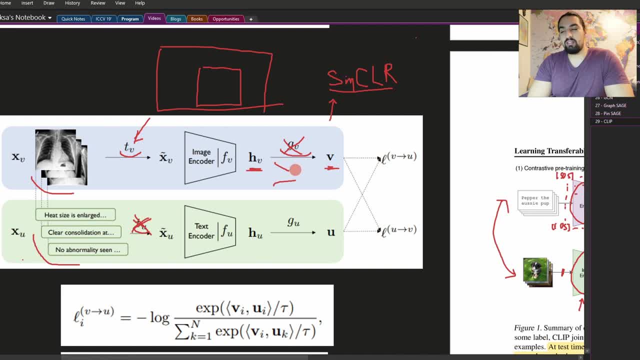 and they just used a linear projection layer and that's it. So no activation functions. You just have one matrix here that projects from the embedding space into the contrastive embedding space. So that's one of the other modifications they did to the pipeline. 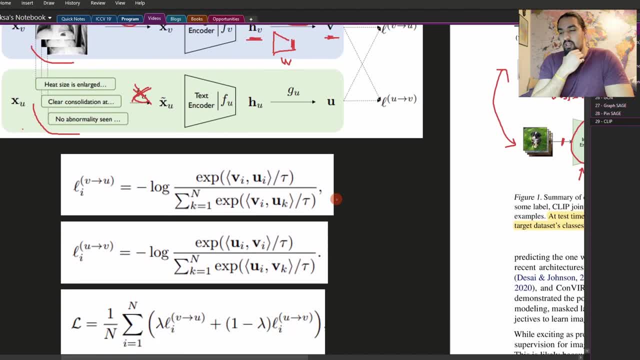 Okay, So once we have that, let's see, like some formulas for the things I already intuitively explained, how it functions. So what we do is the cosine similarity. So this thing, these like angle brackets, just symbolize the cosine similarity. 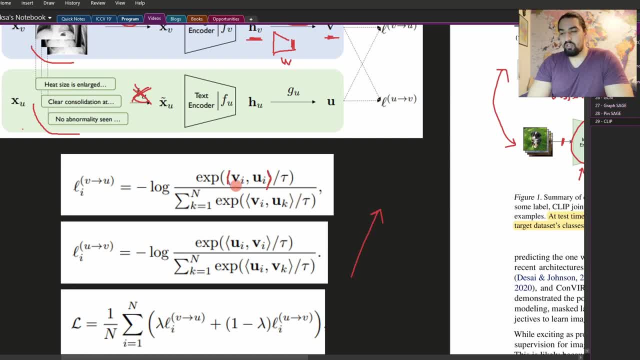 So once again you have two vectors. Let's say this is vi and this thing here is ui. And because this is a cosine similarity, that means these two vectors are normalized. They are basically unit norm. So the norm is: 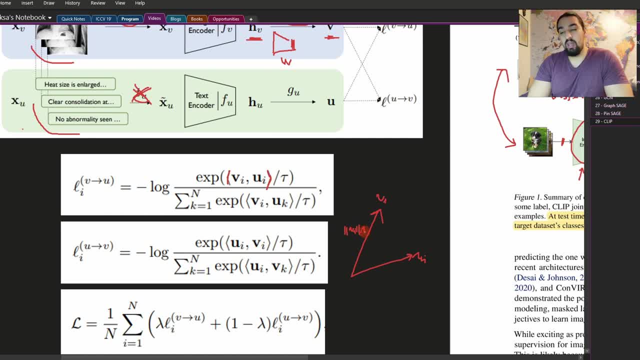 The norm is equal to 1.. And so, basically, when you do the dot product, you end up having cosine of t, So cosine of t of theta, where theta is the angle between those two. So again, if the theta is 0,. 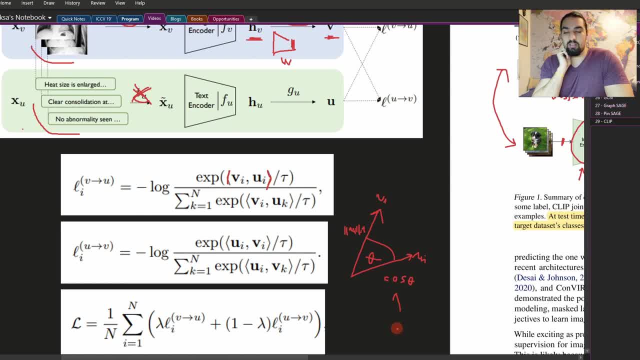 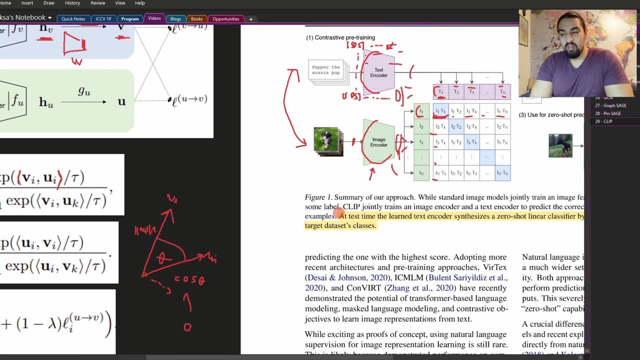 we'll have cosine similarity 1.. If the theta is 0, that means they are orthogonal, etc. So when we say we want to make these two be equal to 1, that means those vectors are pretty much aligned, And that's the idea. 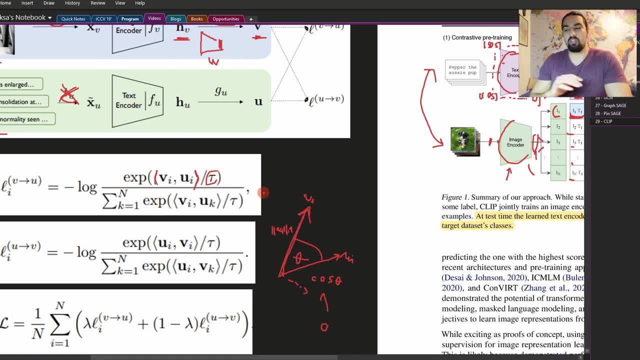 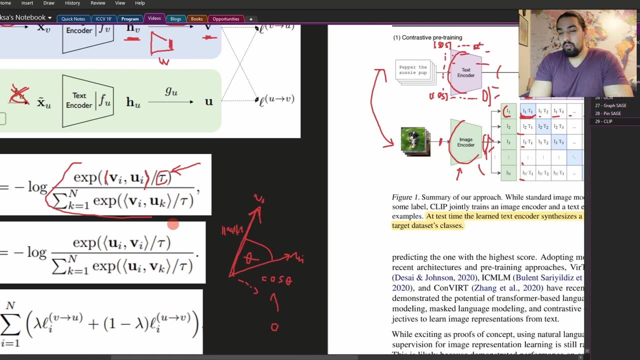 So t here is the temperature coefficient. It just modifies the softmax distribution to make it a bit more steep And it's actually a trainable parameter in this paper and not a hyperparam, And this is a familiar softmax thing. So basically what you're doing. 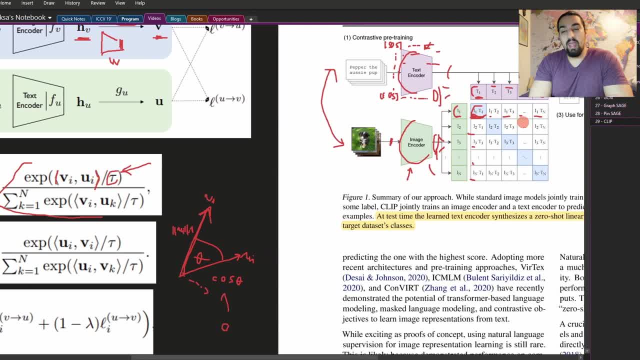 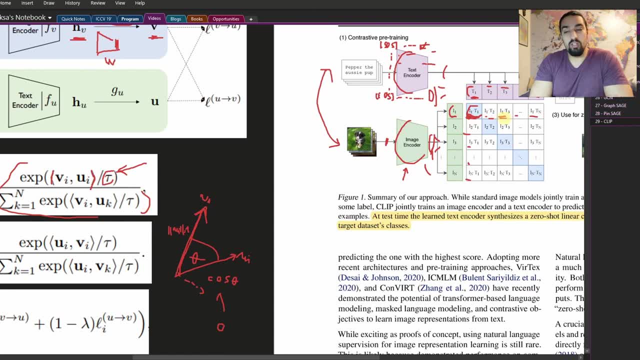 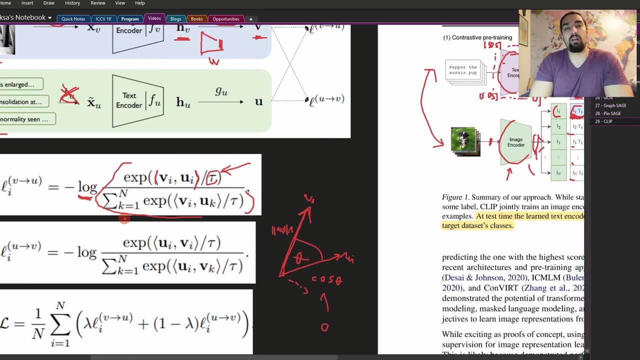 you're summing. So you take this cosine similarity and you just average. So in the denominator you just sum up all of these and you get the probability distribution And then you just have a simple cross-entropy loss over that softmax distribution. 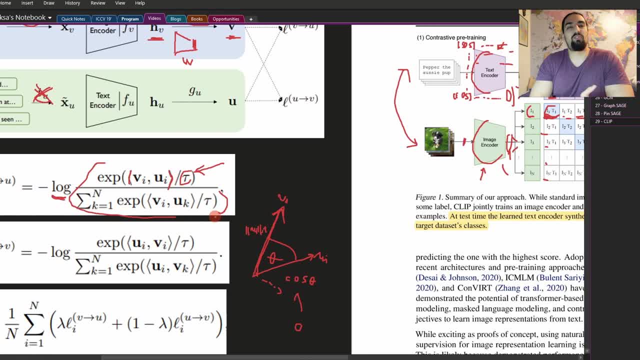 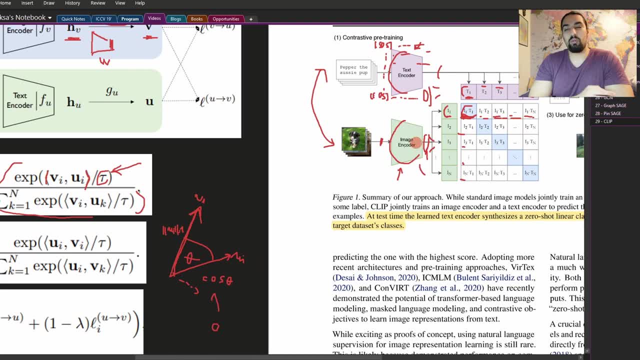 which is a pretty usual thing to do. So you can treat this as a classification problem. basically, You're trying to classify which out of these combinations is the true combination. So what's the true class? And because, as I already mentioned, 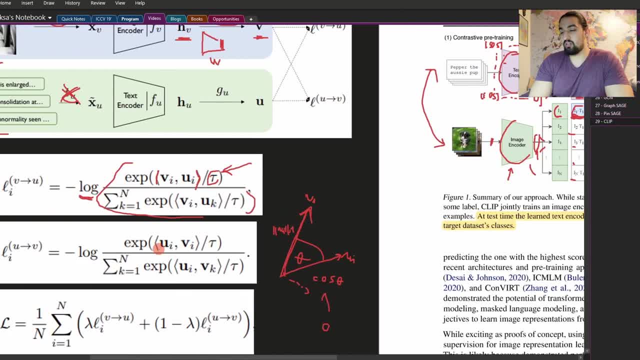 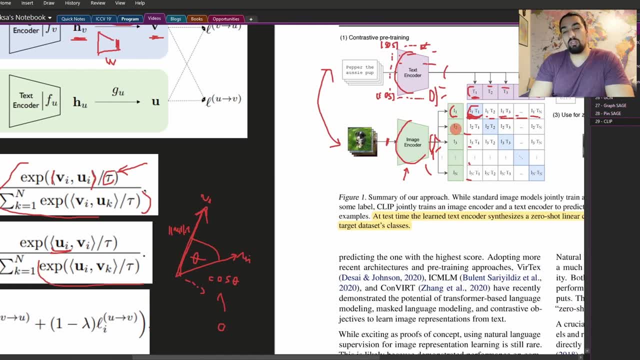 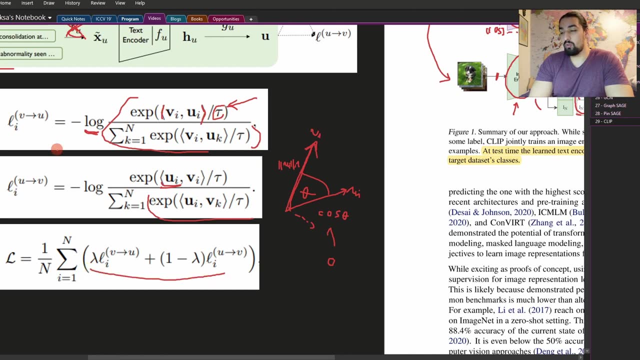 this problem is asymmetrical. you're basically doing the same thing, just this time you put Ui here and your denominator part sums over the column, And the final loss vector is just a weighted combination of those two And you just go over the whole batch. 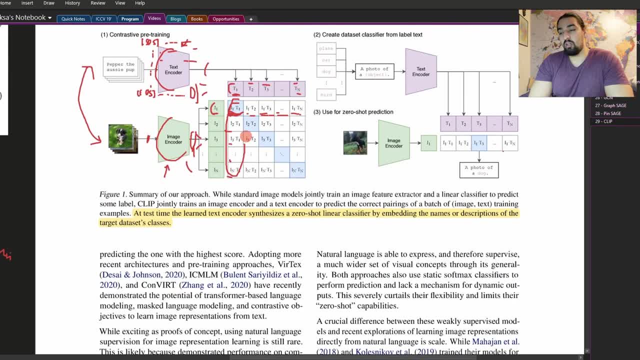 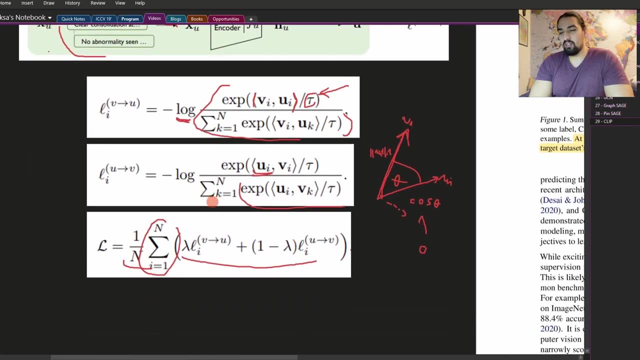 You sum over the batch and you average out. So that means you take these and then you also add this one to the loss and you add the row part And you just do that for the whole batch. So yeah, hopefully that was detailed enough. 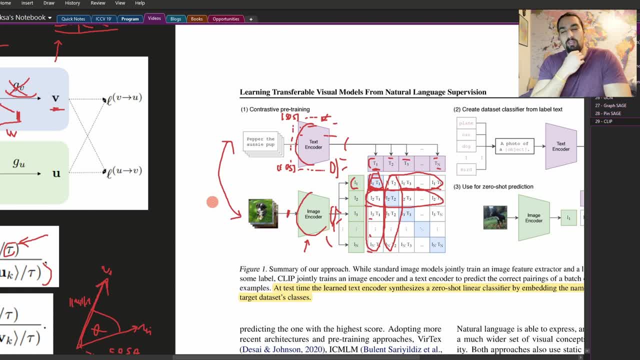 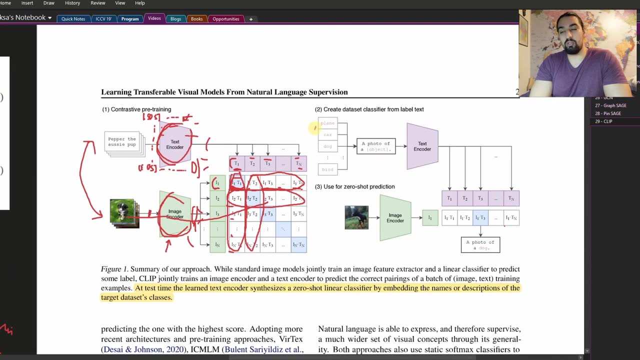 for you to understand the exact way this method works. So once you have that loss, you just backprop the information, the gradients, through your encoders and you train the image and the text encoders and that's it. Your model is ready for this zero-shot learning. 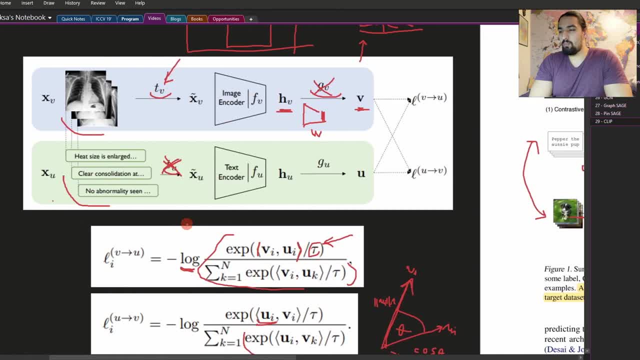 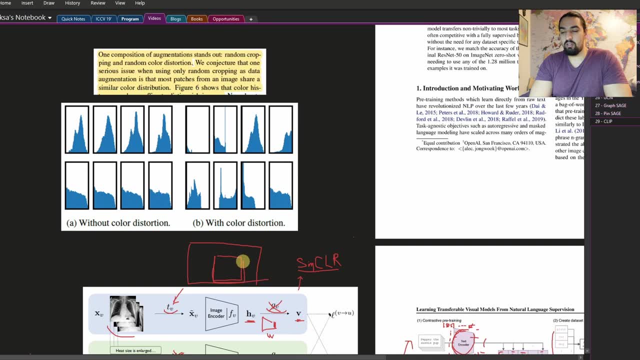 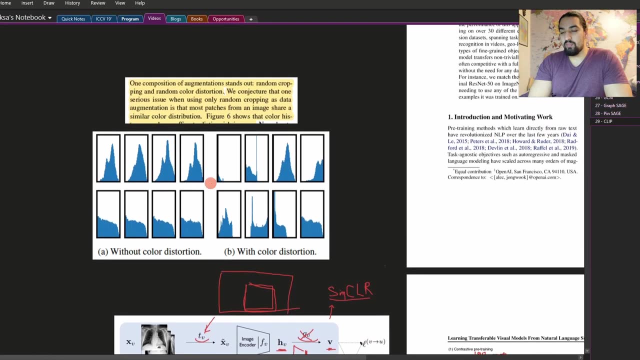 And I'll get to that in a second. And I just want to mention one more thing about data augmentations and the reason they just did this simple geometric augmentation whereby they just cropped from the resized image and not use color jitter. So SimClear this framework I already mentioned. 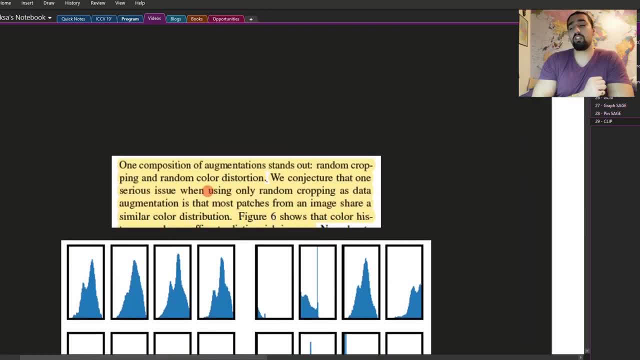 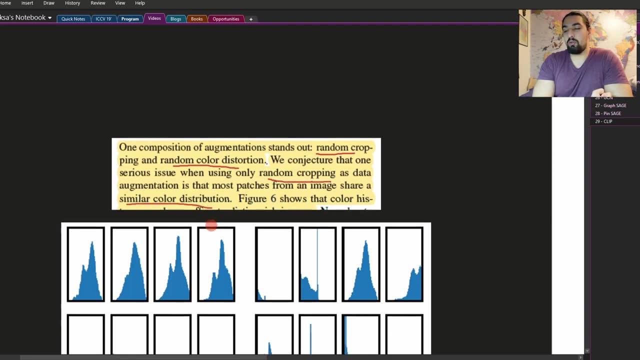 found this nice finding. So one composition of augmentation stands out: Random cropping and random color jitter. We conjecture that one serious issue of using only random cropping as data augmentation is that most patches from an image share a similar color distribution, So that means that the model can learn to cheat. 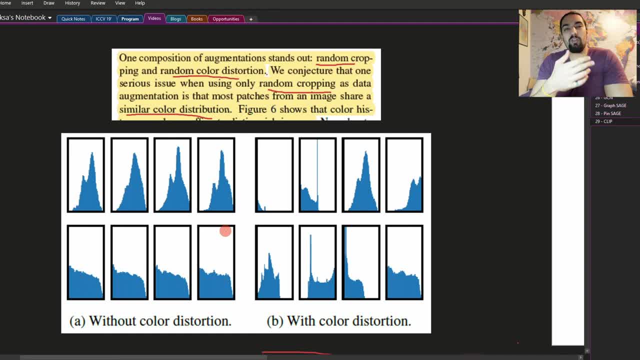 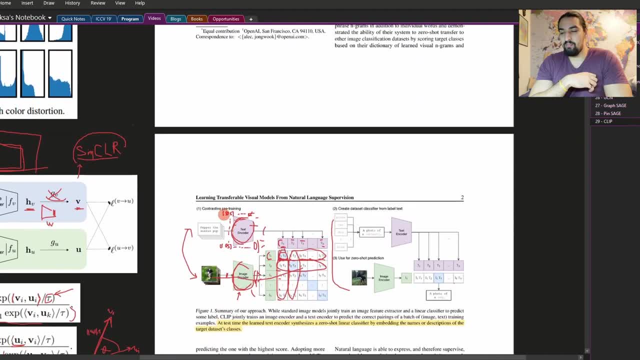 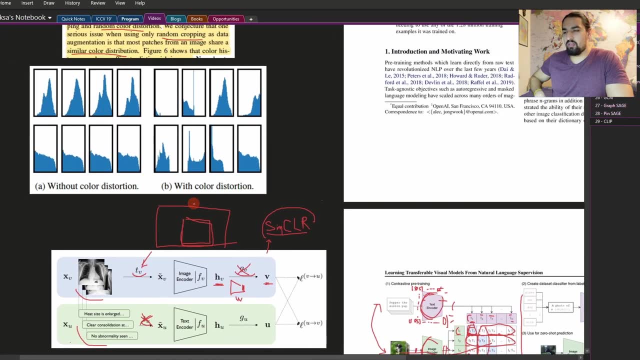 by just looking at the histogram distribution and figure out that those are the same instances. Now the difference between this framework and CLIP model is that they just compared images to images in contrastive loss, whereas we have now text and image. So the reason I think they just did. 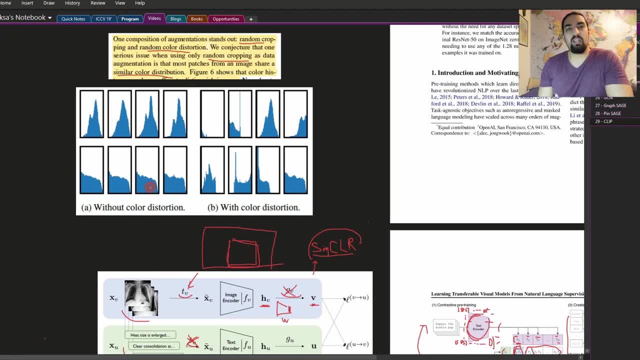 away with color jitter is the efficiency, and we'll see that in a couple of minutes because, yeah, that's open AI. They're just trying to scale things and see how they perform with that scale. So what you can see here is the following: 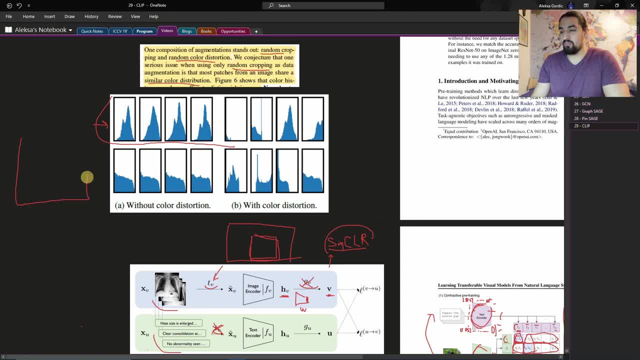 So this thing here is basically you have an image and if you just stitch the color jitter and you just take a crop and you take another patch, and you take another patch, and you take another patch, So all of these patches will have, as you can see here, four different patches. 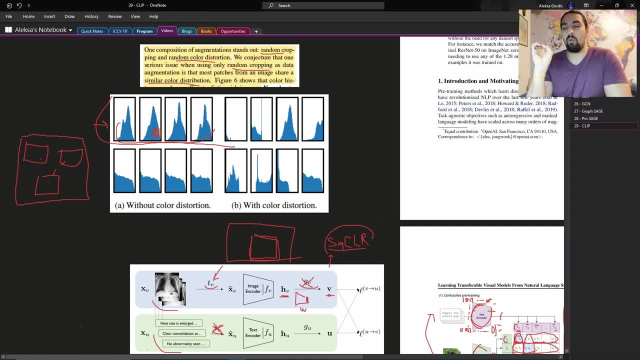 They'll have a similar color distribution and so once you do the contrastive learning between those augmented patches, it will be really easy to even. they are visually different. the histograms are the same, so it will be a really easy problem to just place them in the same part. 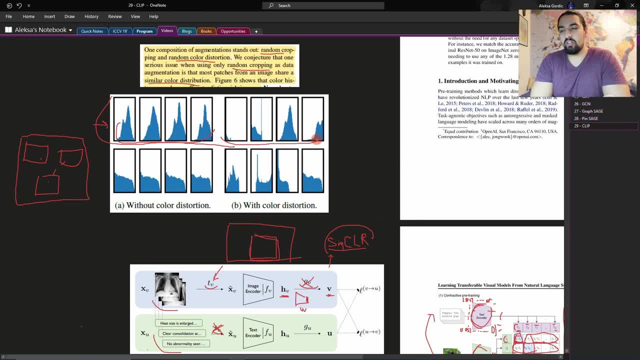 of the embedding space, where here, once you do the color jitter, you can see that the model can exploit, cannot exploit this trick, and that's the reason they use color jitter, But, as I said, probably because of the efficiency reasons. so it was a trade-off. 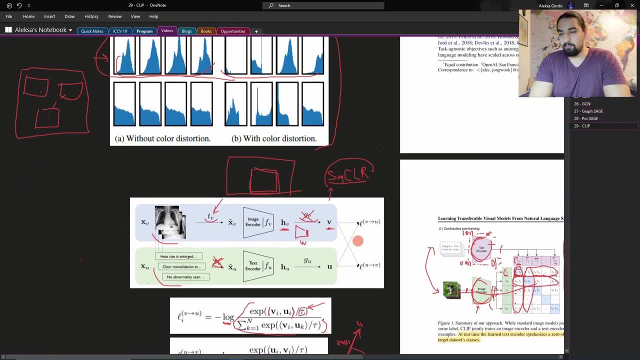 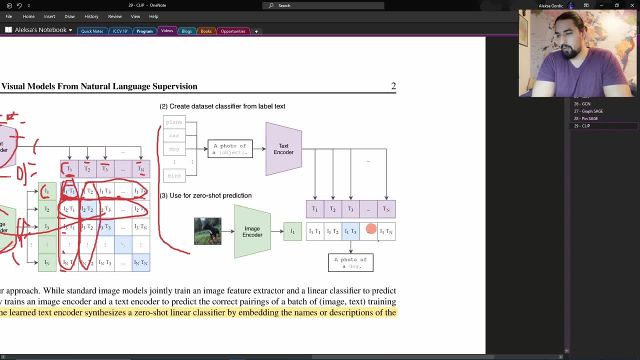 they just used the random cropping. Okay, that was it. Now let's focus on this part- and this is probably arguably the most important part of this paper, and that's: how did they use this thing now? So, after they trained it. 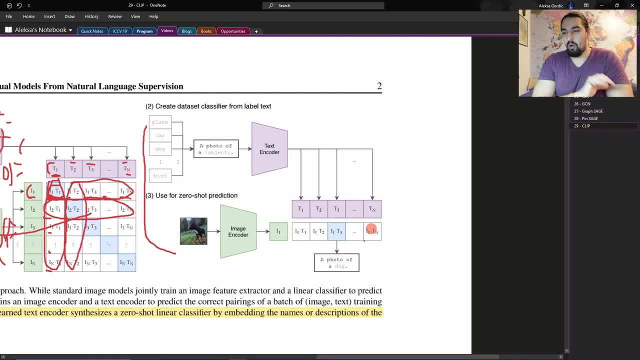 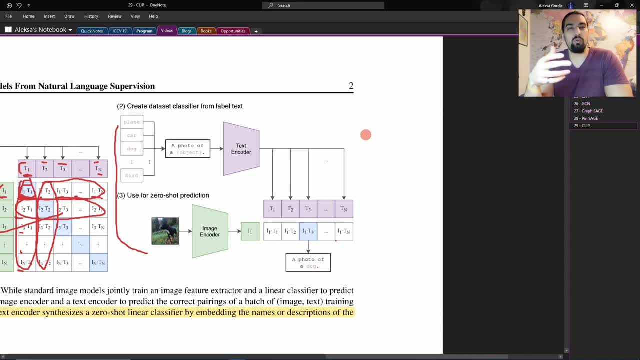 how did they use it in a zero-shot setting And this is how. So basically, let's say you have, you now want to just test this one in a zero-shot setting on a new downstream computer vision task. Let's say we have Cypher 10. 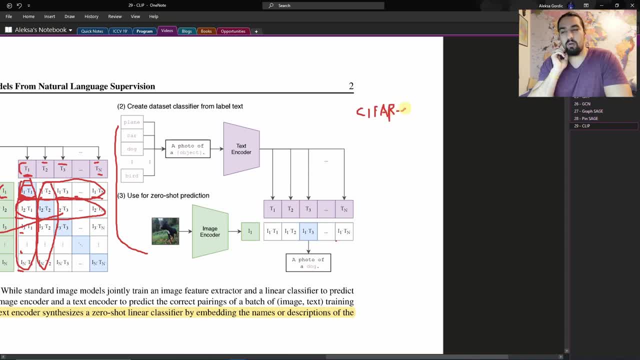 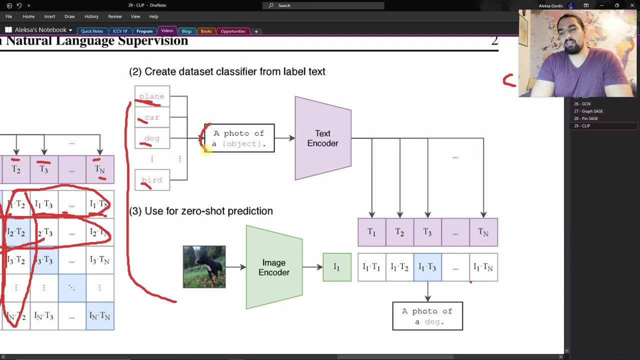 and that's a pretty famous and simple benchmark in computer vision- and you basically have 10 classes right, And so maybe plane, car, dog, bird, etc. So what you do is the following: You basically embed those classes in sentences of this construction maybe: 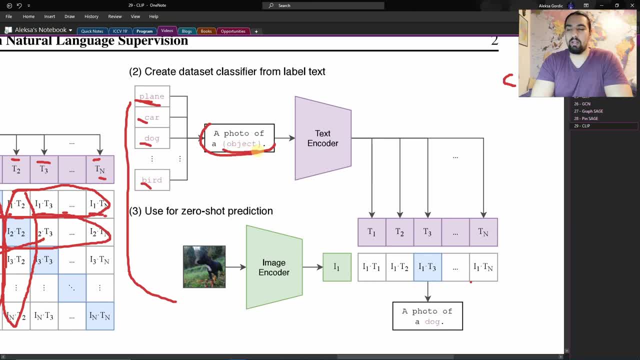 A photo of a, and then you just fill in the blank. You put a plane, your car, dog, whatever So, and once you do that, you just encode those sentences in the same way, so you have end of sentence token. 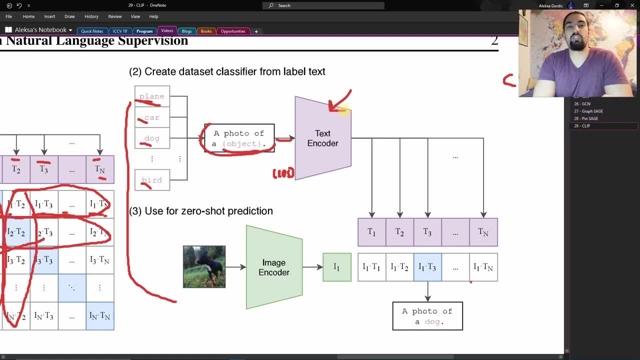 blah blah. this is transformer, but this time this one is trained, so we have it initialized with certain weights after the training, after this contrastive learning training, and so we just prepare all of those embeddings, So we just pre-compute them once. 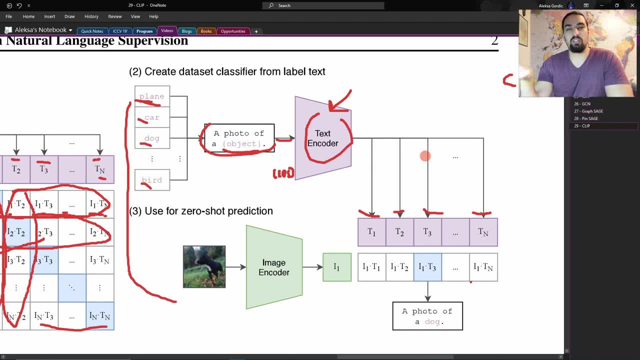 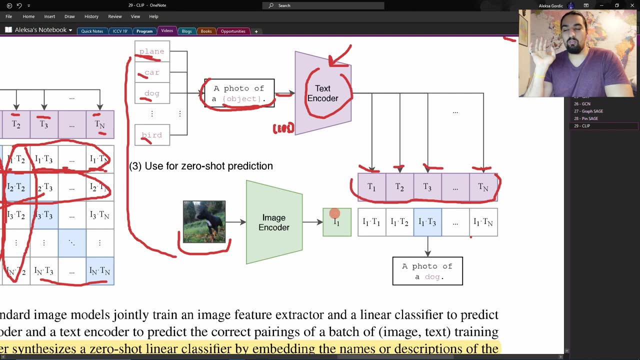 and that's it. We are finished with text encoder. We just have this batch of embeddings here and now. how we do the zero-shot classification is the following: We just take the image that we want to get classified, We find its embedding vector and we just do a simple cosine: similarity. 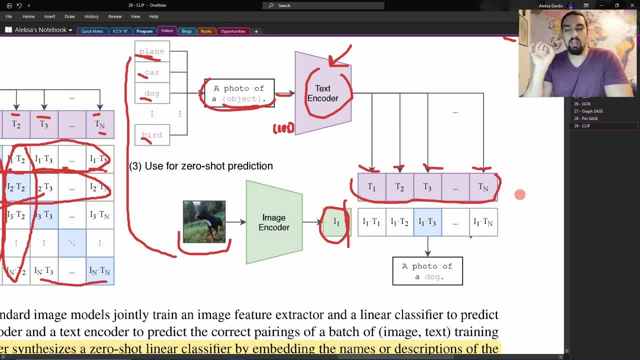 between this embedding vector and between these embeddings here. So we're just embedding textual embedding vectors and whatever the highest similarity is. that's our class and you can see here a photo of a dog. and because T3 corresponds to that particular sentence and it had the highest similarity, 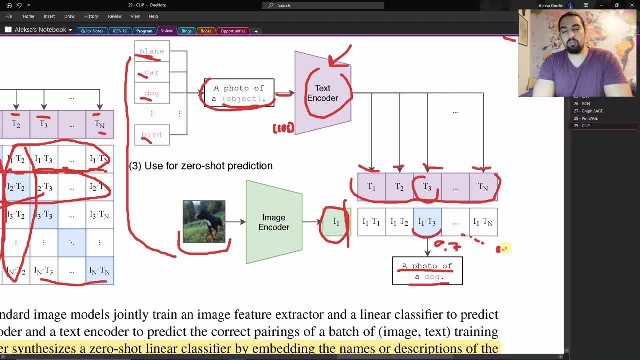 so maybe this one has 0.7 and all of the others had, maybe, I don't know- 0.1.. This one had even smaller similarity, etc. So that's how the method works in a nutshell and, yeah, hopefully this was clear enough. 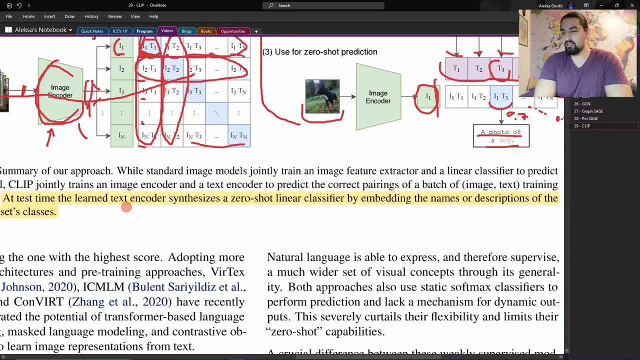 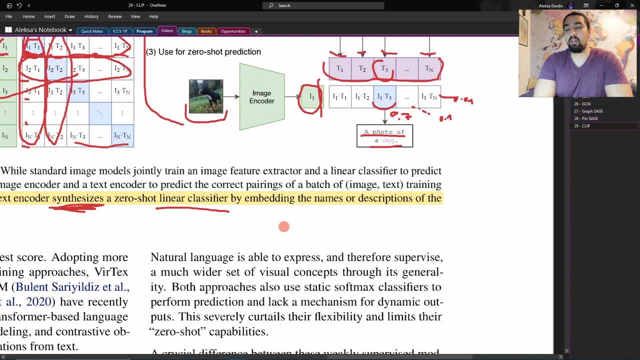 And they also mentioned it here At test time. the learned text encoder synthesizes our zero-shot linear classifier. So synthesizes- that's an interesting word because you can basically treat this as a hyper-network, So you can basically treat this whole system. 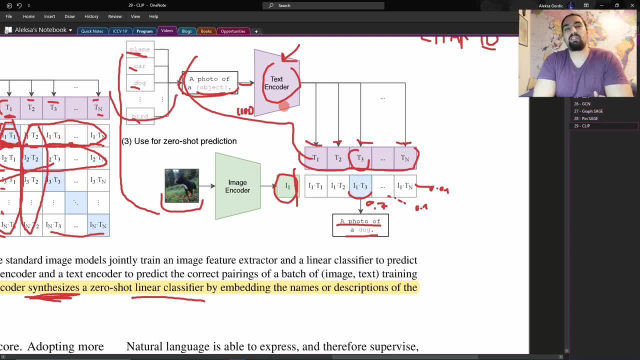 with text encoder and with these sentences as an adaptable, as a hyper-network. So basically, depending on your data set, you construct certain corpus of sentences and those will adapt this text encoder so that it's like a configurable linear classifier, in a way. 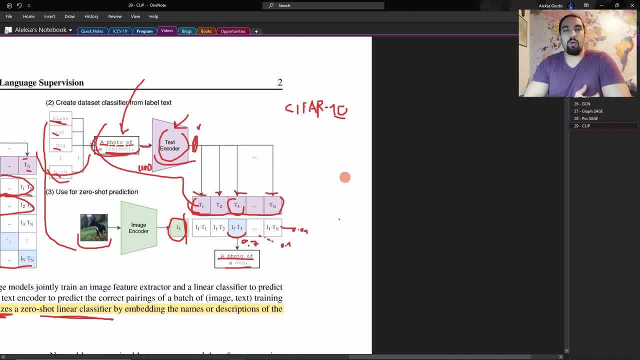 Let's call it that way. So if you're still having problems understanding why this is a linear configurable classifier in a way, let's look at it from a different perspective. So, as I mentioned, we have those linear projection layers from the embedding space of the encoders. 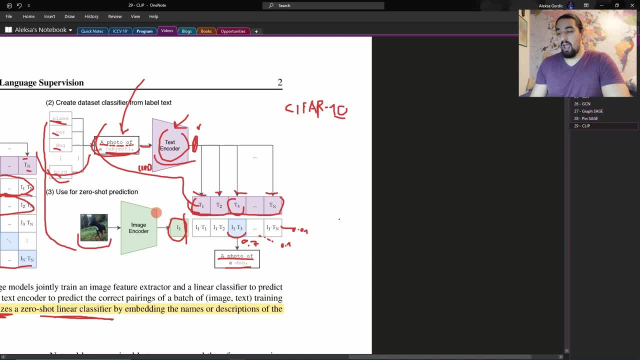 into the contrastive embedding space. So that means after the embedding space here we'll have a linear projection which will project this vector into this vector so that we'll end up having same dimensions across these image vectors and these text vectors. So that means this one is d dimensions. 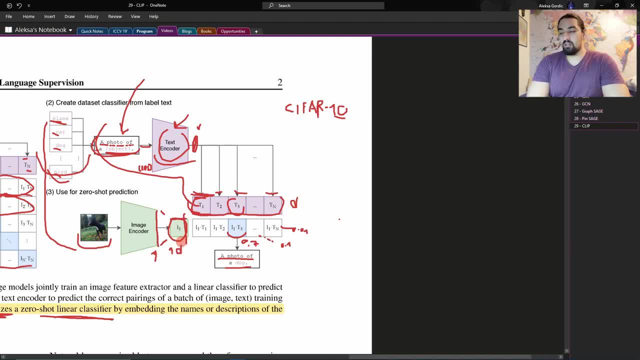 and all of these have d dimensions. So let me take a look, let me just extract this box and represent it as a vector, which it is, And these are also d vectors. So when we do, when we do, cosine similarity, when we do dot product, 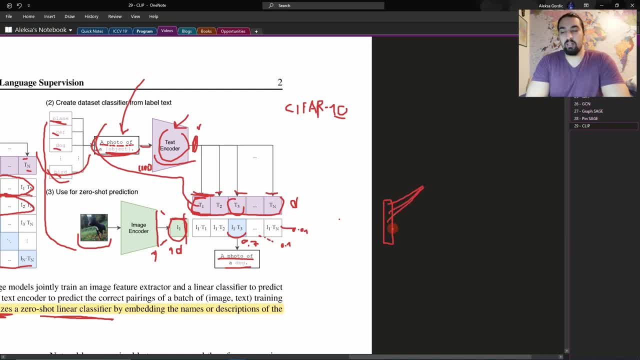 we're basically doing, in a way, we're creating a fully connected layer. So these weights here, these weights correspond to maybe t1. And we'll end up with a value here, And we do the same thing with t2.. t2 is also a fully connected layer. 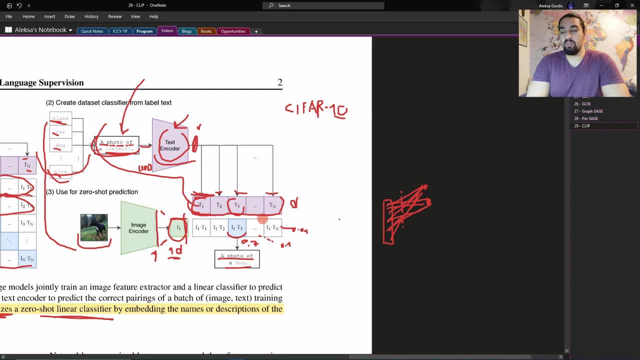 over this vector here And we end up with a second value, And we do that n times, So we'll have n values here, So that's like n heads And you can see that all of these weights here are basically configured depending on the text corpus. 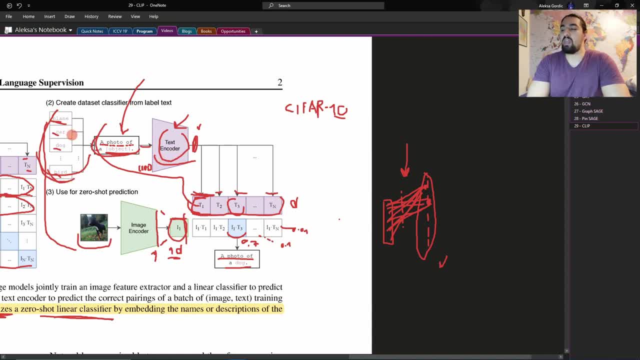 because text encoder is pre-trained and it's fixed And we just input these, this text corpus that's created out of the labels for that particular data set, And we end up with particular weights here which, again, are basically specifying the weights in this classifier. 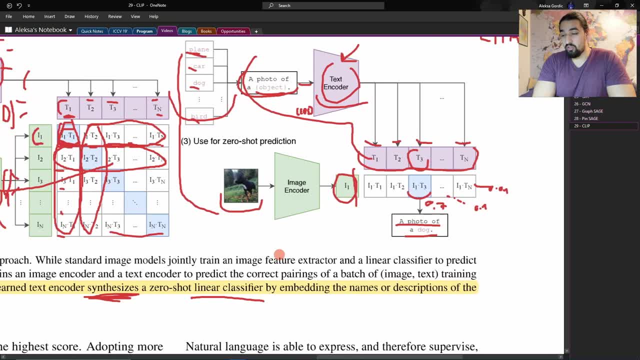 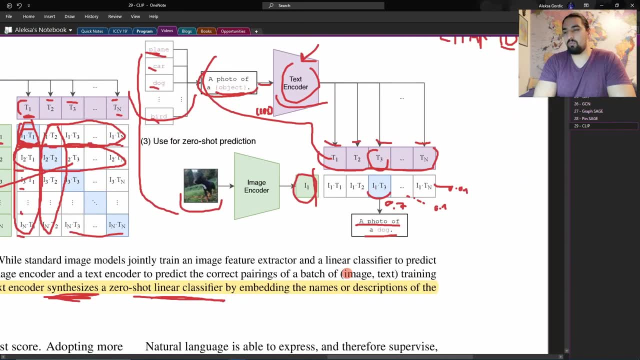 And that's why it's a configurable classifier, And so that's really interesting. So a zero-shot linear classifier by embedding the names or descriptions of target data set classes, And we already saw that, So we just embed it. So one detail I omitted here. 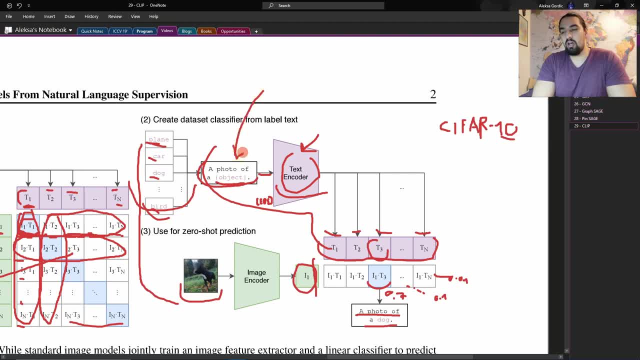 is that basically what I do here is assembling and prompt programming. So if you're familiar with the GPT family of models, you know that prompt programming is a thing It's called like a software 3.0. And the idea is depending on how you construct. 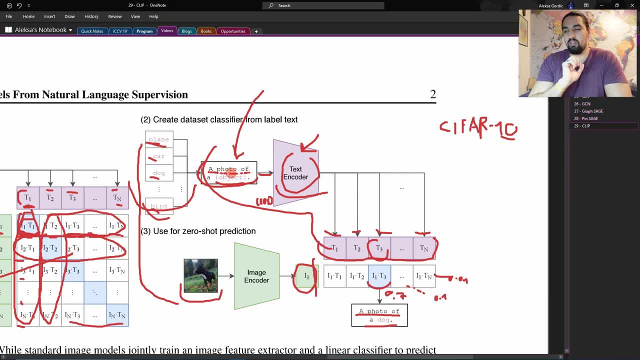 these the skeleton around the class. you'll get different performance out of your model. So what they ended up doing is they played with different constructions and they also assembled a bunch of these constructions, and they just average out these the features here, before they project them. 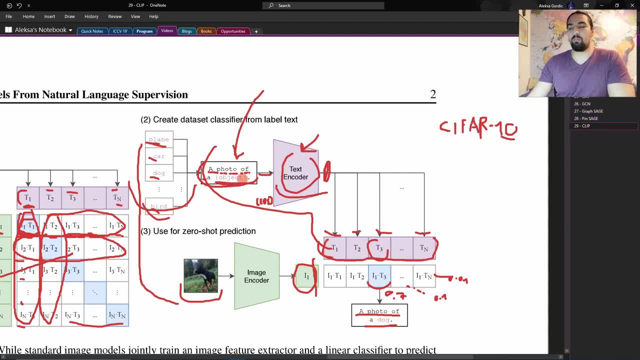 into the contrasting embedding space. So what that means, maybe you'll, they'll have so for car. they maybe have a photo of a car, but they'll have another sentence, like a nice photo of a car, for example, And they'll just take both of those embeddings. 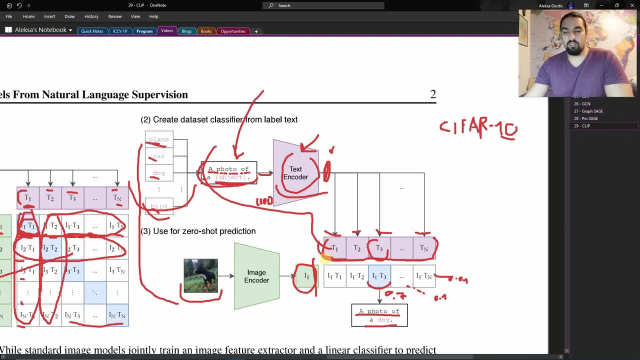 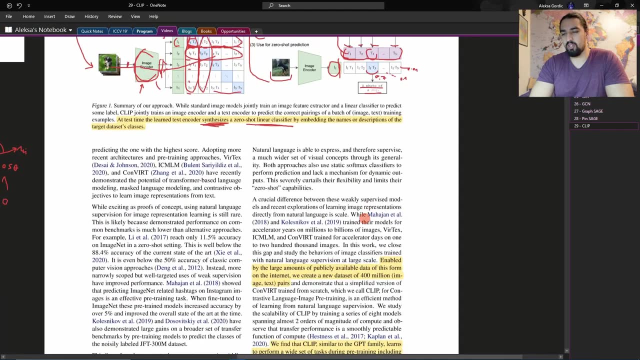 and they'll average it out before they project it into contrasting space, And they found that that small trick actually improves performance significantly. But we'll get to that in a bit more detail a bit later. Okay, So that was that was. that was a good explanation. 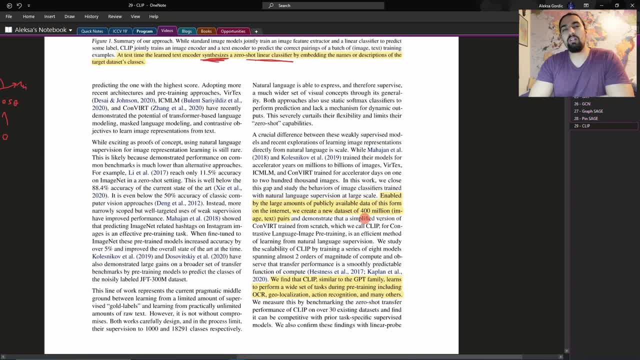 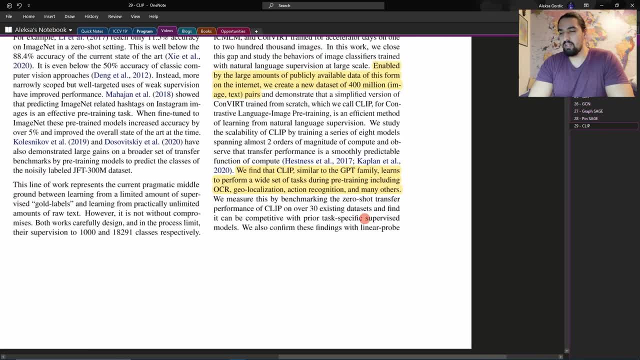 And now let's, let's dug even a bit deeper, and then we'll we'll jump to experiments. So let's see. As I said, we find the clip similar to the GPT. family learns to perform a wide set of tasks during pre-training. 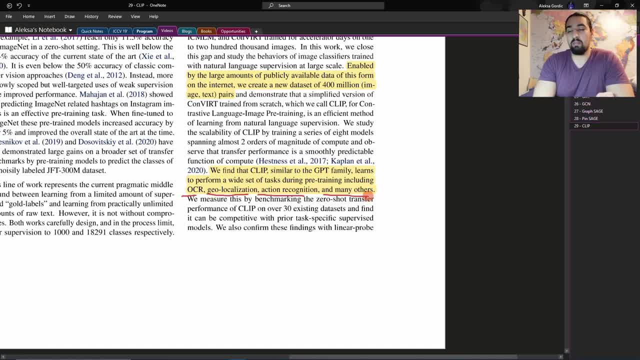 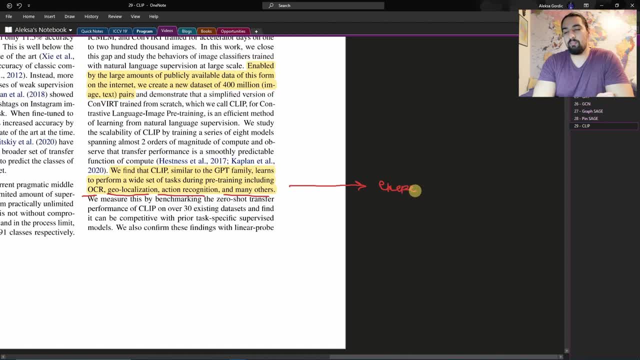 including OCR, geolocalization, action recognition and many others. So, again, if you're familiar with GPT family of models, you know that there is this emerging- let's call it- phenomena happening. So where you're basically training your model, 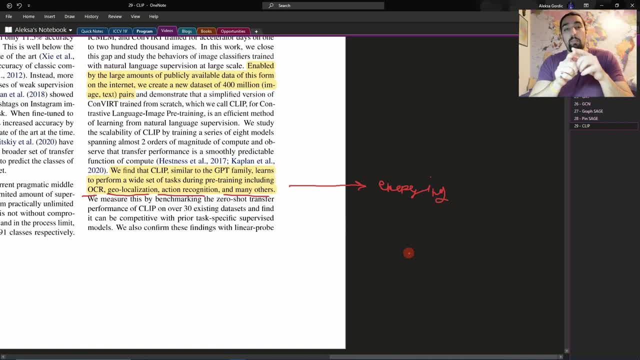 on some tasks, like GPT-3 was just trained to predict the next token And once you do that, they figured out that it learned how to do many other tasks that it wasn't explicitly trained to do. Like maybe you input a sentence into GPT. 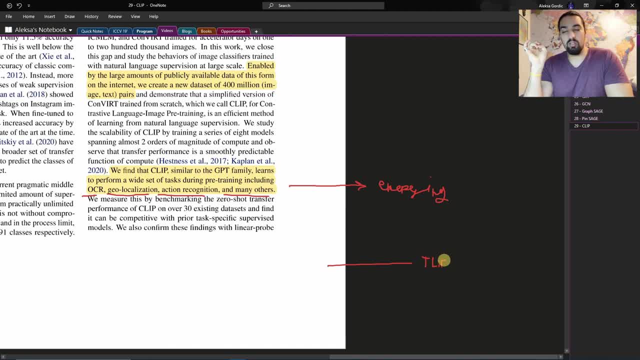 and you just append too long, didn't read words here, And then, after you sample out of it, you'll notice that it actually learned to summarize this input sentence, even though it wasn't trained to do that, And the same thing happened here with clip. 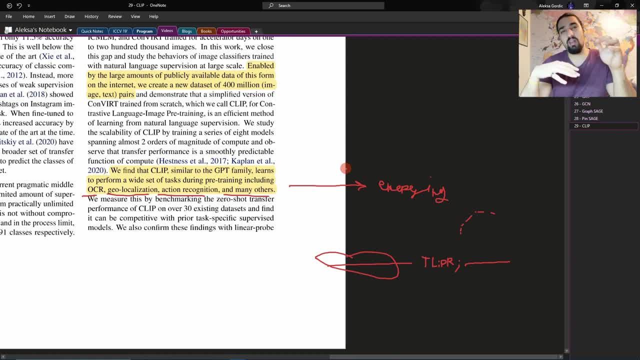 They trained it to, as we saw, to just associate the most probable text sequence with the image, And along the way it learned to do all of these things. So that's interesting. Okay, I'll get to this pic in a second. 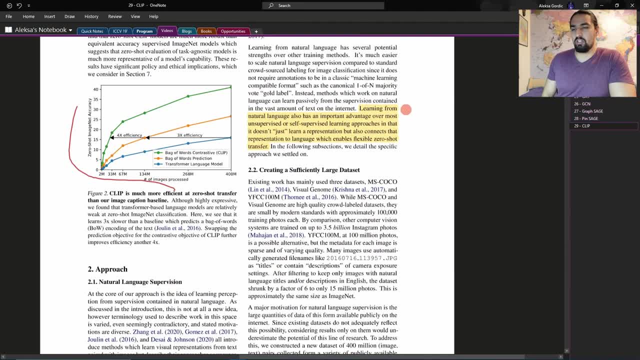 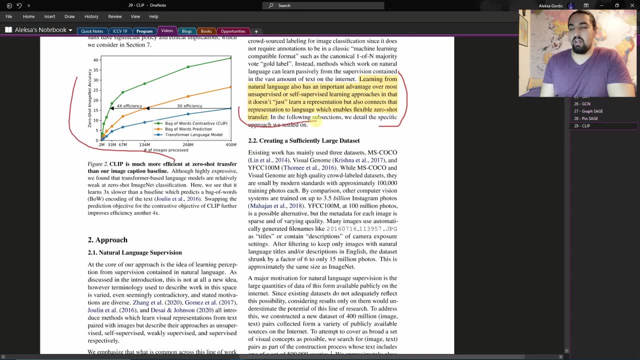 Let's just go over a couple more things. So learning from natural language also has an important advantage over most unsupervised blah, blah, blah. So basically this says that the way how we train it enabled us to do this flexible, zero-shot transfer. 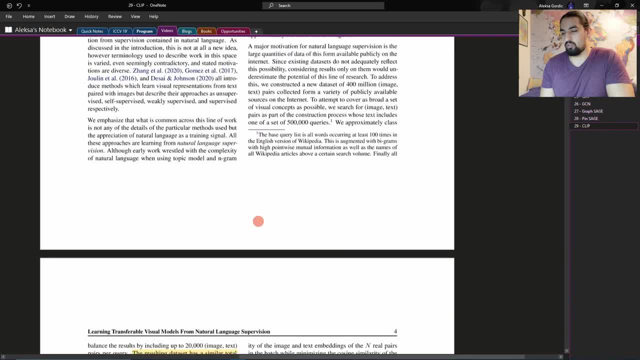 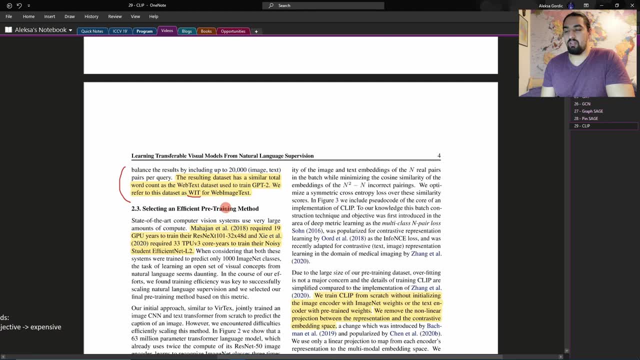 as you saw with the hyper-nap work story. I just explained to you- And yeah, I mentioned that they created this WIT dataset, which has 400 million pairs of images and text. So why they did it Is because they wanna leverage the scale. 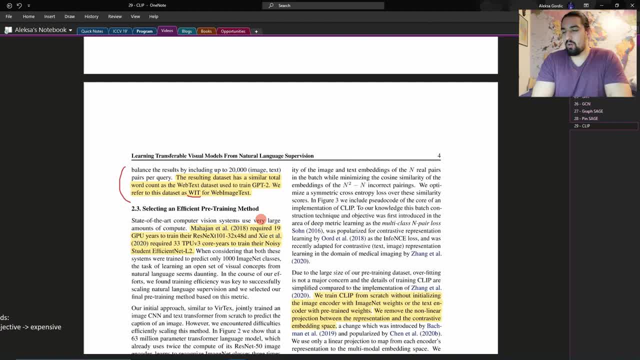 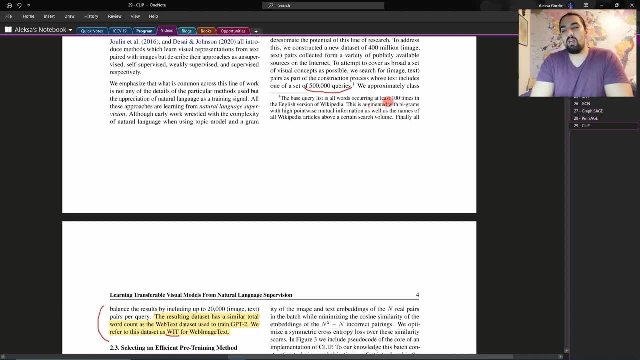 And none of the existing datasets had that. So that's why they did it, And it's interesting how they created it. So they had like a half a million queries, which they created like by collecting words that appear at least 100 times in English version of Wikipedia. 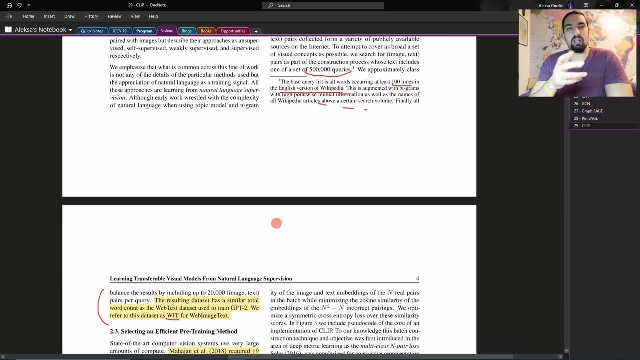 and some other heuristics, And they tried to balance it out so that every one of those queries has, like a similar number of images associated with them. That's how they created the dataset. But, more importantly, let's jump into this part about efficiency. 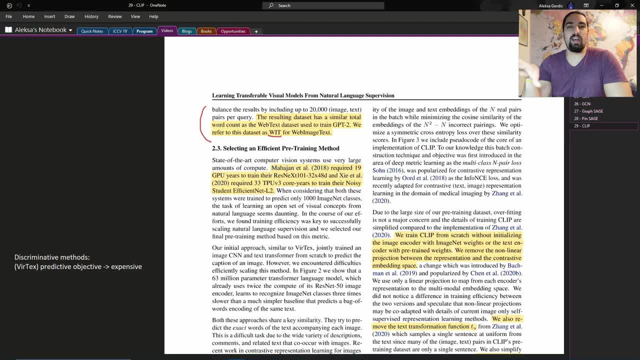 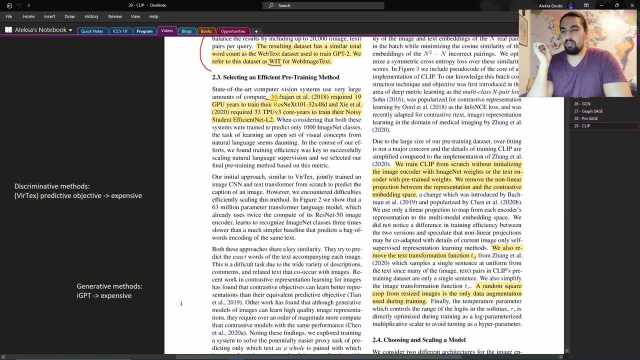 So let's see why they ended up having the exact same task that I just explained. So they say here that Mahajan and his collaborators- folks from Facebook- required 19 GPU years to train this ResNext model Xi, and others required 33 TPUv3 core years. 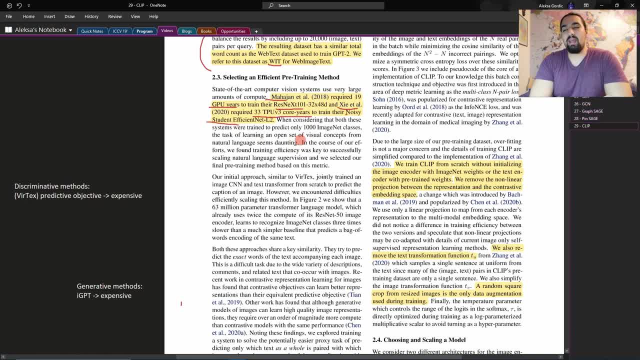 to train the noisy student. So that's a lot of compute And the only thing they're trying to do is predict 100 ImageNet classes And compare that like comparing that to the to learning the open set of visual concepts from natural language seems daunting. 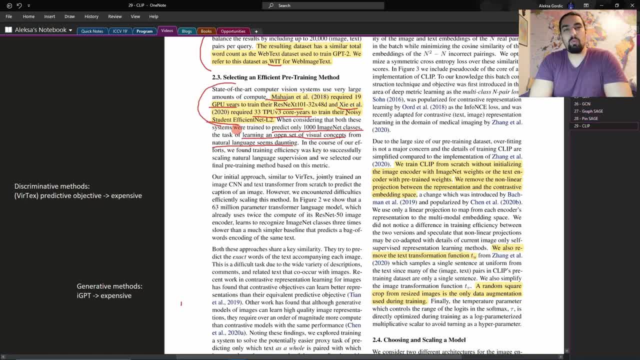 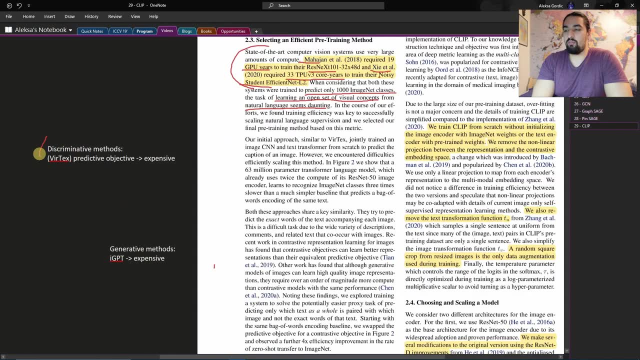 So if this was so hard to do, then just imagine how much harder it is to train the model of predicting, like just natural language labels that they're open for. They did try first exploring with this discriminating method that has a predictive objective instead of the contrastive objective. 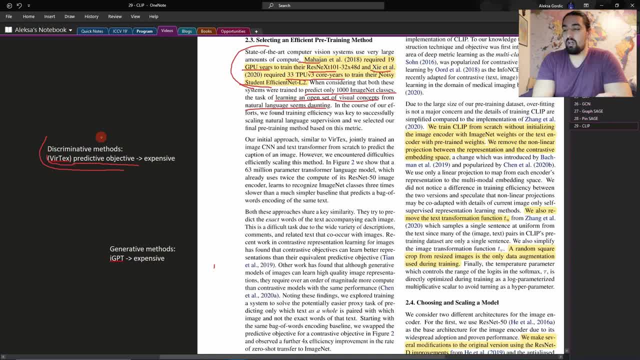 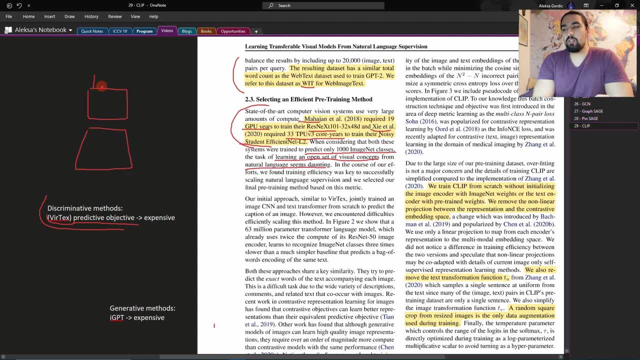 I just showed you. And what Vertex paper did is they basically also had an image encoder and they had a transformer above it. They were trying to predict the exact same words from the caption of that image. So you have an image, you have a caption associated with it. 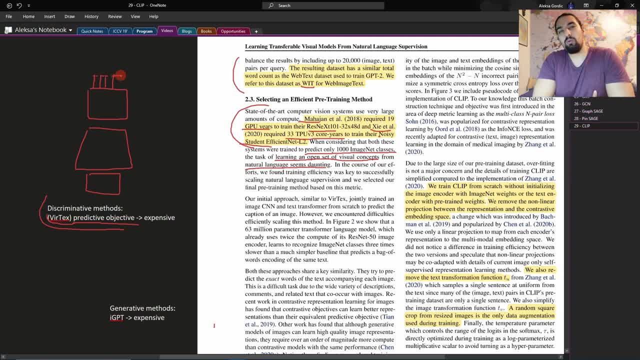 and you're trying to predict the exact same word. So that's not the new approach. like, we've been doing these captioning predictions for a long time And people noticed that the visual representations you get out of these tasks. so when you, for example, 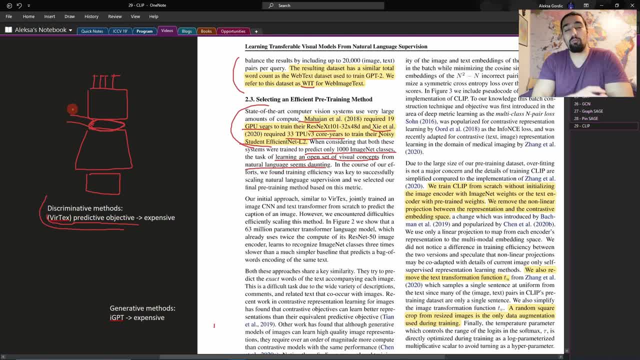 do some linear probing on these representations that they're really useful for many downstream tasks: classification, et cetera. So the thing is they tried this one and it was too expensive, And we'll see one of the charts above which will nicely explain this. 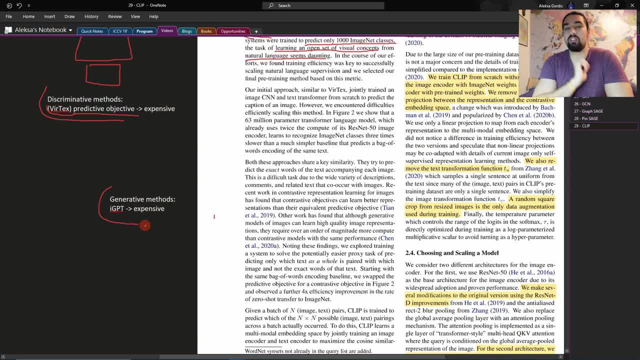 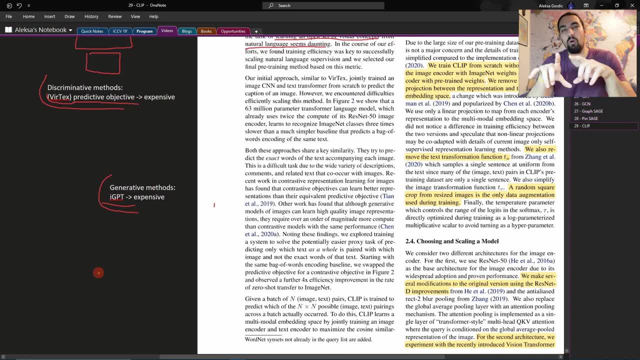 And the second thing: they also considered these generative methods like image GPT And what it does: it learns to autoregressively, just regress the image, the input image, And it also learns really nice visual representations. But the thing is, 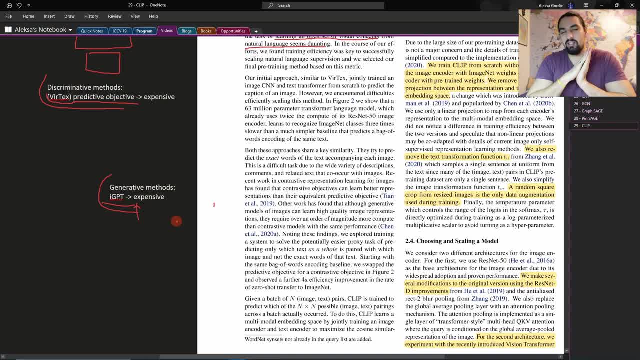 it's not efficient, And efficiency is the key point here. This is OpenAI. They want to make the most efficient method and then leverage the compute they have, both in the Harvard Sense and the huge data set they collected. So, like the Bitter Lessons by Sutton, 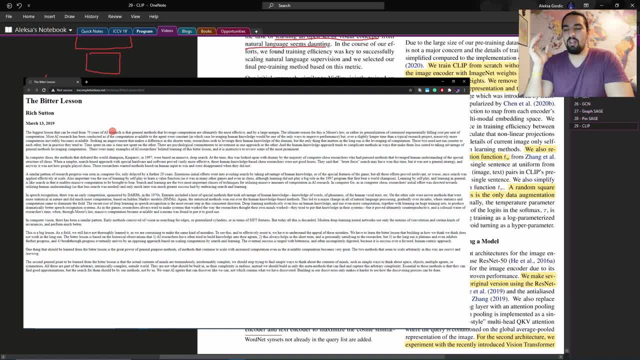 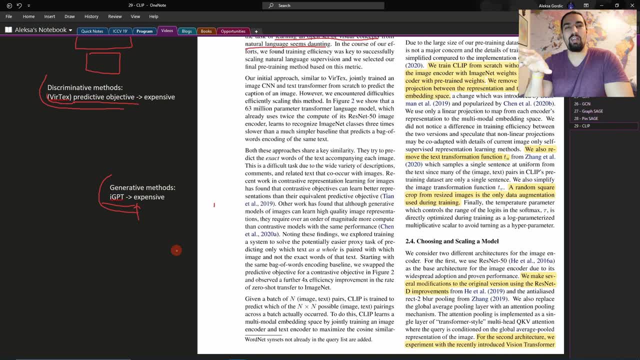 are a nice read if you're not familiar with this. But basically, the more compute you can throw at the problem, usually that's a good idea. I'm not saying that's the only way we'll go forward with the research, but that's definitely an option. 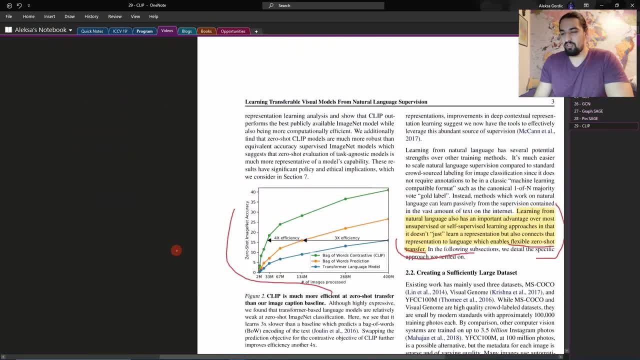 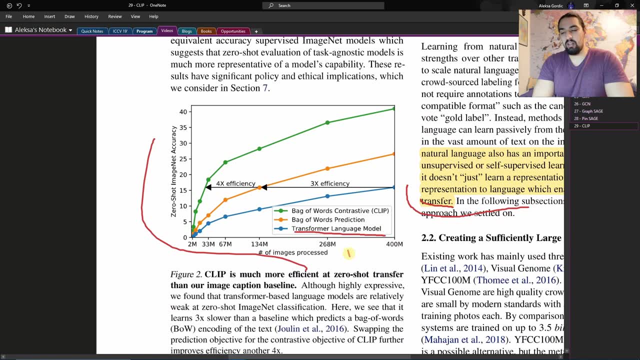 Okay, Having said that, let's just jump to this chart, And what it did is. what it did is the following: So this transformer language model, that's basically that vertex approach I just mentioned. So you just basically stick the transformer on top of the image encoder. 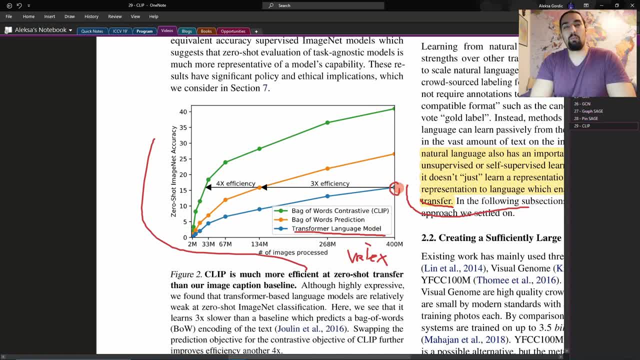 and you can see that by trying to predict the exact same words from the caption, the zero-shot image- net accuracy is really low and you need a lot of data to accomplish it. Compare that to just a simple baseline, where, instead of trying to predict the exact same words, 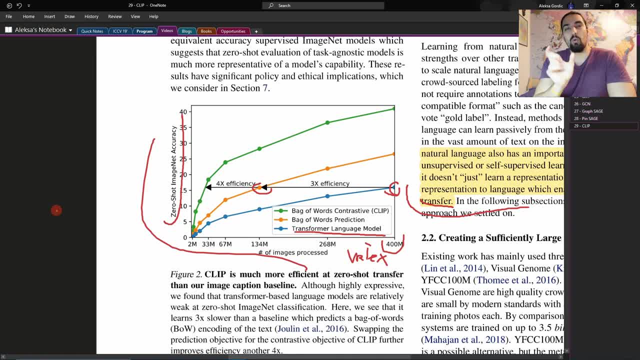 from the transformer. you're just trying to predict which words appear in your caption. So that's a much simpler problem. So you have like a vocab here, like maybe 30k of words, and you're just trying to predict which words are present. 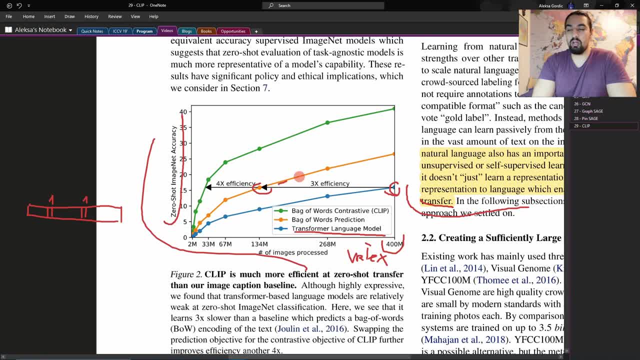 in your current caption And that's this orange line. you can see, And we already noticed that we have a 3x efficiency gain. And finally, once we ditch that, once we ditch the predictive objective altogether, so trying to predict the words, 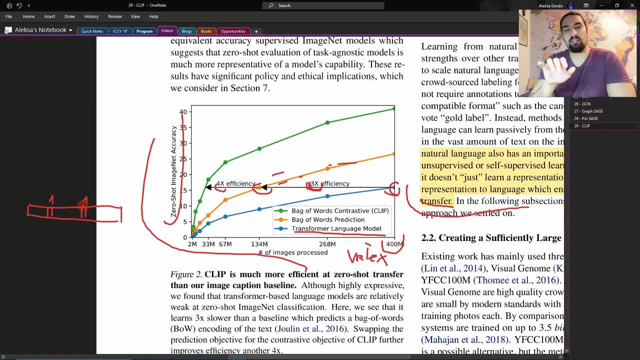 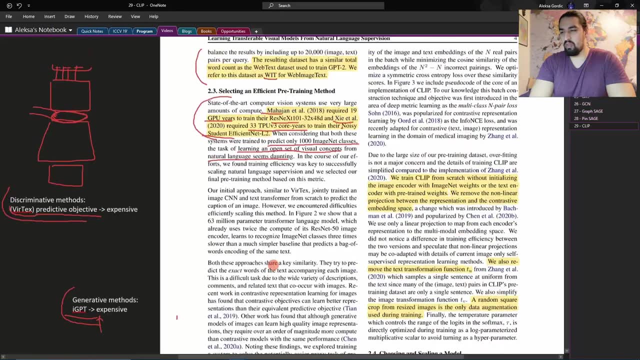 and just trying to associate the textual sequence with the image, we get a boost in efficiency, a further boost, and now we can truly leverage the computation. Okay, So that was it. That was it about the efficiency part, And now I'll go into some more details. 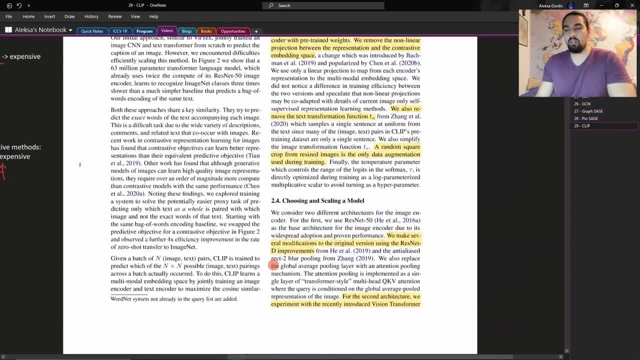 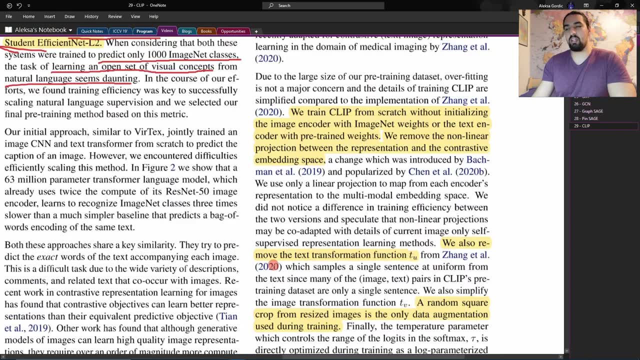 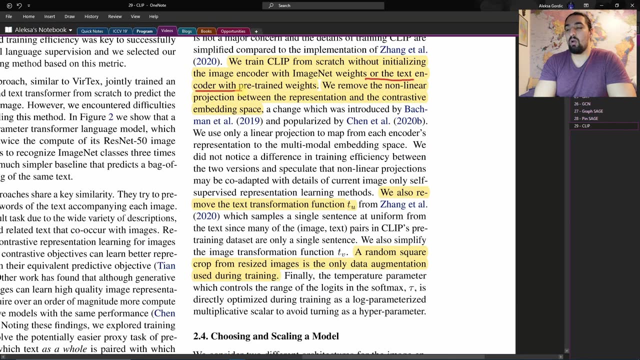 about the method, and then we'll just jump to exploring the zero-shot results they got. So they say here that we train Clip from scratch without initializing the image encoder with image net weights or text encoder with pre-trained weights. And why they do that is because work like Vision Transformer. 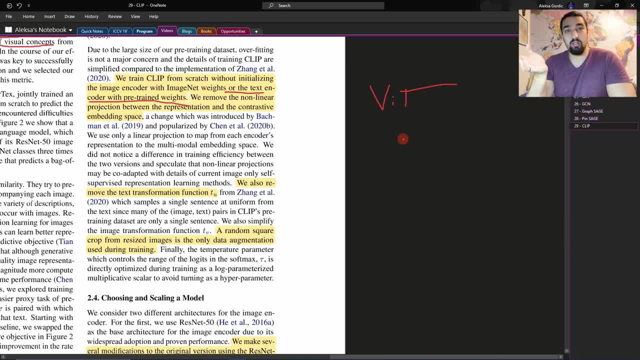 already showed that once you have enough compute and enough data, you really don't need to bias your model in any way. So what Vision Transformer showed is that this particular model is better than CNN's, given enough data, like they use JFT 300 dataset. 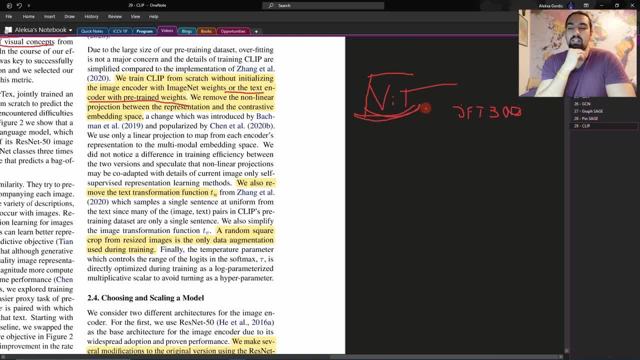 and that's Google's proprietary dataset, and they show that it outperforms CNN's and it learns something similar to CNN's just a bit better, obviously. So that's why they don't encode it, why they don't initialize it with pre-trained weights. 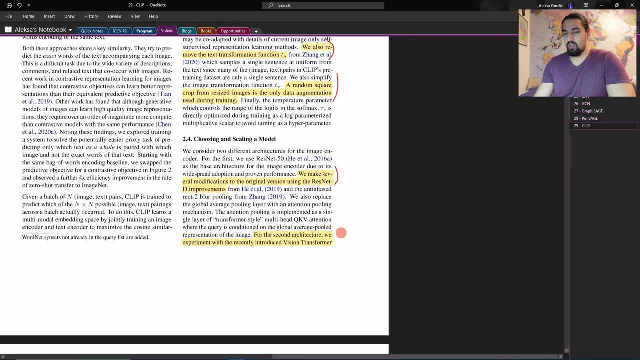 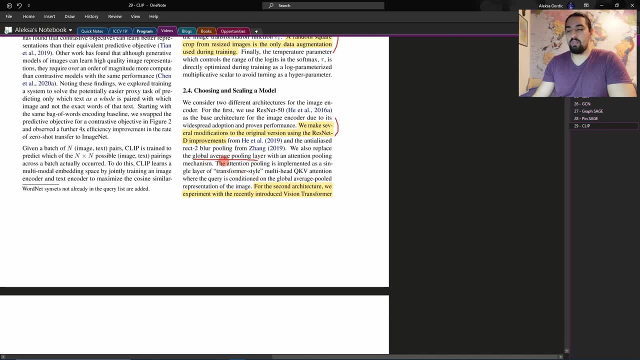 So I explained most of these, so I'll just skip them. Yeah, this is an interesting detail. They are not using so for ResNet. they just swapped this average pulling layer with the attention pulling layer that's implemented in a Transformer style. 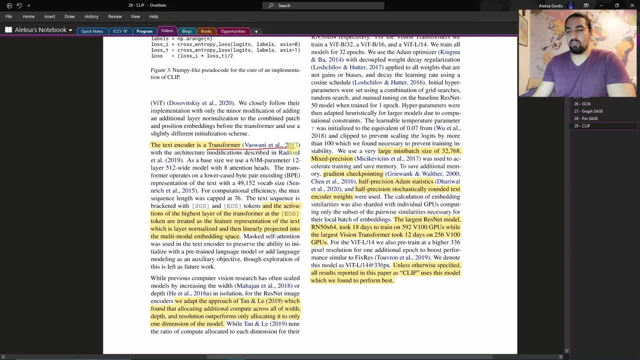 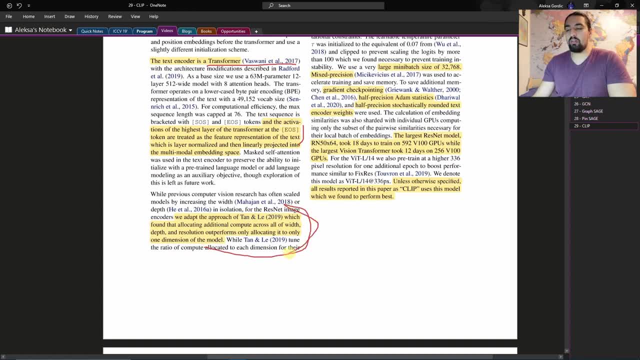 And yeah, they're using- as I said was funny for the text- encoder, and I also mentioned this one about EOS. So the interesting part about how they scaled their approach is that they used EfficientNet's ideas, So they used ideas from this paper. 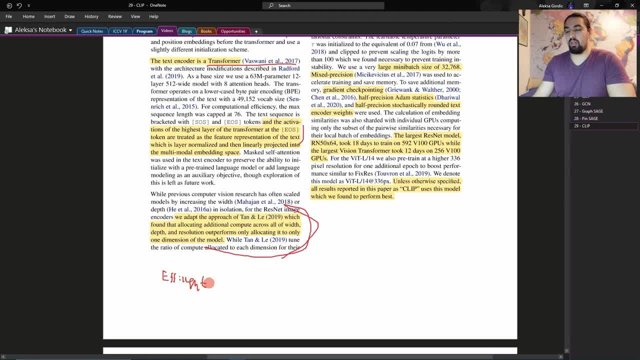 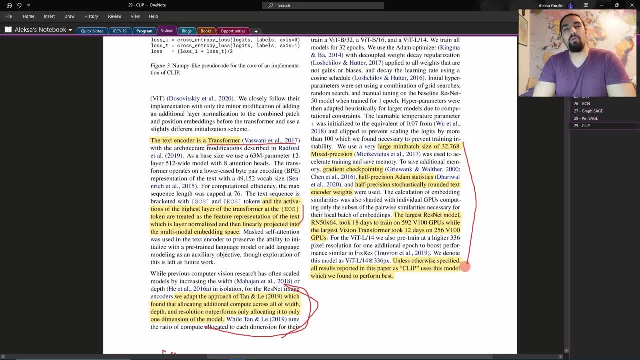 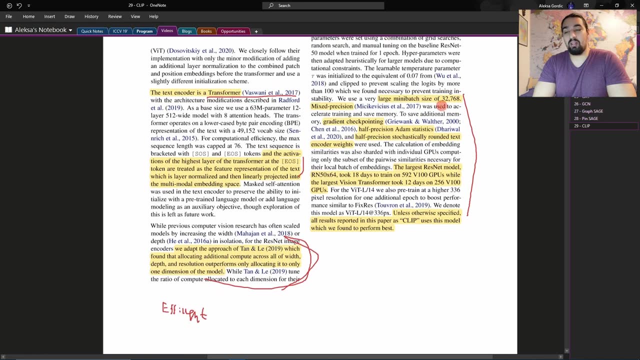 to scale. I don't know how to write today. okay, to scale their technique, And I just highlighted these just to show you how much engineering goes into all of their research work And, like you can see, all of this mixed precision. 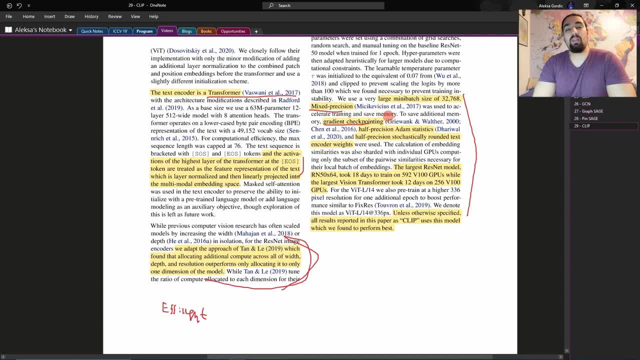 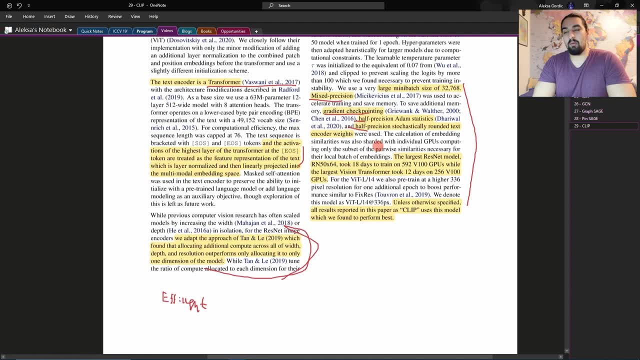 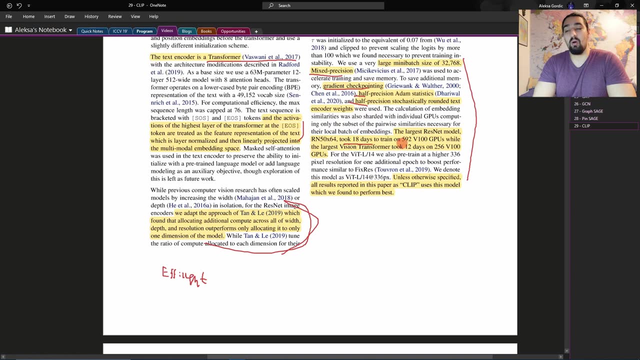 gradient checkpointing is all about making use as efficiently as possible of the memory available on their hardware. So half precision, half precision. And yeah, it still takes a lot of time to train their biggest models. So it took 18 days to train. 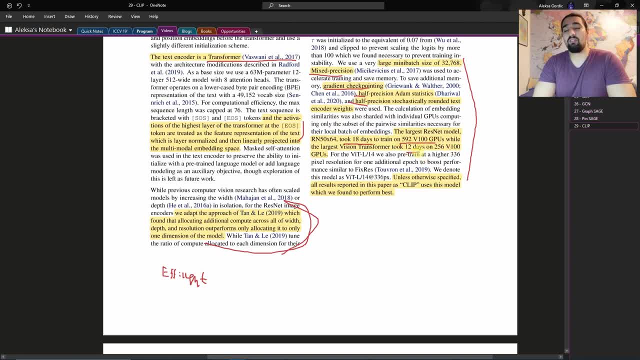 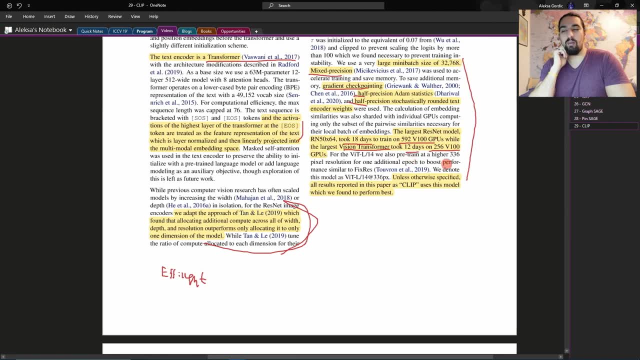 on almost 600 Wii, 100 GPUs and 12 days on 256 for the Vision Transformer, which is. Vision Transformer is more efficient than CNN's, and that's one of the points that that paper made, And that's why it takes a lot less. 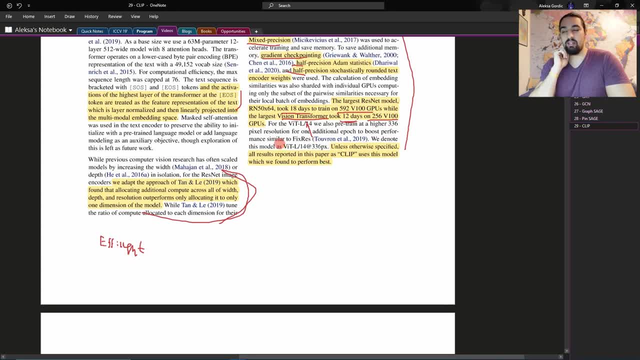 time to compute. And finally, the best model they had is the Vision Transformer L that was trained for one epoch on a higher resolution of 336 pixels, And that's the final Clip model that they are using throughout this paper. Okay, finally, experiments. 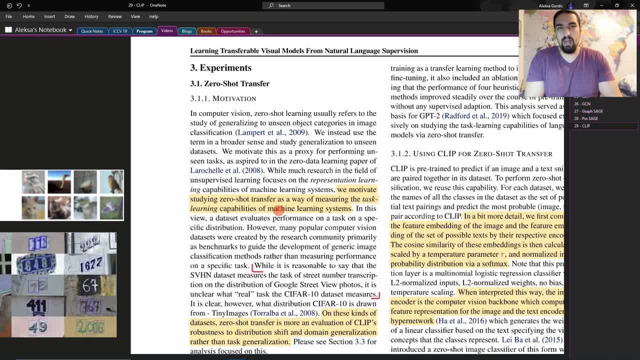 So, as I mentioned, the target, the goal of this paper is to show that Clip has a really nice zero-shot transfer performance, And what they mean by zero-shot transfer performance is a bit more general than what they usually mean by saying that in computer vision. 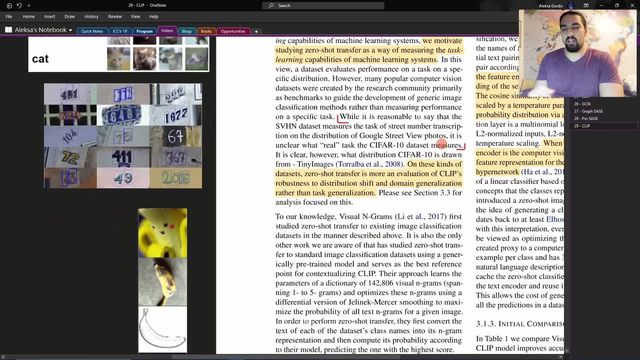 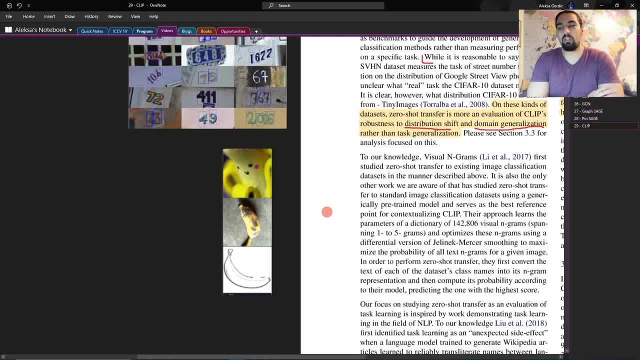 So usually- and it's here, they say it here- most of these tests are testing for distribution, shift and domain generalization. So what that means is that previous models in computer vision. basically, you want to test if it's having a really good performance. 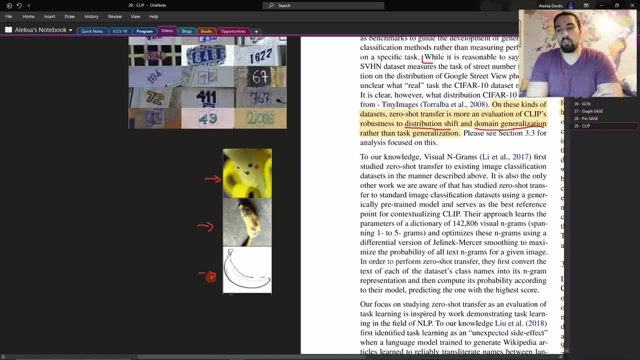 even when you change the underlying distribution. So basically, here you have a banana like a real-world banana, like a sketch, and those are called different domains. And the other thing that we're testing for is that, for example, if the model was testing, 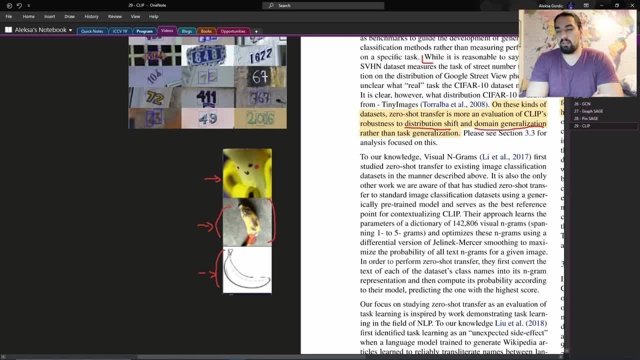 was trained on real-world objects like banana, I don't know- dogs, cats, whatever- and you want to see how easy it is to just do some fine-tuning or do some linear probe on top of the feature space to maybe learn also about new object. 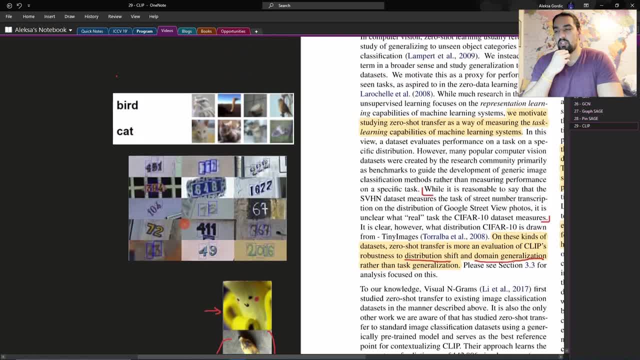 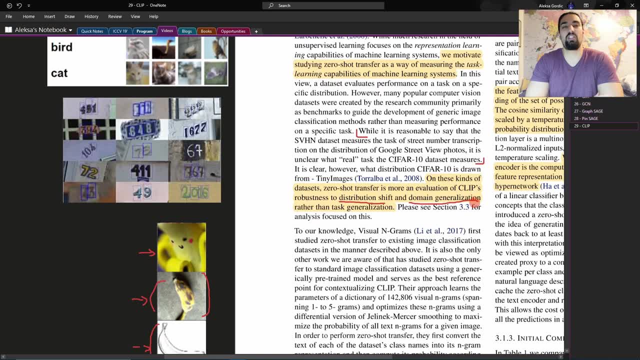 like maybe horse, And what they mean by zero-shot transfer learning in this paper is not generalizing to those, so distribution shifts and domain generalizations, but to new tasks. So for example, they say it here- well, it is reasonable to say: 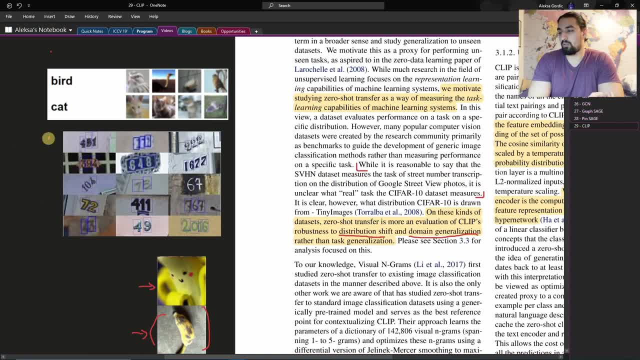 that the SVHN dataset, which is this one, measures the task of street number transcription on the distribution of Google Street View photos. It is unclear what real task the Cypher10 dataset measures, And this is Cypher10.. So basically, 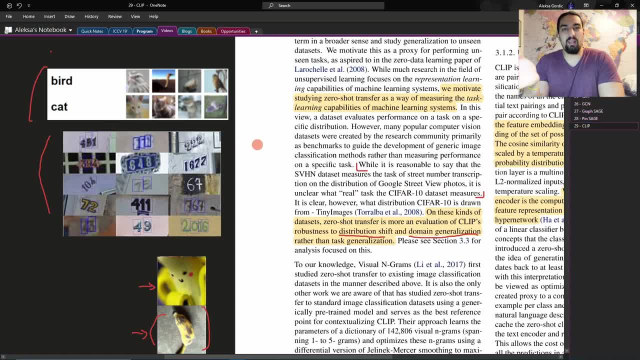 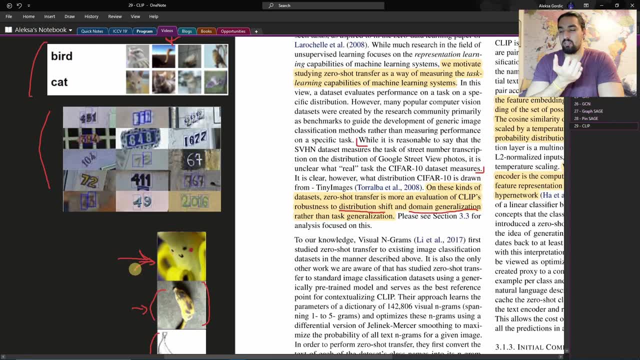 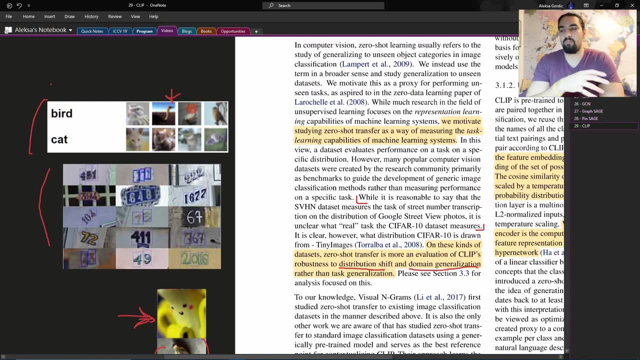 if you train the model on, maybe, ImageNet and then you want to test it on Cypher10, like this, you're basically doing what I already said. So you're doing basically just a different distribution and maybe some different objects, Whereas if you're testing on SVHN, 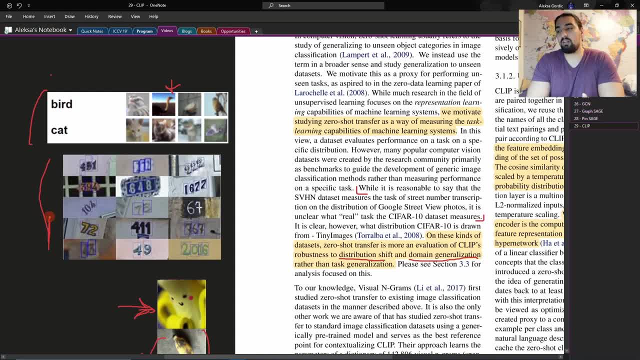 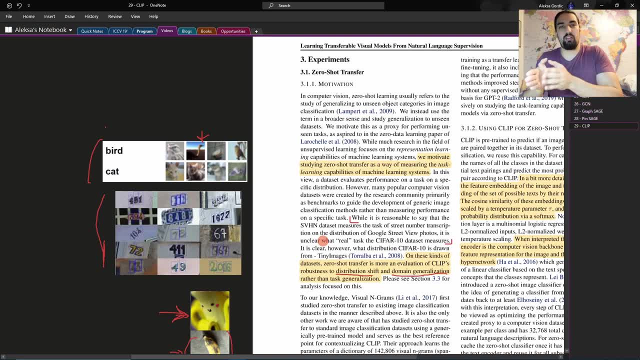 you're basically learning how to do OCR in the wild. If your model learns how to extract numbers from these images, So that's it. So we want to generalize, not only to distribution shifts and generalizations to new objects. we also want to generalize. 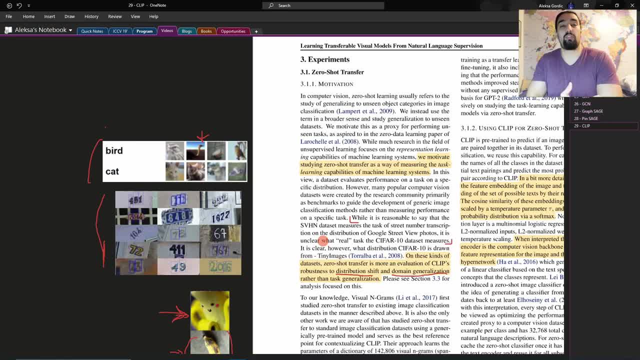 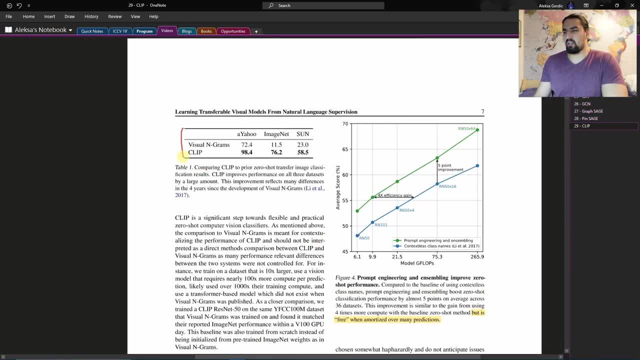 to new tasks like OCR, and not only to different classification datasets. Okay, Let's start exploring the paper First. this table is not so important, They just show So. visual engrams are a method from 2016, which had a similar notion. 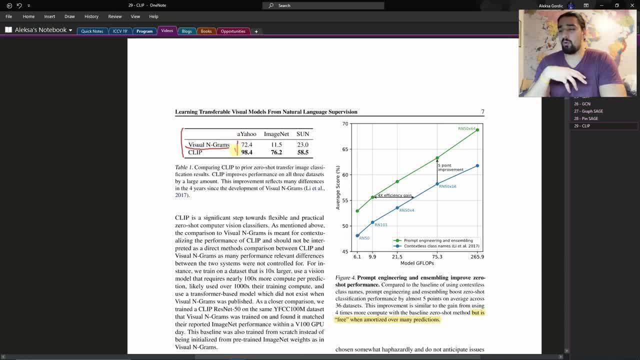 of zero-shot transfer, And that's why they compare with them, although it's not comparable, because many things like transformers did not exist back then, And so, yeah, they just have much better. Clip just has much better results on these datasets like ImageNet. 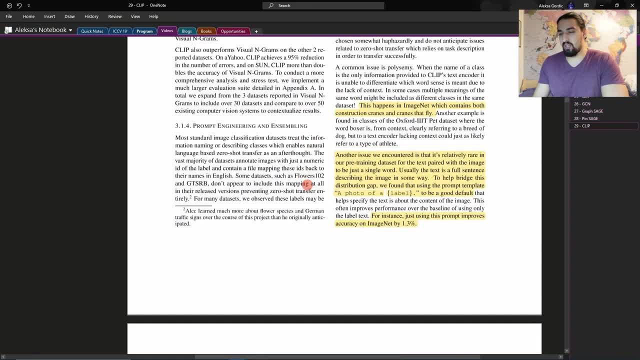 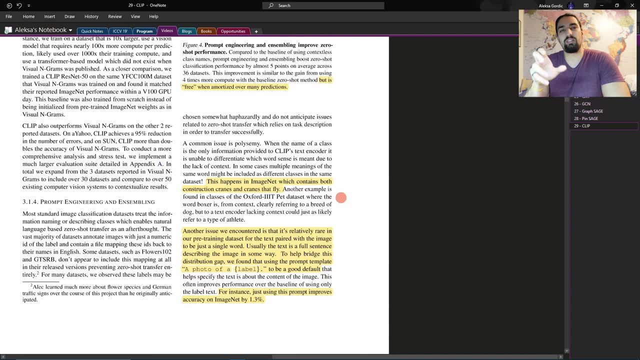 So before seeing the zero-shot and few-shot performance of Clip, let's first go through prompt engineering and assembling details. So the first thing they had to cope with is the fact that there is a polysemy problem in some of the downstream. 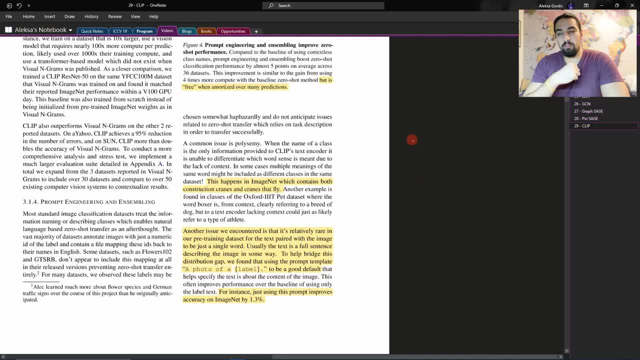 computer vision tasks And that means that, for example, in some of the datasets like ImageNet, you basically have two words which mean two different things, So different semantics. And maybe they give an example here: Construction cranes and cranes that fly. 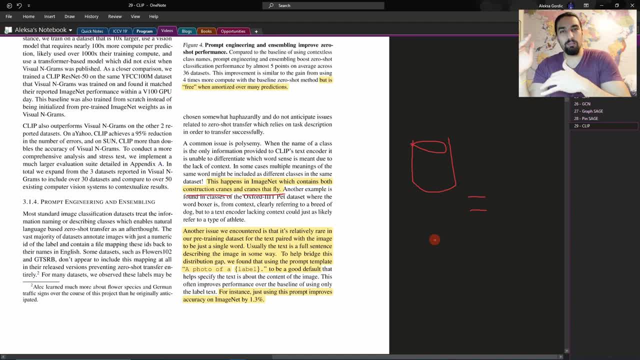 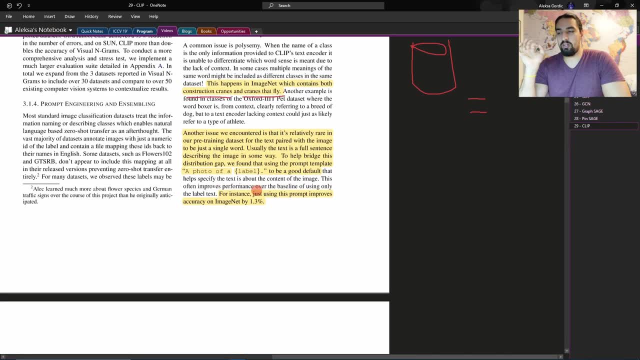 So the first thing they had to do is for a given dataset and labels, to disambiguate between those labels which have the polysemy problems. The second thing- and I already mentioned this one- is they had to construct the sequences like this: 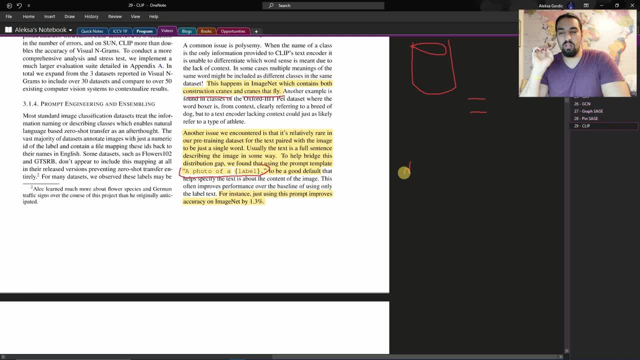 So instead of just using labels- So, for example, if you have on a downstream task you have labeled dog- instead of using dog in your zero-shot classifier to configure it, you use something like this: a photo of a label, And by doing that, 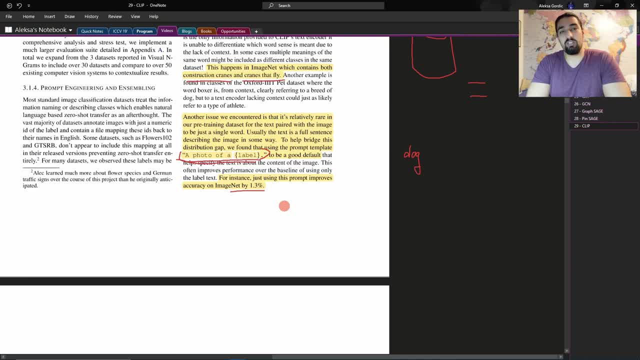 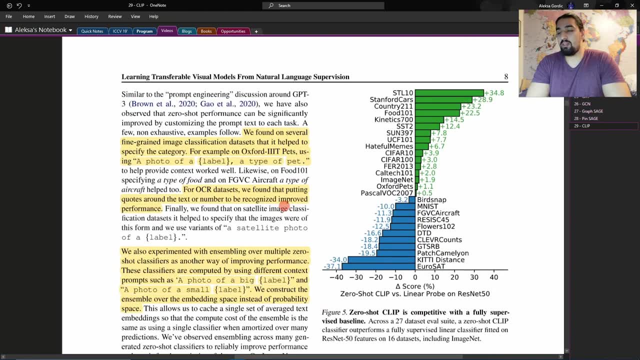 you get a 1.3% increase in accuracy, and that's like a low-hanging fruit. The second thing they did is again they play with prompt programming. So instead of just using a photo of a label, they also experiment with adding maybe. 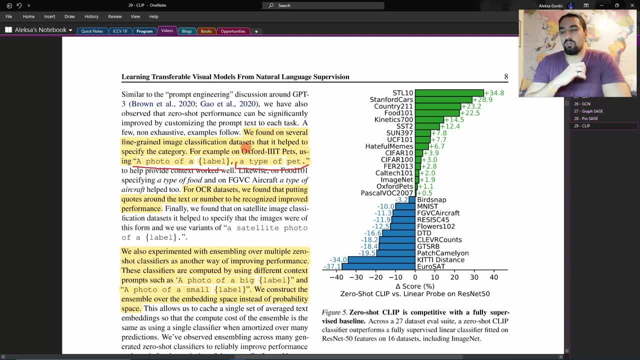 a type of pet, if that made sense for the. So we found several fine-grained image classification datasets that it helped to specify the category. So for example, on Oxford pets, using that one would even help them even boost the performance even higher. 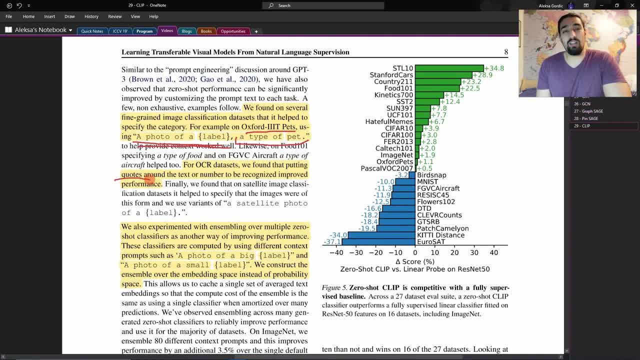 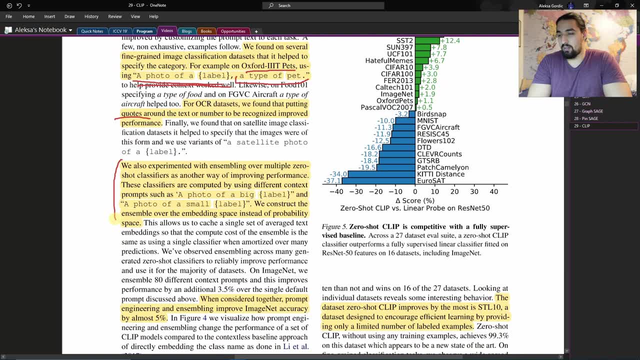 So, on OCR, just putting the quotes around the numbers would also gain, gave them some additional boost. They also played with ensembling, as I mentioned, So here is a concrete example. So by using a photo of a big 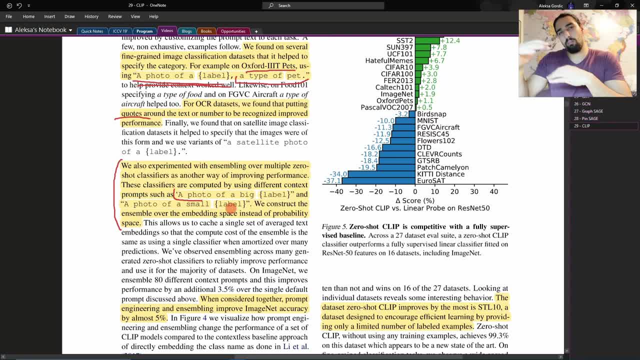 for example dog and a photo of a small dog, and combining those in the embedding feature space they get additional boosting performance. So they did not average in the probability space, They just averaged before they do the softmax and everything. So considering those two things together, 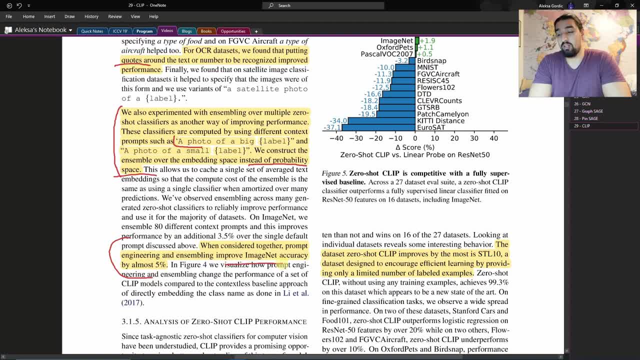 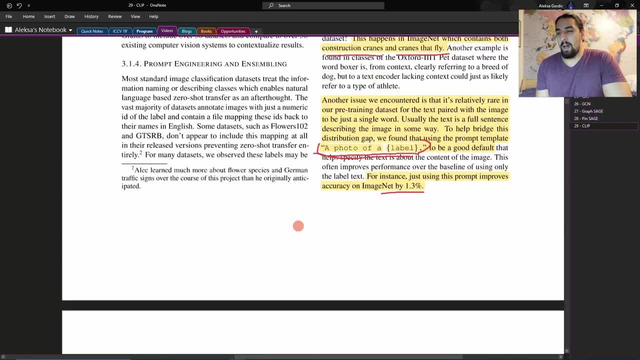 they get a boost of almost 5%, and that's on ImageNet. So that's a really low-hanging fruit and they made use of it. So let's see that on the chart here, Basically for a given compute. 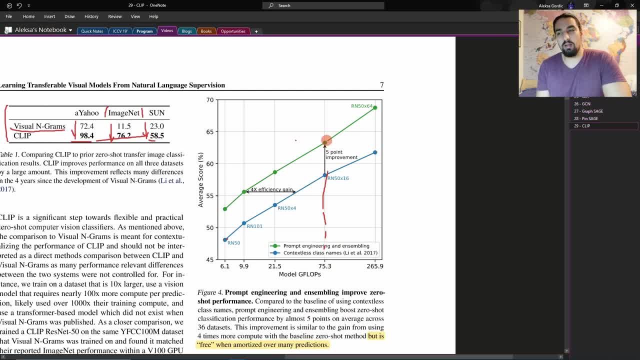 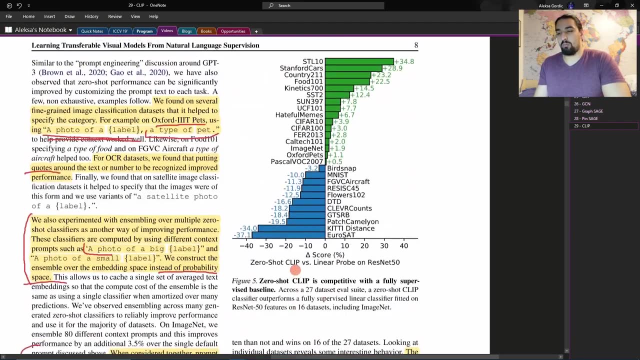 by just using those additional ensembling and programming methods, they just get huge improvements in the average score. So that's the first thing I wanted to mention. Now let's jump to the zero-shot performance of Clip. So what they did here is: 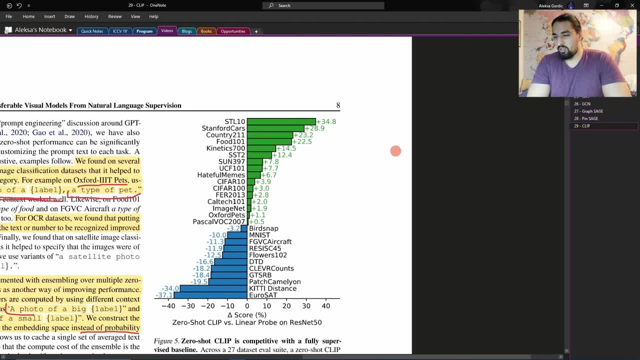 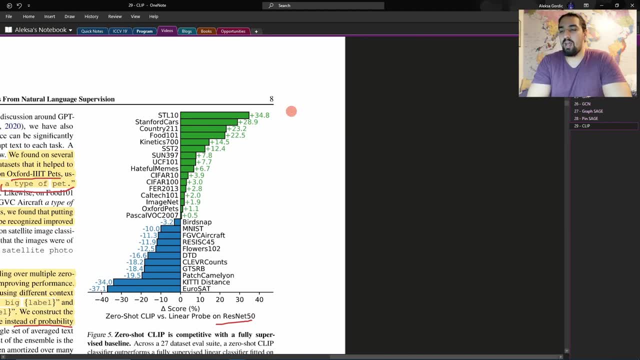 they took off-the-shelf models such as ResNet-100, I think no ResNet-50 here- and they just fully fine-tuned it on every single data set you see here. So they pre-trained it on STL-10,. 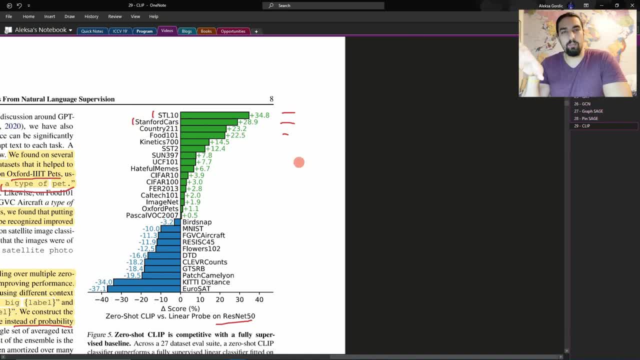 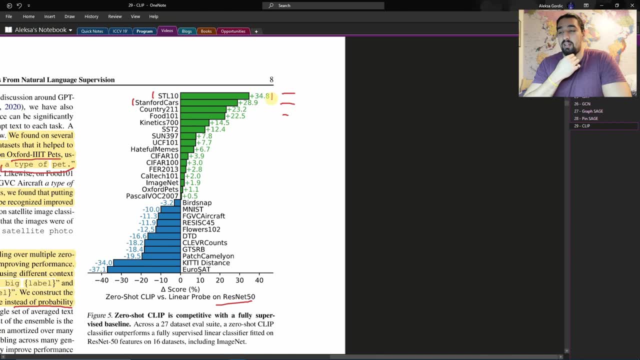 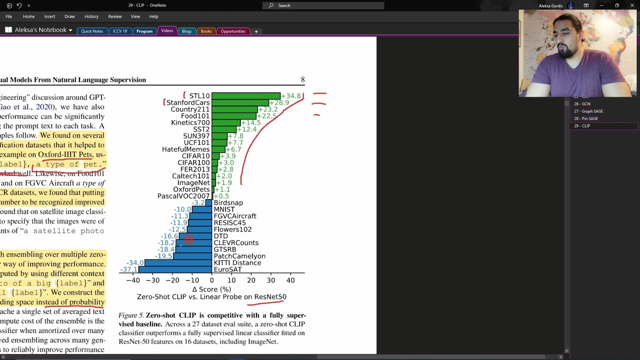 Stamford-Cars etc. And they took on the other side. they took Clip in a zero-shot setting and we can see that Clip is much better than fully supervised ResNet-50 on many of the data sets. And now, if we just analyze the extremes here, 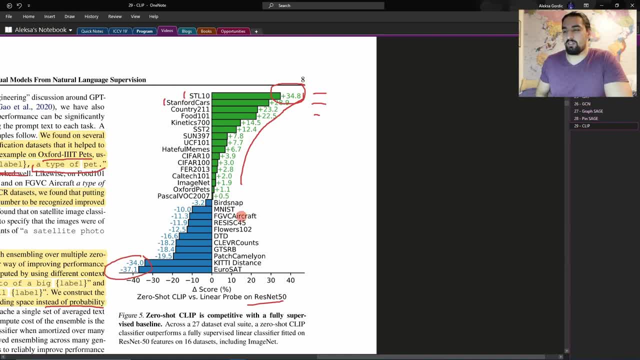 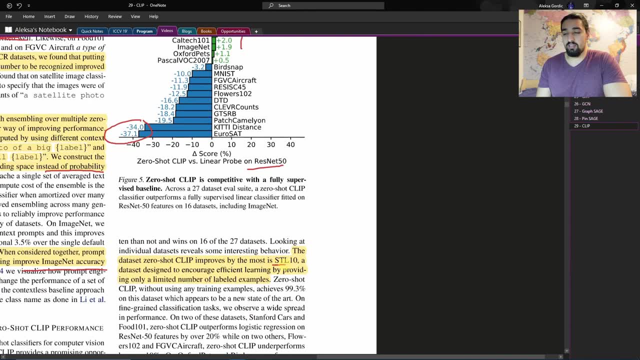 this part and this part that will probably give us some more information. what's happening here? So first things first, the data set zero-shot Clip improves by the most is STL-10,, a data set designed to encourage efficient learning by providing only a limited number of labeled examples. 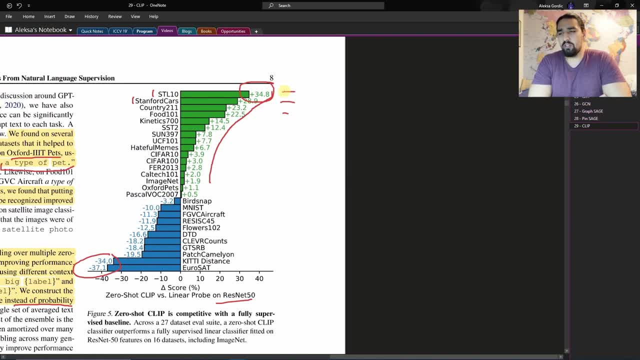 So what that means is that for this particular data set- because ResNet was- you basically take the ResNet features that we got from ImageNet and we freeze those and then we take the classifier and training that one. with this small amount of examples, 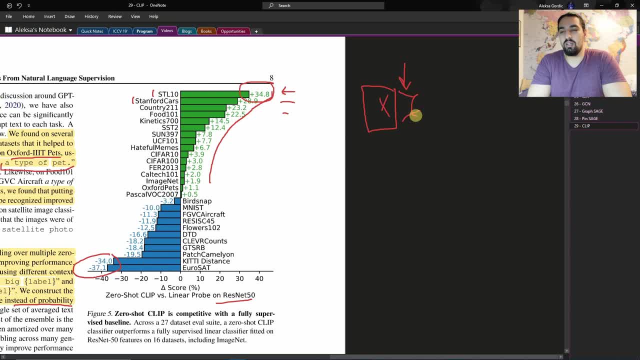 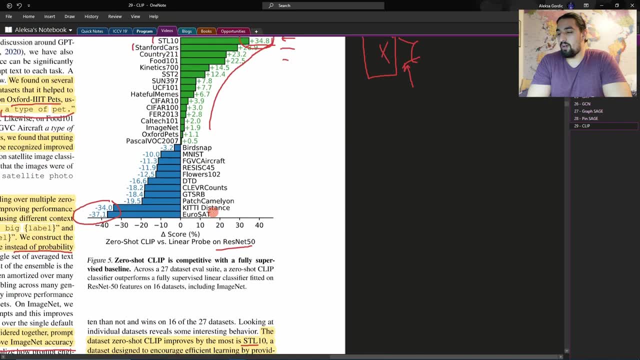 just didn't give us good results. So you can see that Clip was much better than ResNet. And, on the other hand, we have this other part of the spectrum where, if we analyze these data sets, you can see that these data sets 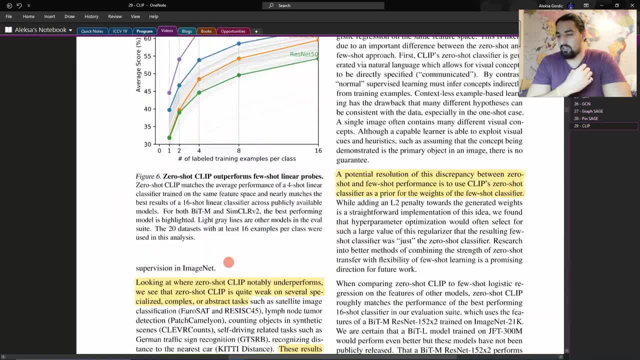 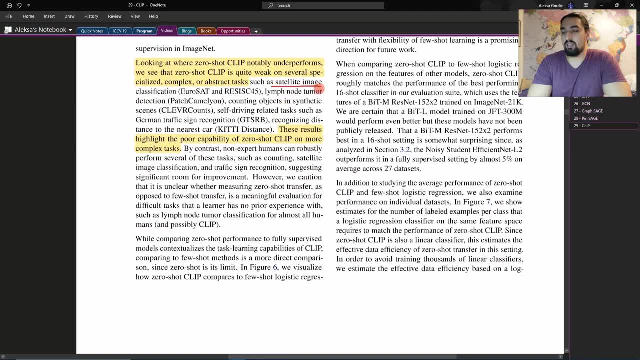 are complex and specialized. So they said here, looking where it underperforms, it works really weak on these data sets like satellite image classification, lymph node, tumor counting objects, blah, blah, blah, And these results highlight the poor capability. 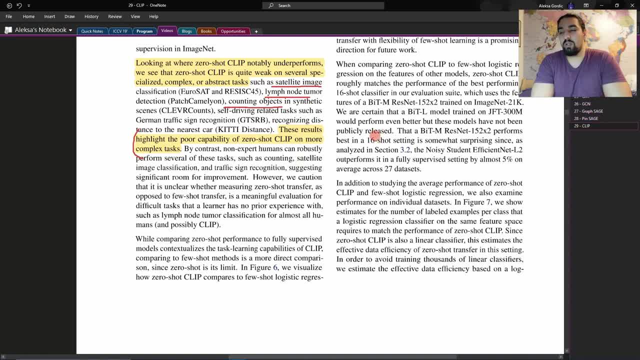 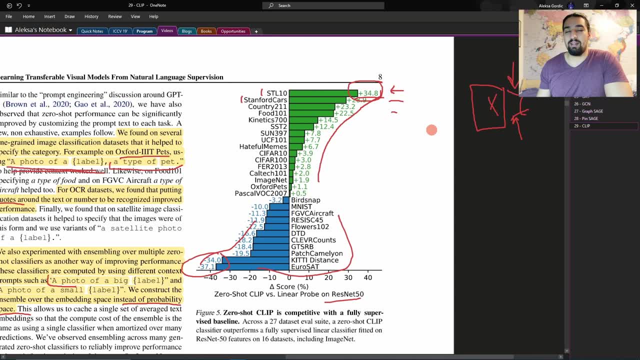 of zero-shot Clip on more complex tasks. So that's where it underperforms ResNet. But it's still quite fascinating that a fully supervised model using labeled information is underperforming Clip on many of the data sets, So it's worth mentioning, of course. 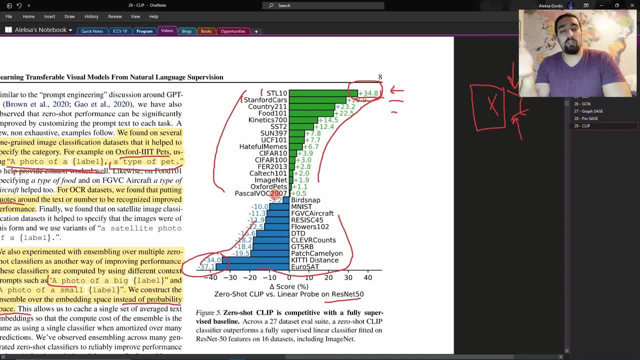 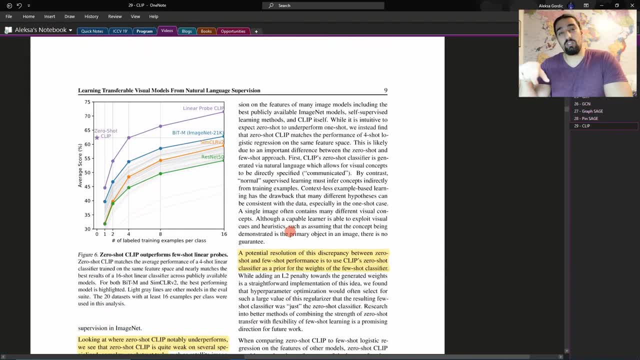 ResNet-50 is by no means state-of-the-art currently. So let's now examine what happens when we compare Clip with state-of-the-art, but in a few-shot setting this time. So these models are not trained like with all of the labels. 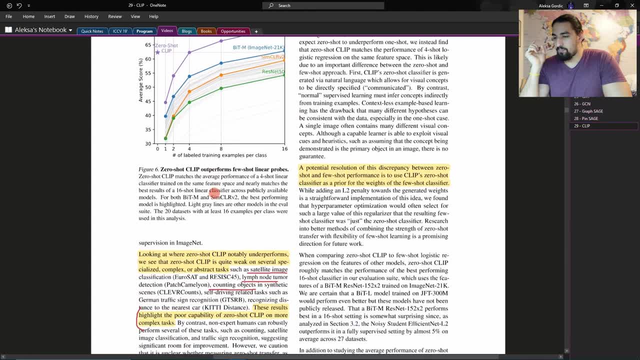 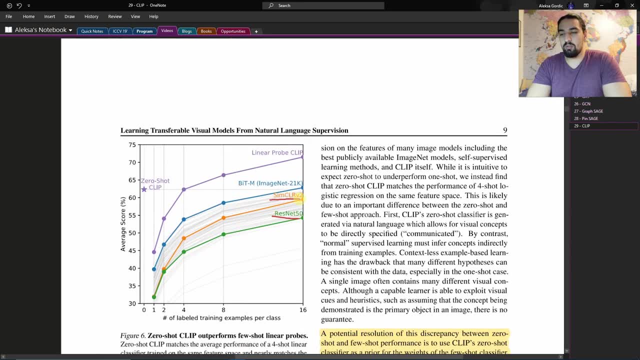 They just take a couple of labels. So let's analyze the chart. And they took three models. First is ResNet-50, SimClear, the self-supervised framework I mentioned, and Bit BigTransfer. So this one was trained on JFT 300,. 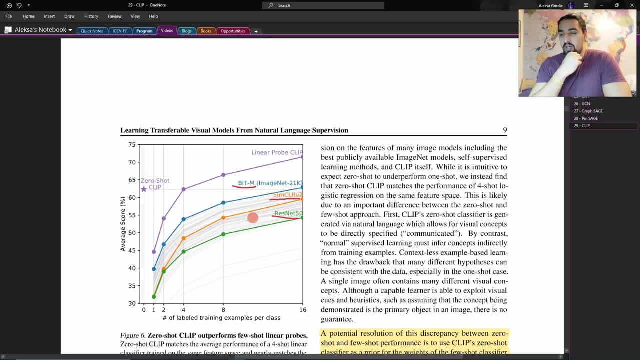 so a lot of data, And we can see that with 16.. So what we do here is we take those models like Bit and we freeze the weights, we add the classifier and we fine-tune on these data sets And we see that for 16 examples. 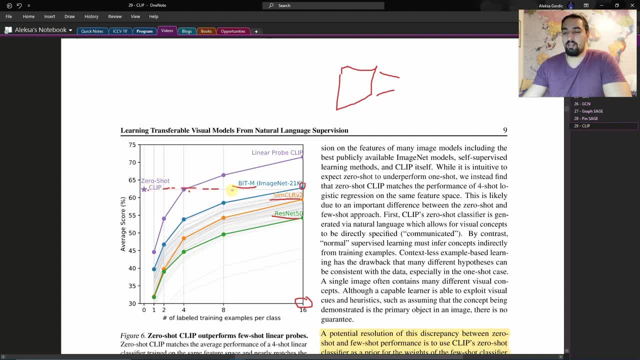 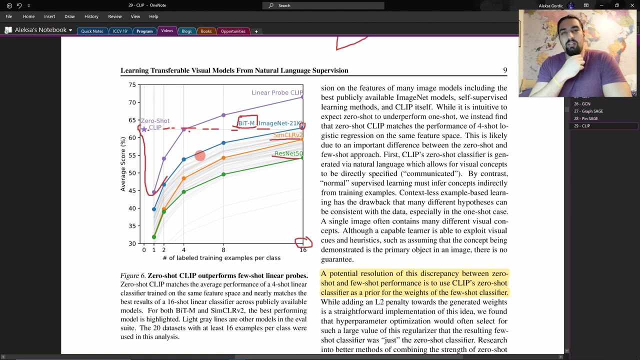 we are approaching the zero-shot Clip, which is a nice result because these are the best methods available currently, And what's interesting here is that there is this drop between zero-shot and one-shot And basically that discrepancy shouldn't be there in an ideal world. 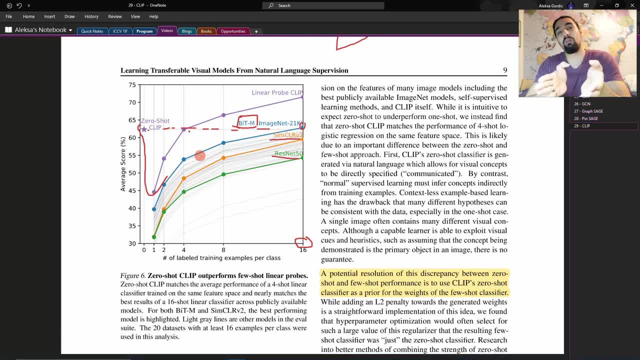 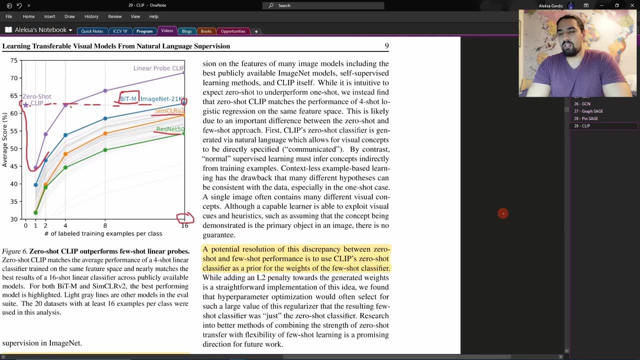 because humans, for example, when you give us one example, we won't be underperforming Like yeah, we'll be better. So that's something they are trying to work on And the potential solution they propose is just to initialize. 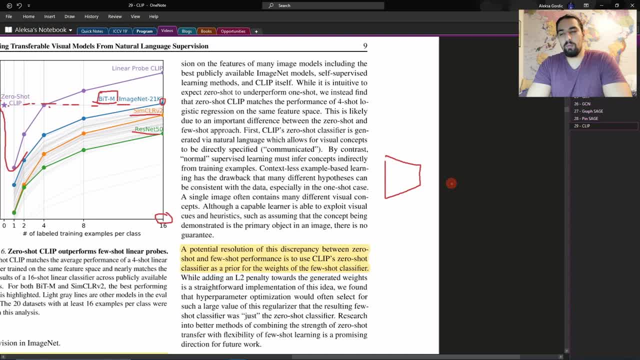 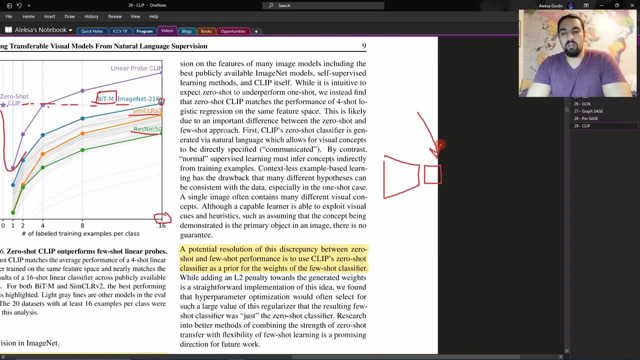 So you take the vision encoder of Clip and instead of training a classifier from random, they just initialize it with the zero-shot classifier as weights for that particular data set and use that. But that still didn't help them, so they just left it out. 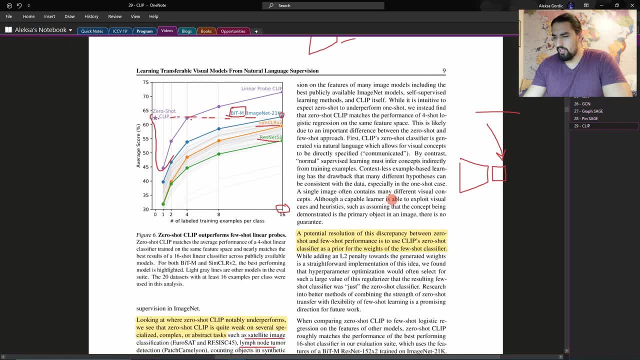 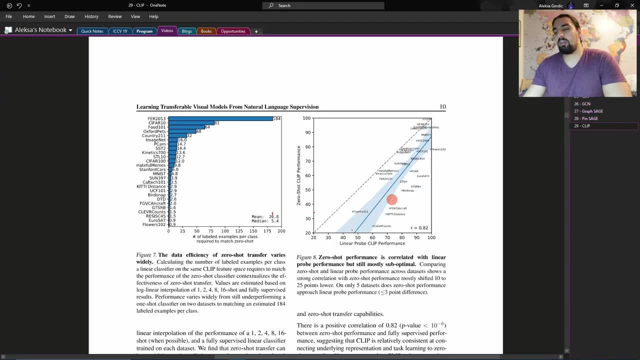 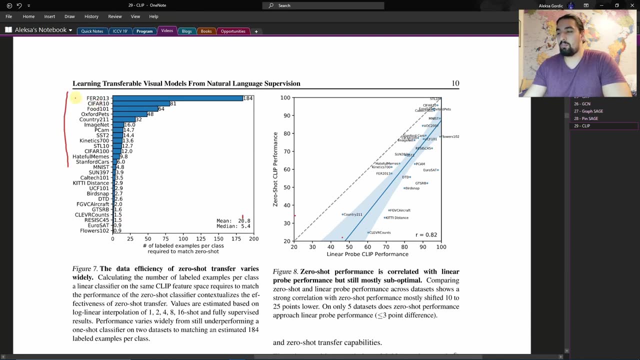 for the future exploration. Let's continue and see how good the zero-shot classifier actually is, And here we see. what we see in this chart is, for example, how many labeled examples do we need to achieve the same accuracy as zero-shot classifier? 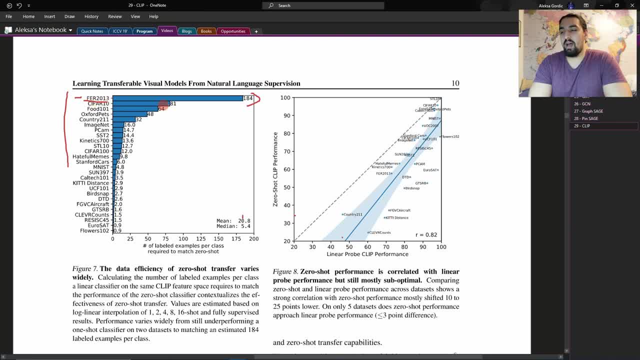 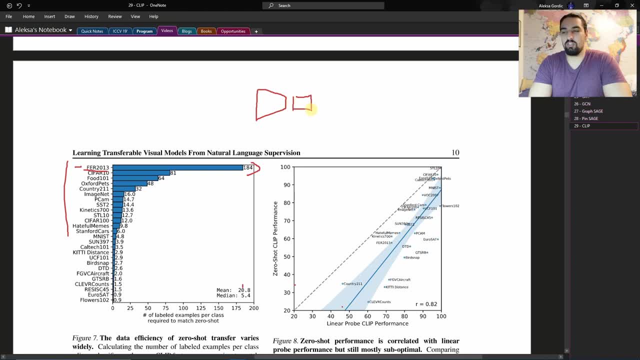 So for FAIR 2013,, if we just take that- the vision encoder of Clip- and use a random initialized classifier, we need 184 examples to achieve the same performance as zero-shot Clip. So that's a good result We want to make. 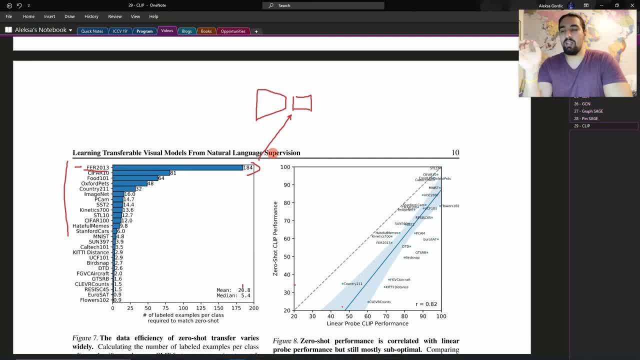 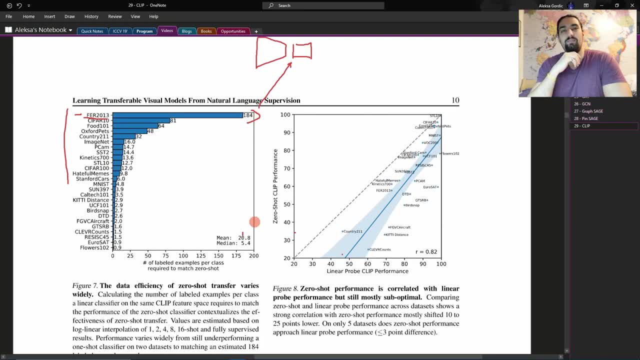 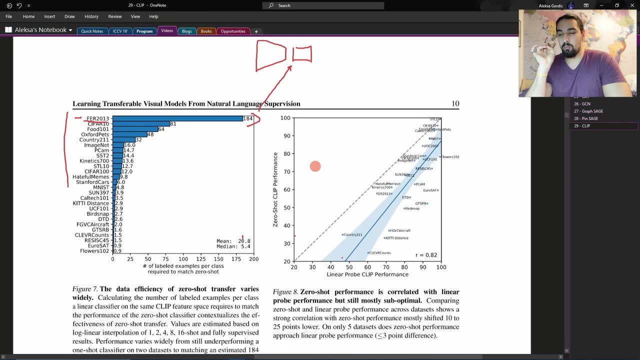 zero-shot classifier as good as possible so that even with a lot of labeled data, we can improve upon it. So that would be an ideal result. if every single data set required a lot of labeled examples to improve upon that randomly initialized classifier, That would be a good result. 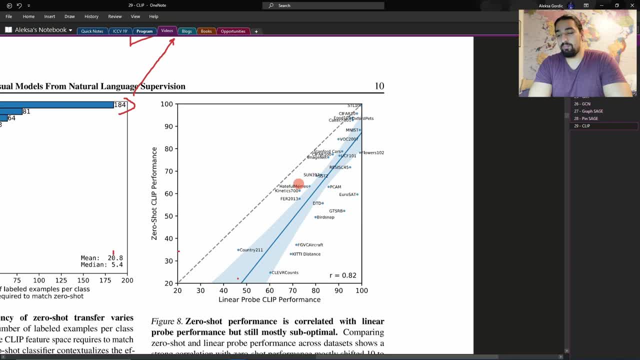 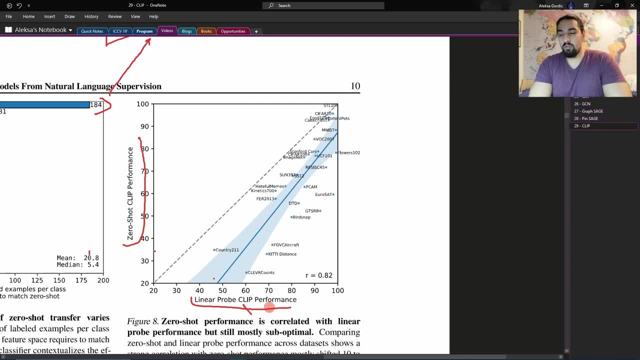 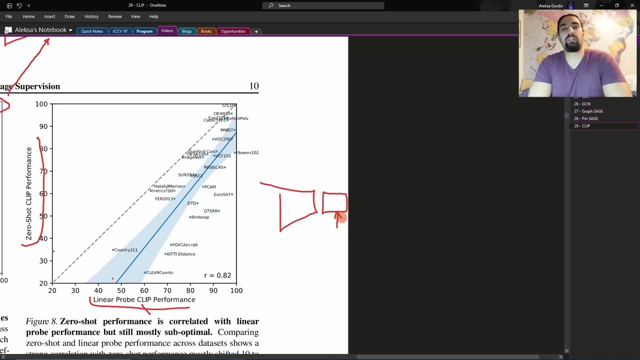 Here on the other chart, we can see the difference between a linear probe Clip performance versus a zero-shot performance. So this time you take that classifier and you basically train it with all the available data. So it's fully supervised and we use all of the data. 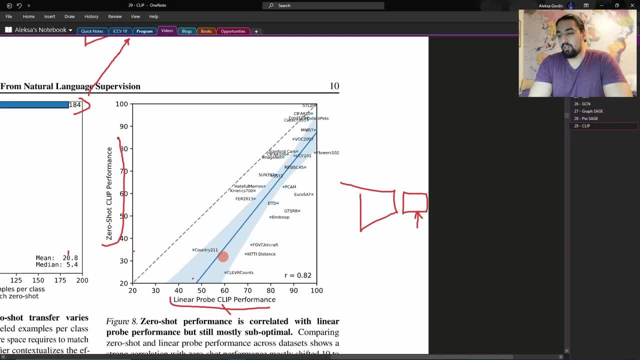 available in a particular data set, And we see that for a given data set, like maybe this one, the performance is maybe 45% once we leverage all of the data, but by using zero-shot we have only 35.. So obviously, 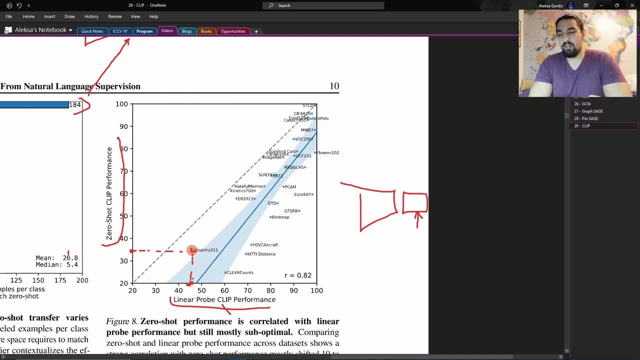 zero-shot classifier is suboptimal for this data set and we can see the general trend. So in a perfect world, zero-shot would be as good as this classifier that used the whole corpus of labeled data. But you can see the trend. 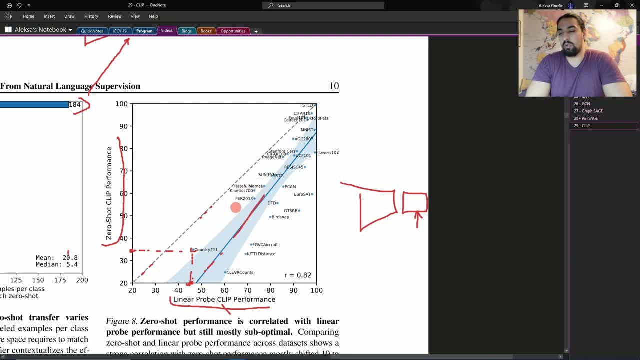 it's suboptimal and it's down by maybe 20 or 15 points And only a couple of data sets, like STL10, and if you remember that one has a small amount of labeled data available. So here the zero-shot performance. 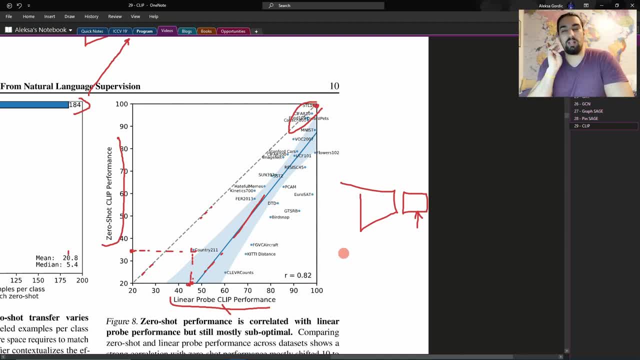 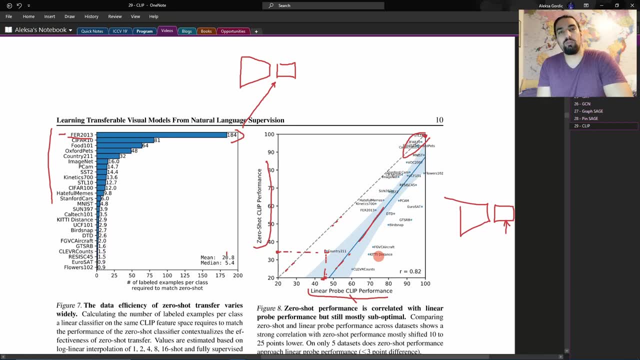 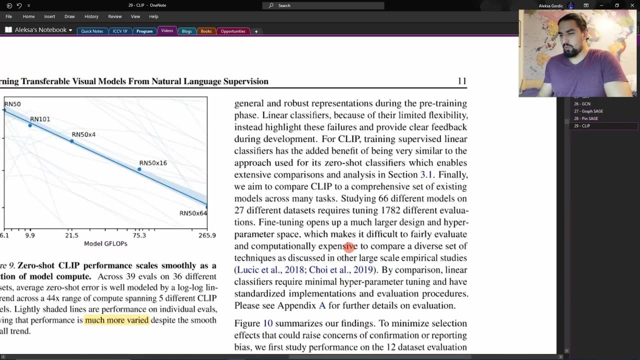 is similar to this fully trained classifier. So that shows us that there is a lot more space to improve upon this zero-shot classifier. Let's continue and analyze other charts, So this one. what it tells us is that basically increasing the compute. 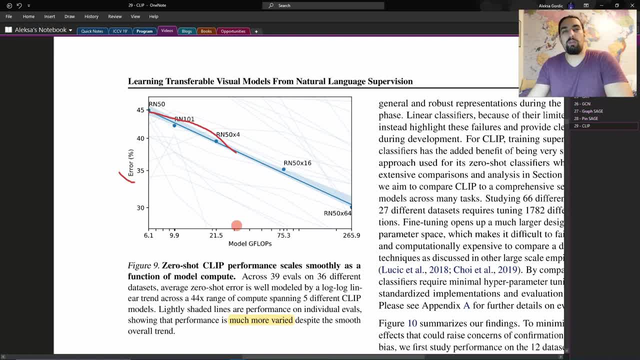 will decrease the error, which is something we could expect. But the interesting thing is it's really noisy. So if we take a particular data set, we can see that with compute sometimes the error increases and then it decreases. So it's really noisy. 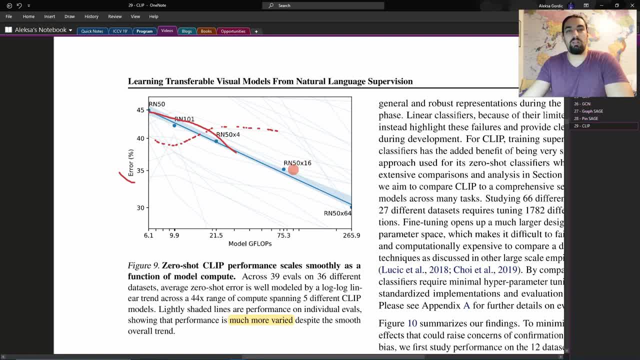 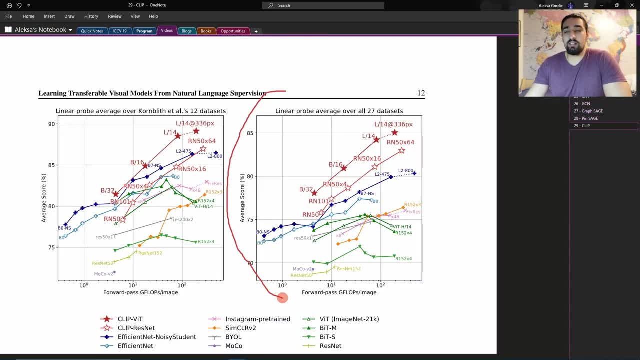 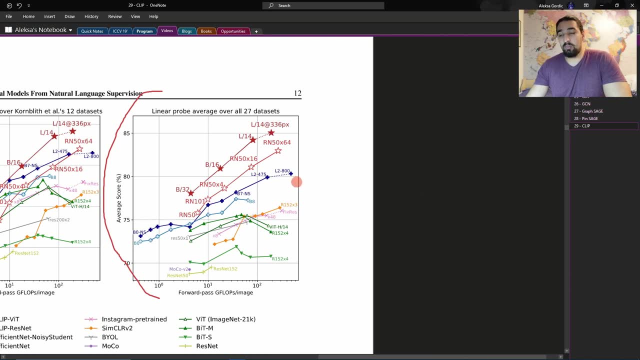 but the overall trend is still strong in favor of more. computation is better. Here what we see is that basically the feature space of clip is high quality because once we do, once we compare it with different models, like you can see here: EfficientNets. 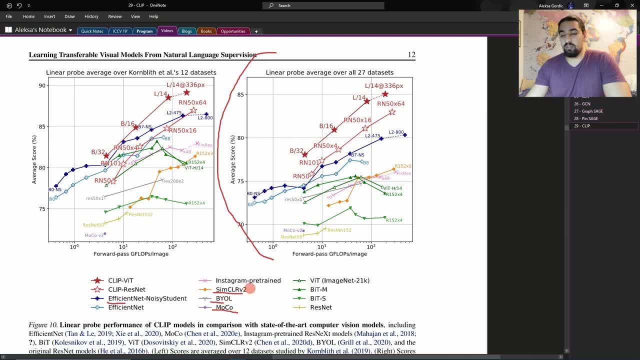 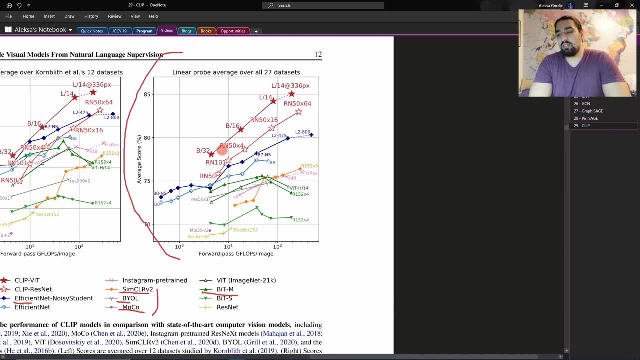 and Buell and MoCo SimClear, like self-supervised methods, and Bit, which is fully supervised. we can see that the feature space is higher quality for clip, And so what we see on this diagram is the amount of compute on x-axis. 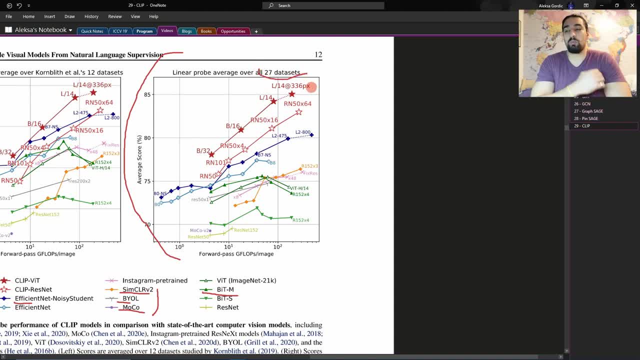 and the average score across a suite of different- like 27 data sets, And every single model was had. a had a linear probe, fully trained on the frozen feature space and clip again shows a much better, much better average score, which is something that we ideally want. 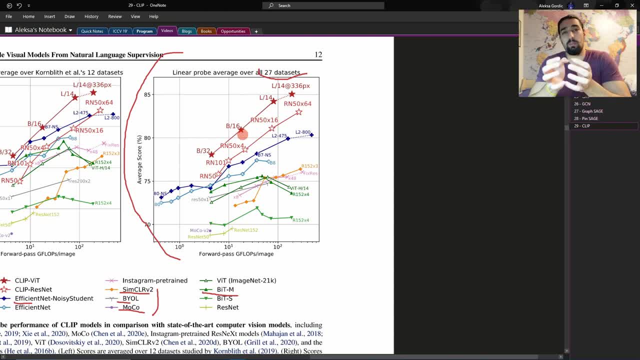 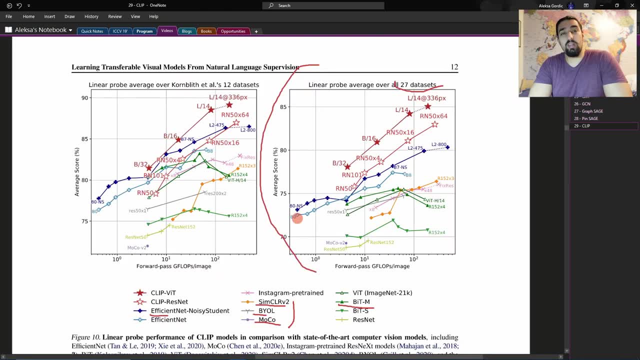 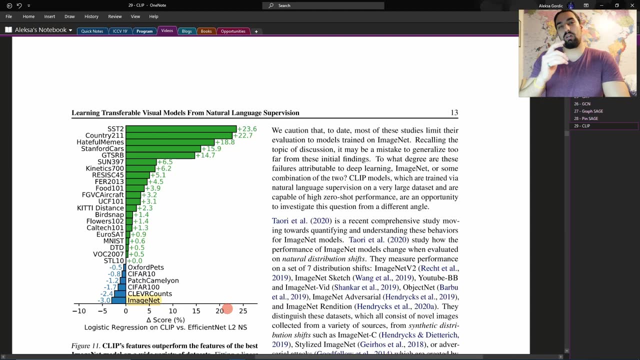 We want the clip to be. the features we train for clip are really good for many downstream data sets and it showed that here. If we take one specific model, like maybe EfficientNet noisy student, and we analyze, we break down those instead of using the average score. 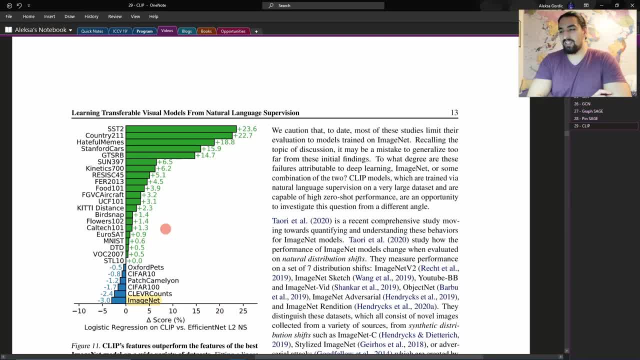 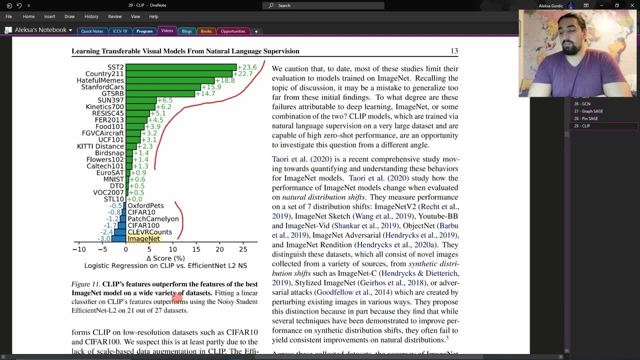 we just see the performance across every single data set. We can see where the the results for clip are much better and where it's a bit worse than EfficientNet, and because EfficientNet was basically pre-trained on ImageNet, so it does make sense that 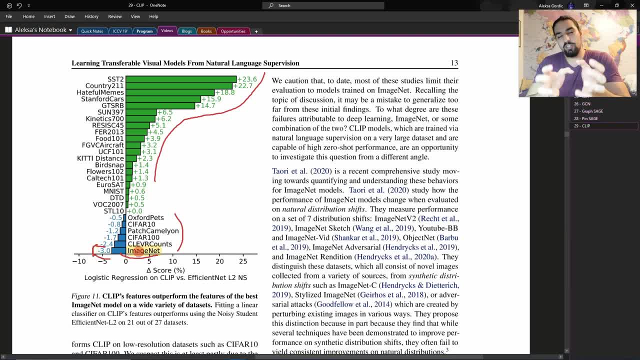 it has better performance than clip. That the feature space it developed is better for ImageNet, but only for ImageNet. As we can see on most of the other data sets, the feature space developed by clip is way more high quality than EfficientNet's feature space. 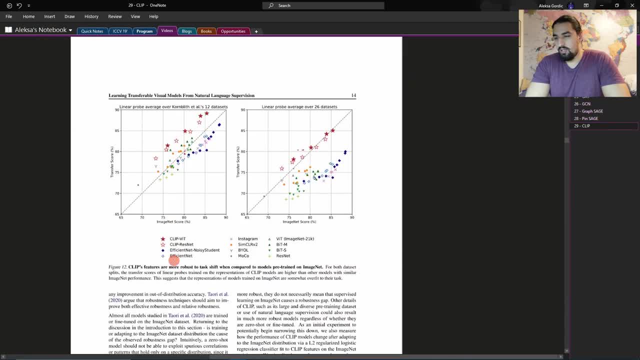 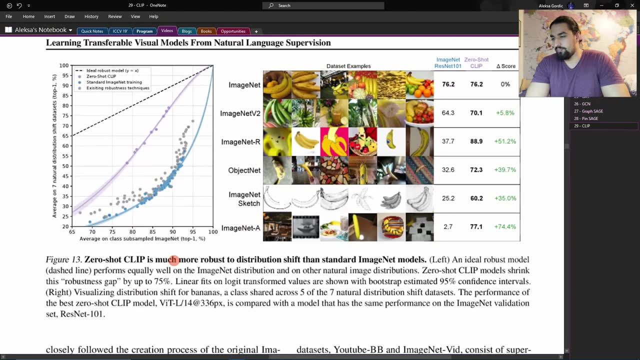 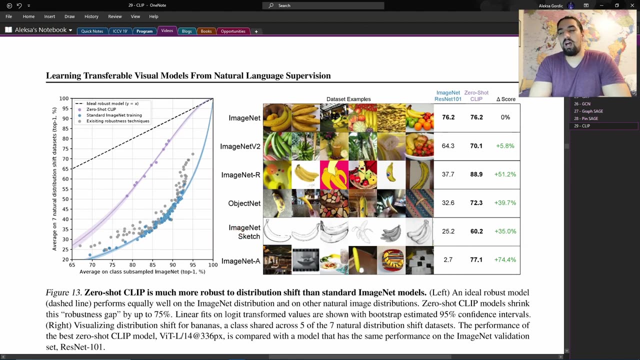 Okay, let's continue and see some other results. I'll skip this one, not that interesting, and I'll jump to this one. Basically, if we take what we see here, is the following: We wanna see, we wanna see how the clip accuracy behaves. 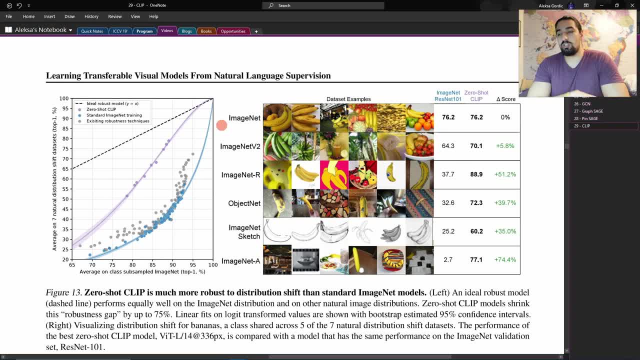 when we change the underlying distribution. so we see here basically same same objects, same classes, but like different distributions. So here we have sketches, here we have real world objects, some like again, some drawings, et cetera, And if we take, for example, 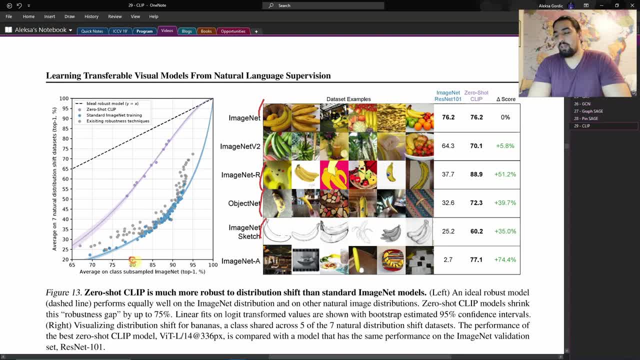 a model that had 80% accuracy on ImageNet top one accuracy. we see that for all of those standard ImageNet models that they severely have much lower accuracy on those other related datasets, just with different distribution, Whereas on the other hand, if we take the results for clip, 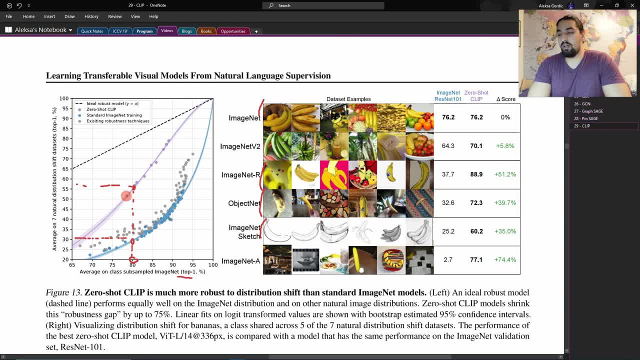 it has much higher accuracy than ImageNet wants And ideally again, if we have 80% on ImageNet, we want to have 80% on all of those similar datasets, just with different distributions. If we take a look at the tabular data here: 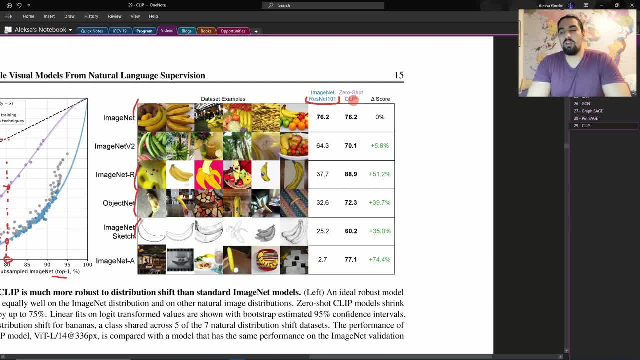 what we see is when we take Resonant 101- and so it was just pre-trained on ImageNet. We don't fine tune it on any of these new datasets with different distributions. We just use it as it is And we see that the performance. 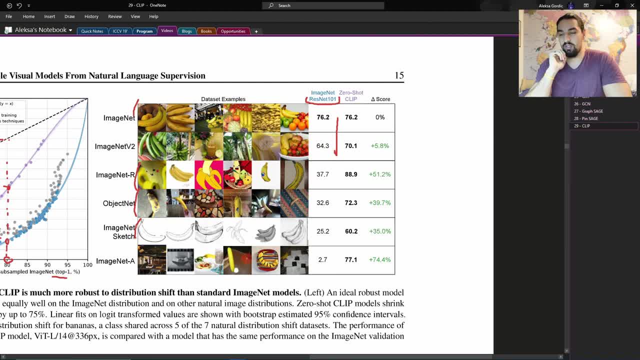 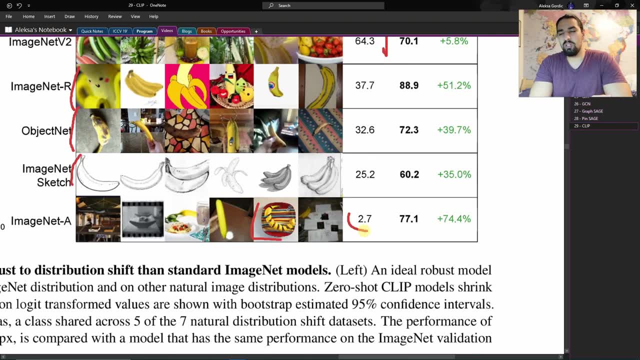 that the accuracy just severely drops. And for these adversarial examples, like you can see here, some chopped banana, something that the model never saw during training- it has really, really bad accuracy. On the other hand, clip's got much higher accuracy. 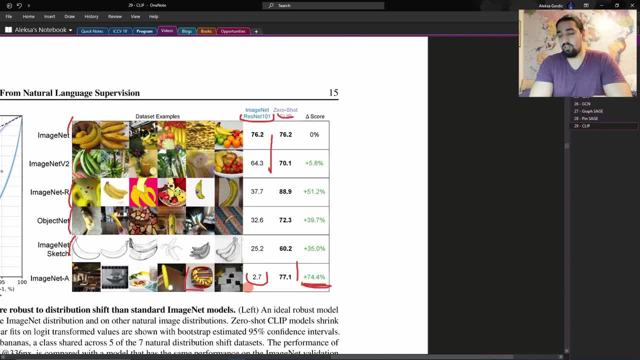 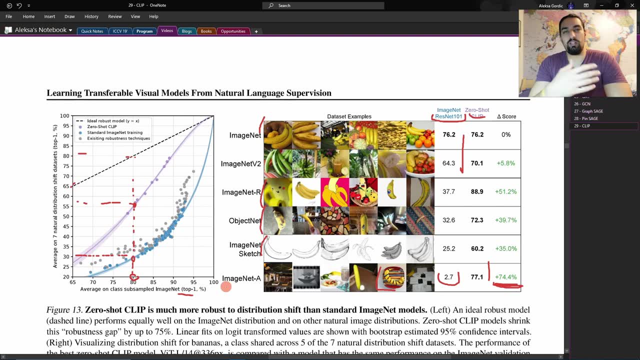 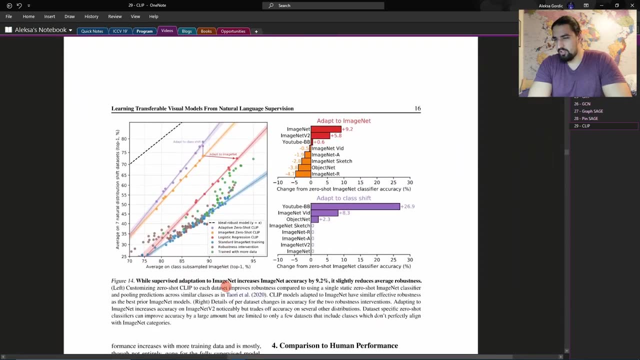 and it improves, like even 75% in this case, on this dataset. So that shows that clip is much more robust to distributional shifts than these other methods. Let's see some other results they showed, and this one is interesting, So this line is the same. 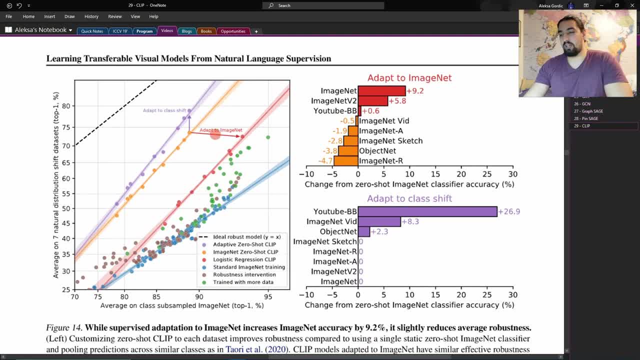 as the one above. So we just use clip in a zero shot setting And if we actually fine tune clip for ImageNet, we can see that even though it improves the ImageNet accuracy, the actual robustness to distributional shifts. so again we have those datasets. 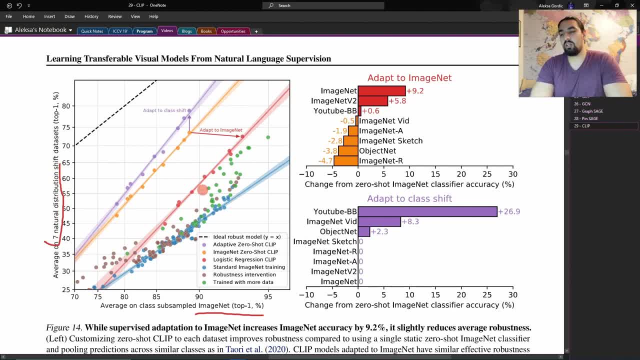 like those seven datasets. we see that the curves actually go down and it's less robust to all of those datasets. From another perspective, if we look at this chart, it has some improvements on ImageNet, whereas on many other datasets it just has less good performance. 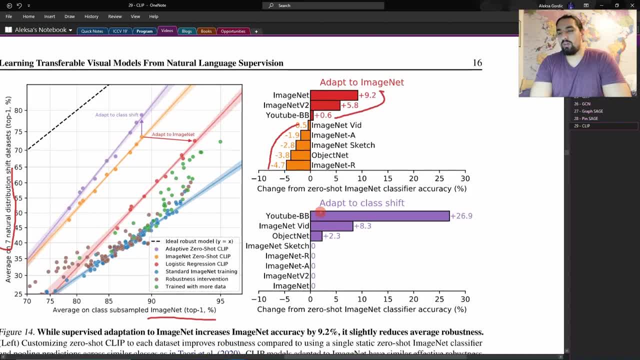 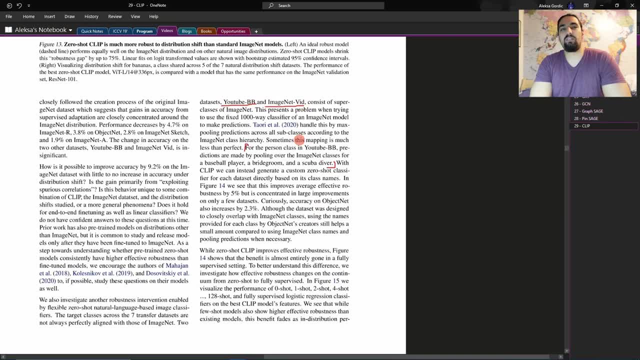 So was this adapted to class shift? So I think I noted somewhere here. basically because some of these datasets, like YouTube BB and ImageNet Vid, have different classes than ImageNet, which has a thousand classes. So for the person class in YouTube BB, 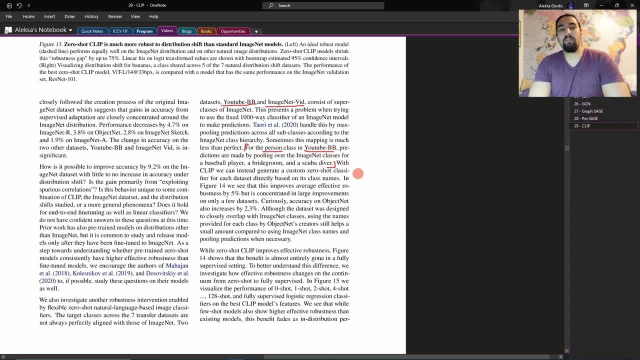 what we have to do for those ImageNet models is collect the scores over baseball player, bridegroom and scuba diver, and that's how we give the prediction for person on YouTube BB, which is suboptimal, But since clip is configurable. 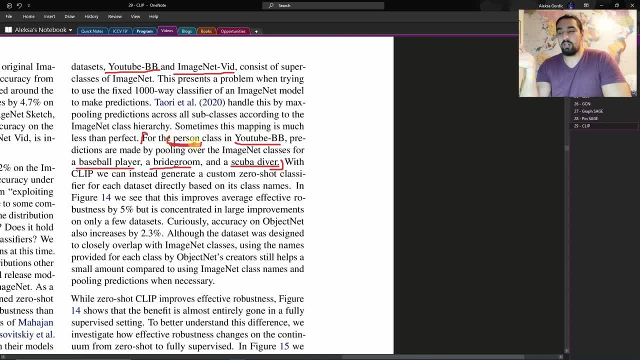 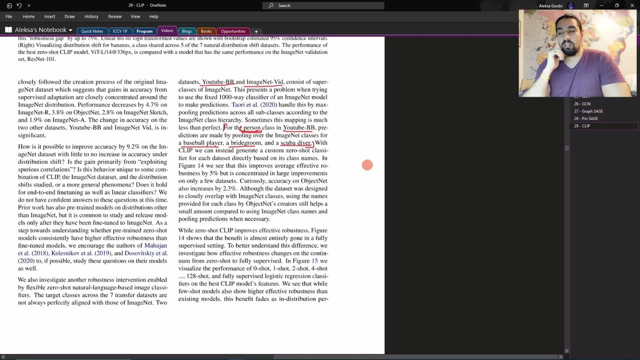 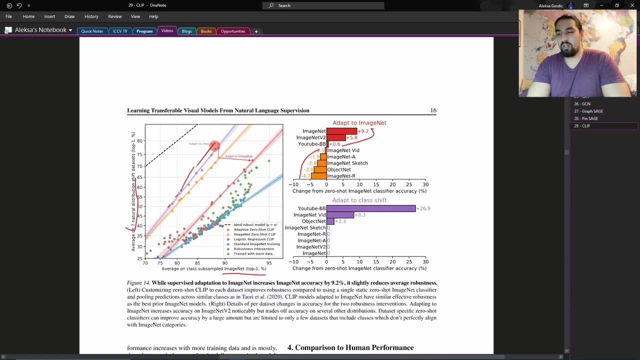 we can just use this new class and create the construction, a type of a person or whatever, to have much better results. So you have much better results than these fixed ImageNet models And when we do that we can see that the trend improves. 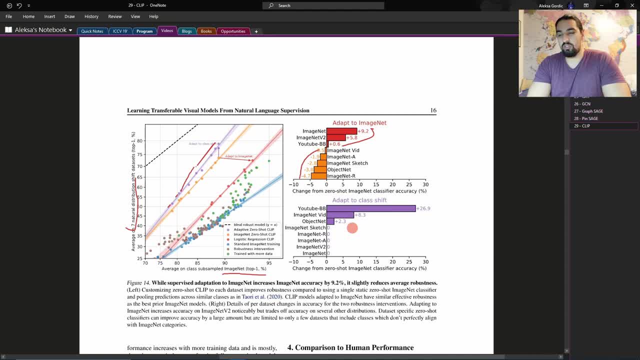 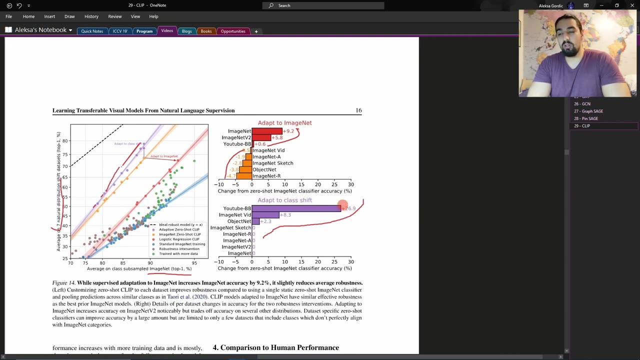 and the robustness increases further, which is really nice. And particularly on those couple of datasets which have that superset of classes, this small trick helps, Whereas the other methods, as I already explained, have to do the following. So, for example, 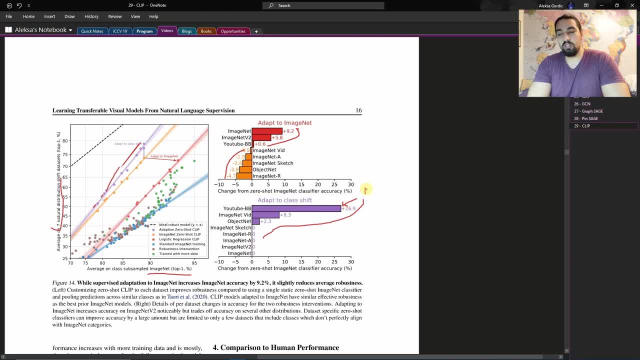 this dataset has maybe class person. So when we're testing EfficientNet we have to pull over three classes out of thousand, that it has to give an estimate of what person would be, since it doesn't know of the concept of a person, And on the other hand, 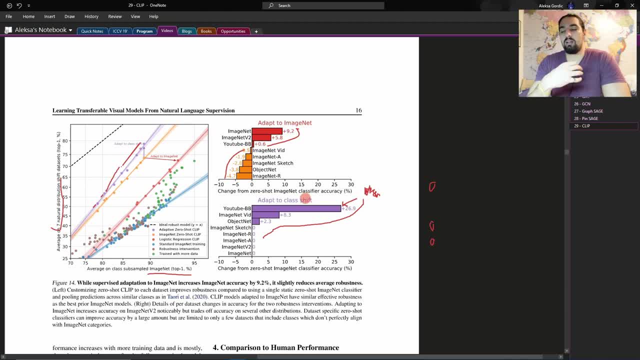 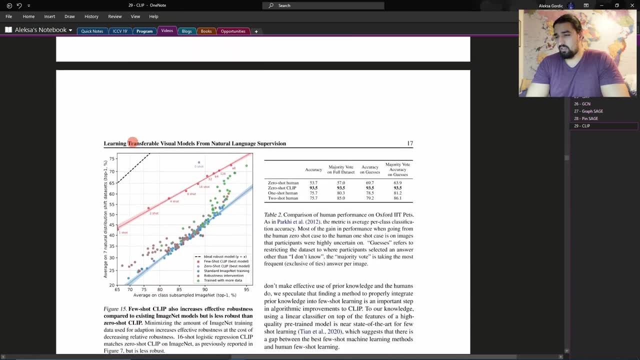 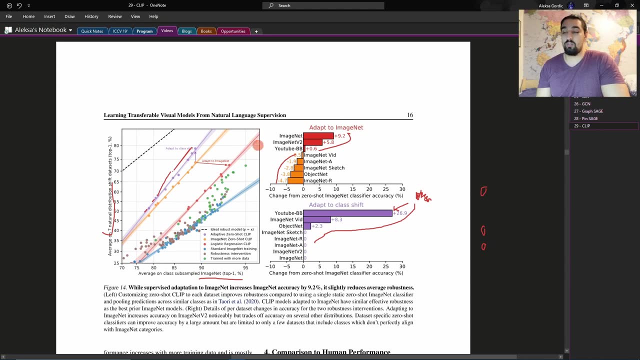 we can just use the flexibility of a zero-shot classifier and get the direct results instead. I'll just skip some of these, because this is serious. Similar experiments to these ones, It's just that instead of doing showing us the fully supervised curve. 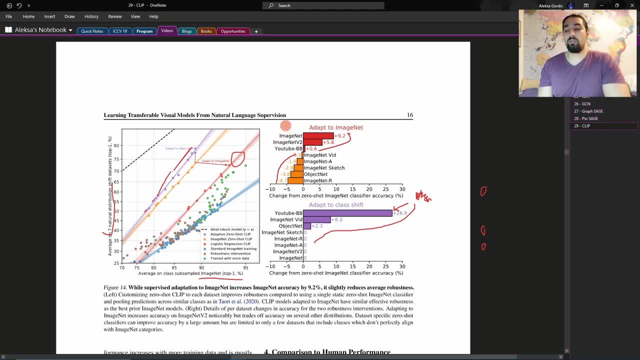 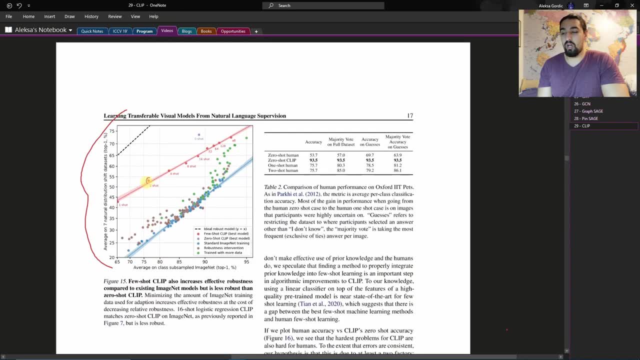 so this model is Clip that's fine-tuned to ImageNet, fully fine-tuned, And instead of that they just show a trend once we start from few shots. so two shots, four shots As we start increasing the number of labels. 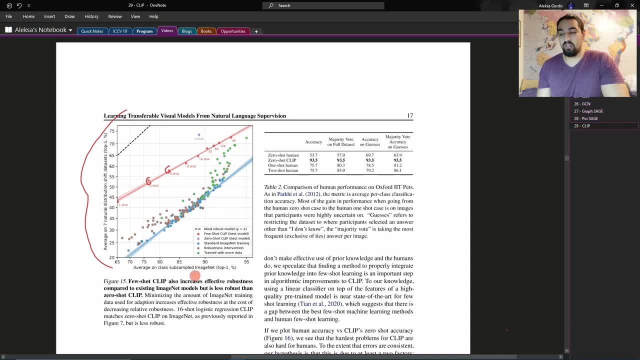 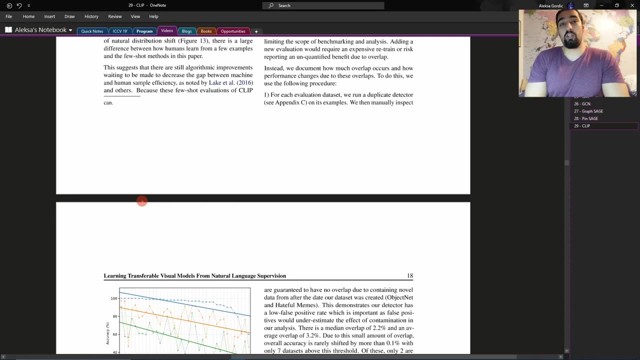 from ImageNet we can see that we are slowly increasing the ImageNet top one accuracy, but we're still underneath zero-shot Clip on these seven natural distribution datasets. Okay, there's a lot of information here. The main idea is basically that Clip's feature space 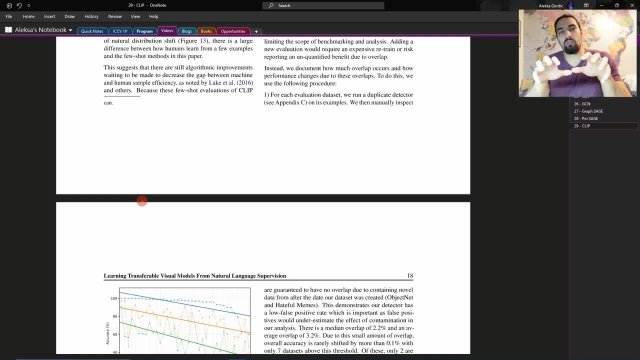 is way better suited to just extend to many other downstream tasks and it's much more robust, as we saw, to different natural shifts. So in a way it's a better way to and, additionally, it's not using those costly supervised datasets, It's just using those pairings. 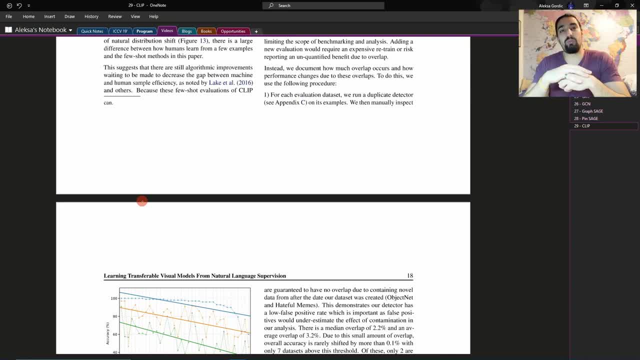 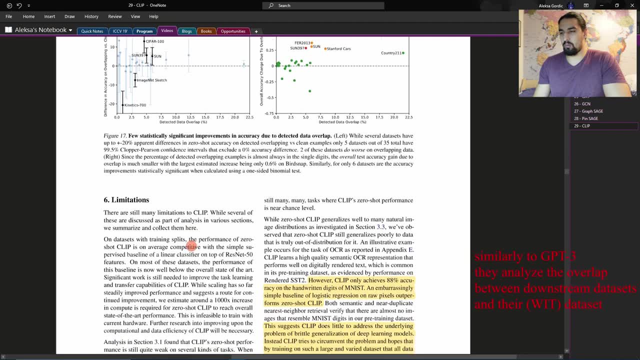 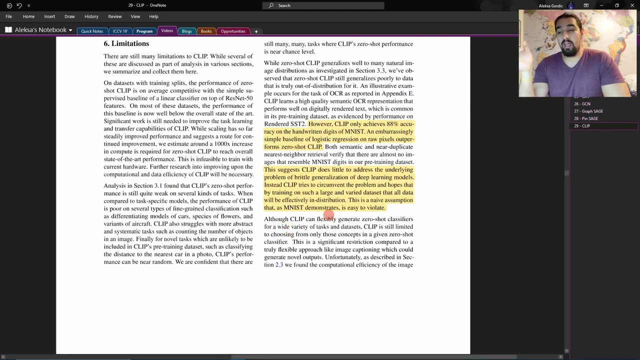 and so it's easier to just get a grab of that data. That's the main idea of the paper. This shows some contamination analysis and finally, I just want to show that there are some examples where it's not working really good and a nice example of a failure. 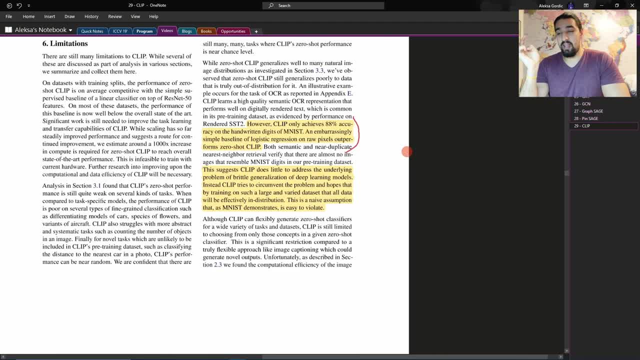 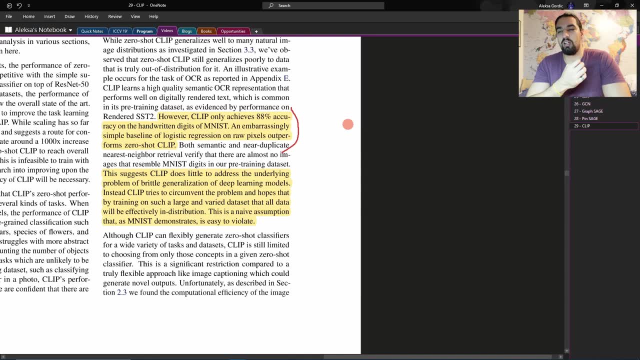 is on MNIST, where it achieves only 88% accuracy on MNIST, Just for comparison, if you take a simplest baseline. so you just take MNIST image, which is 28 by 28, you just flatten out the pixels and you use a simple feedforward net. 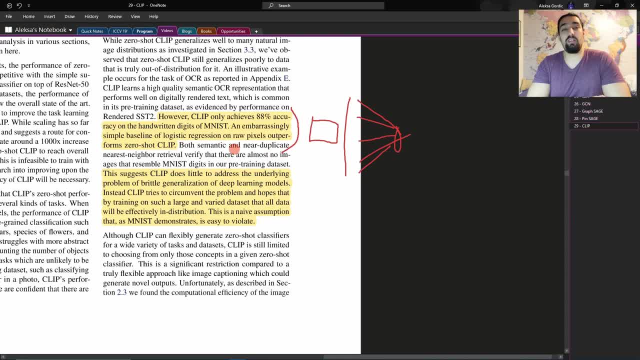 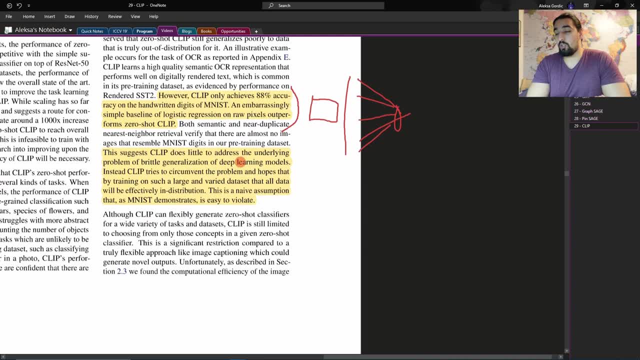 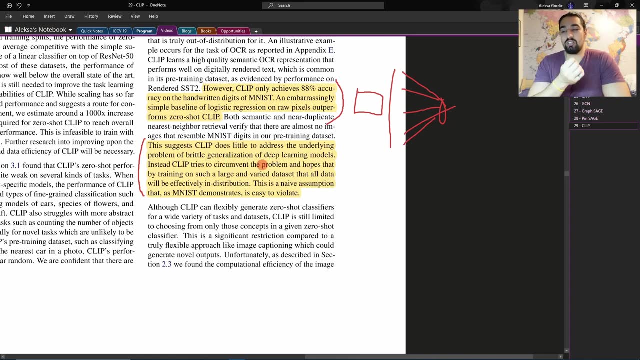 this one will achieve higher accuracy than Clip, which was trained on a lot of data and lots of compute, so it really failed on MNIST. So, as they say here, this suggests Clip does little to address the underlying problem of brittle generalization of deep learning models. 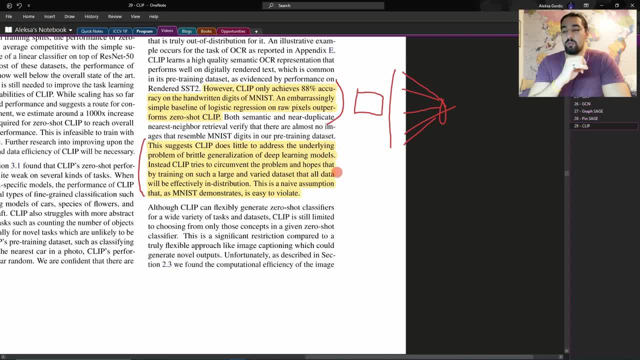 Instead, Clip tries to circumvent the problem and hopes that by training on such a large and varied dataset that all data will effectively be in distribution, and this is a naive assumption that, as MNIST demonstrates, is easy to violate. So obviously this is not the final way to go. 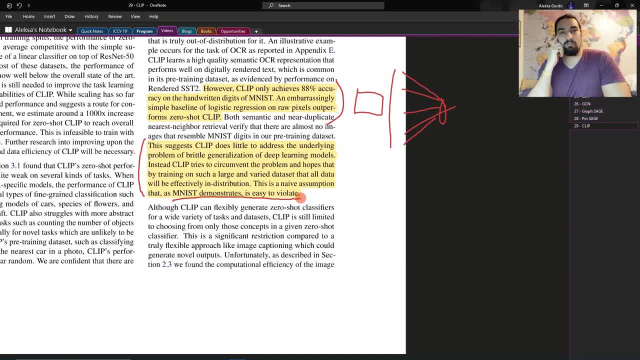 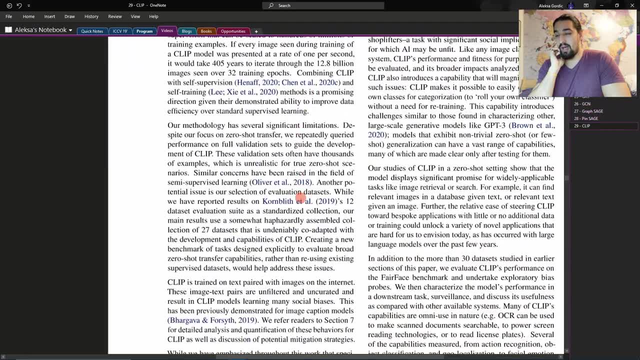 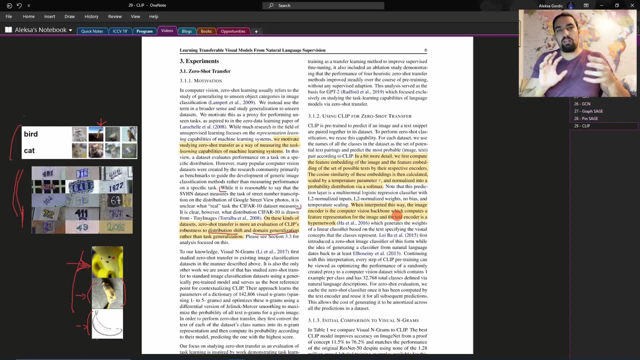 towards really generalizing to really general models, but it's a step forward and I'm excited about this work. So, yeah, that was pretty much. it A short recap because there was a lot of details and hopefully this will make it kind of consolidate in your head. 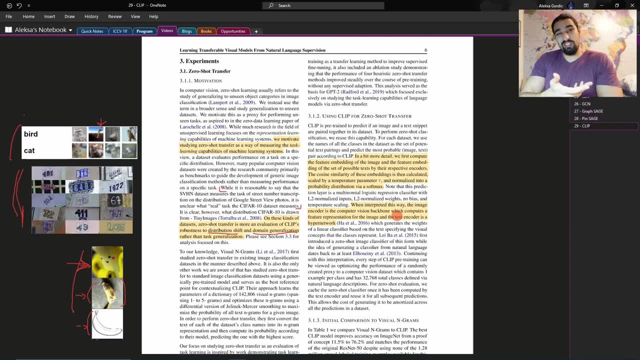 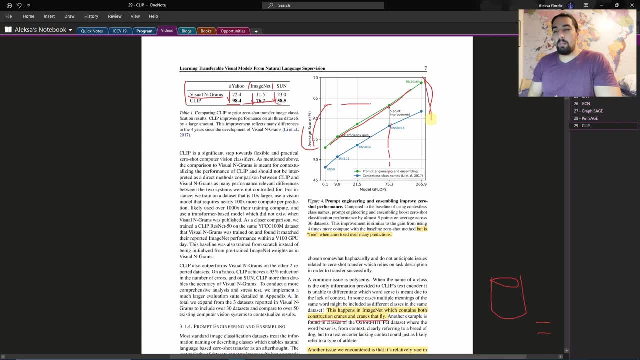 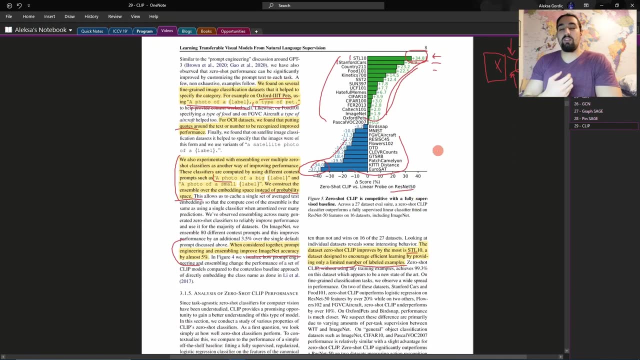 And so they care about zero-shot performance generalization to new tasks and not only new distributions and domain generalization. They show that prompt programming and assembling does help boost the performance of Clip models, so that's important. They show that even against a fully supervised baseline. 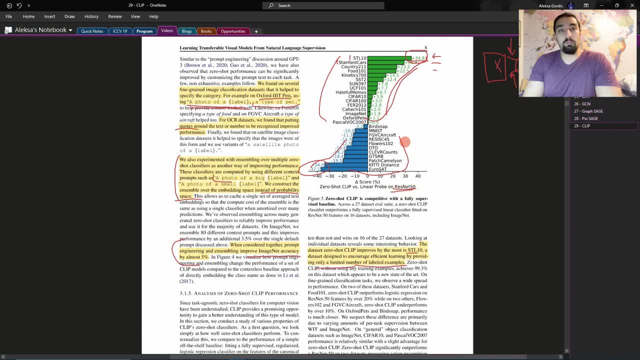 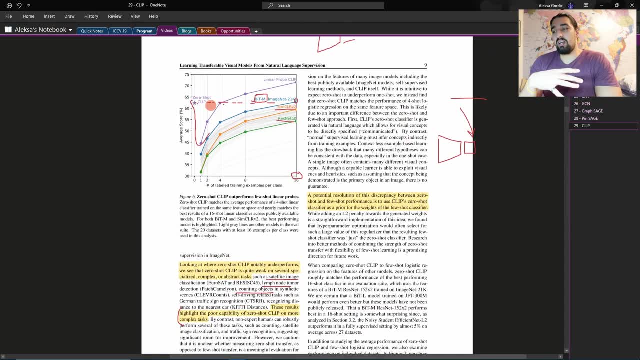 such as the ResNet-50, they are comparable and those are exciting results. They show that even against the best baselines in a few-shot setting, they are comparable in a zero-shot setting and they are better when they are doing the same thing. 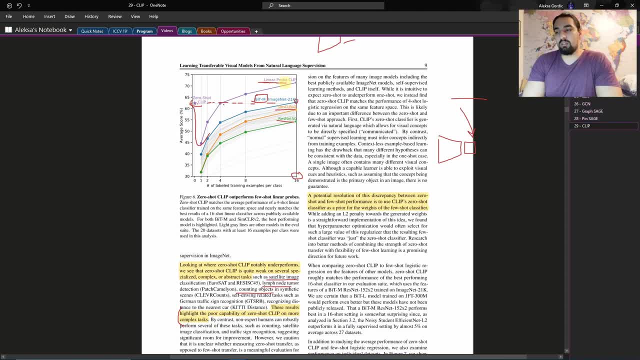 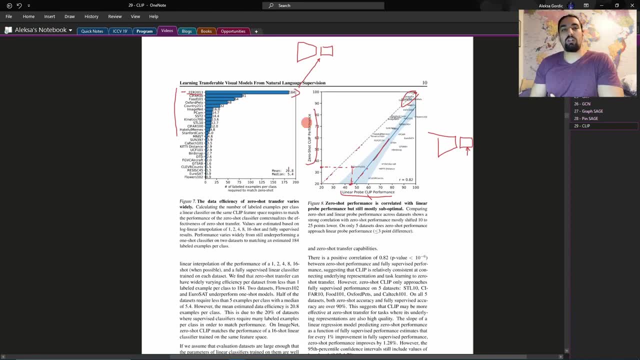 when they are also fine-tuning their model, ie linear probing, actually here. Next, they show that zero-shot classifier can be further improved. It's suboptimal to the classifiers which are imaginable by just fine-tuning them on specific datasets. 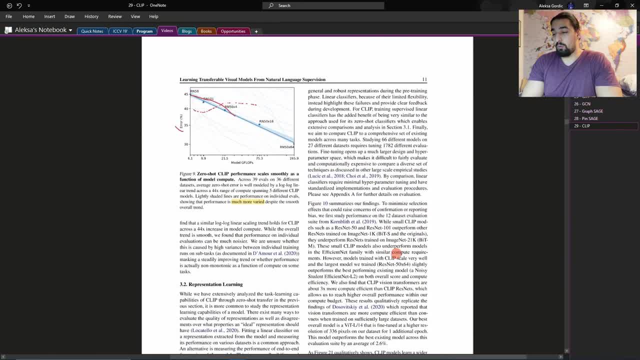 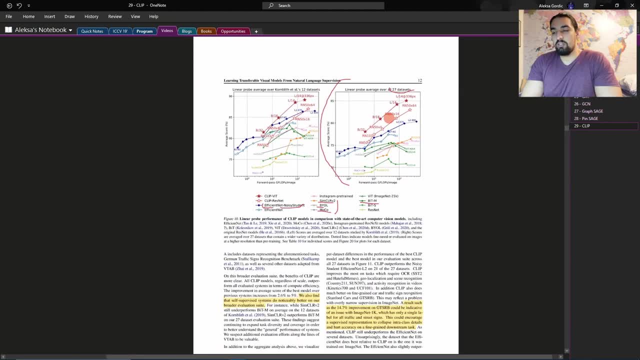 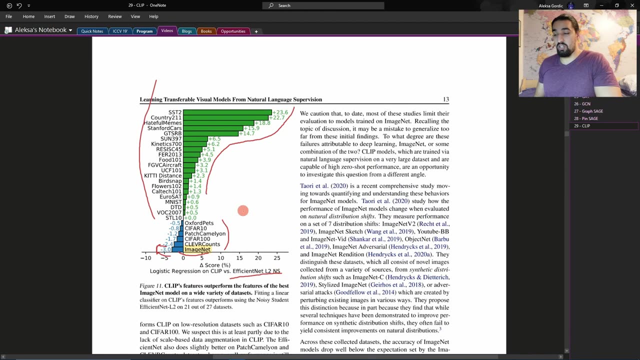 So there is more work that can be done on improving that. Again, compute does improve. Clip features are better, so feature space that Clip provides is better than other baselines and compared to for a specific baseline, EfficientNet, here we can see that it's much better. 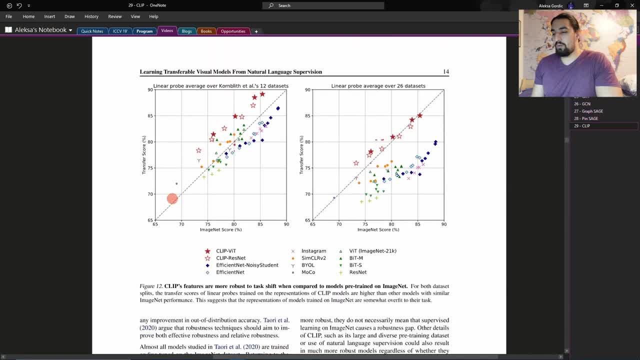 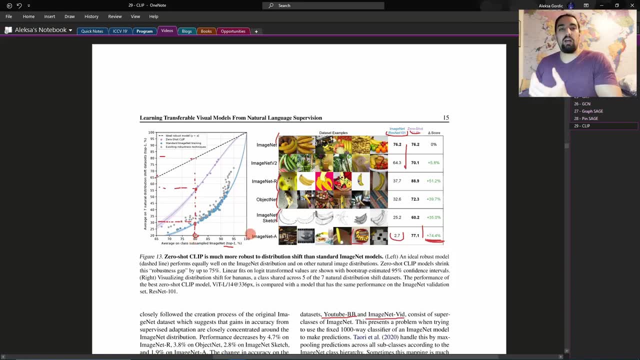 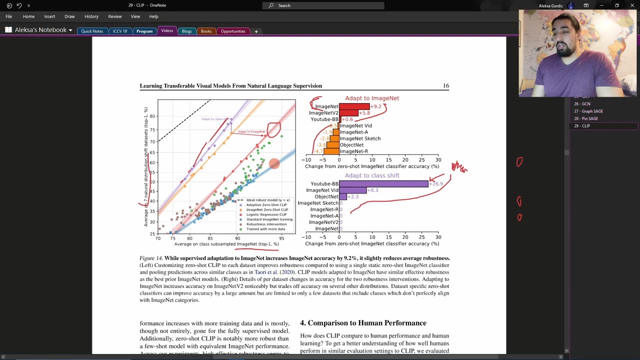 on many datasets. So again, feature space is richer than the other baselines. Here it shows an impressive generalization to robustness, to distribution shift and same thing here. And they show that if you kind of add a classifier and linear probe the Clip onto ImageNet. 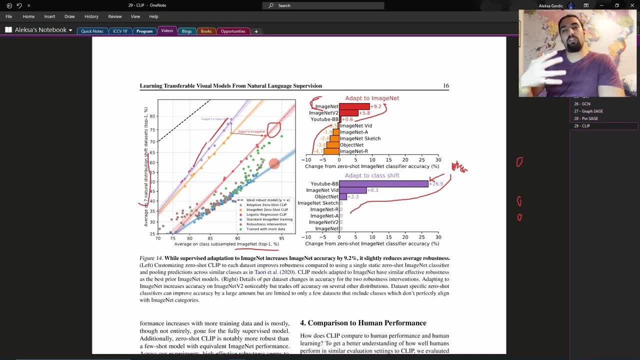 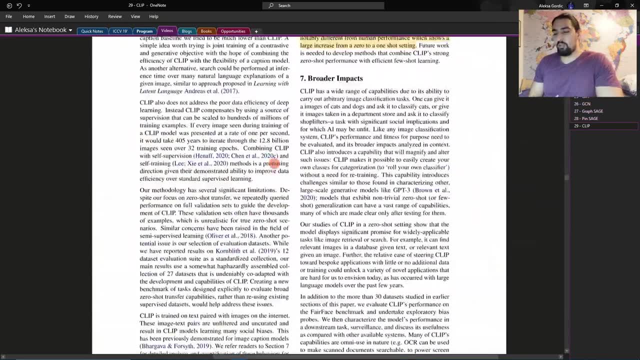 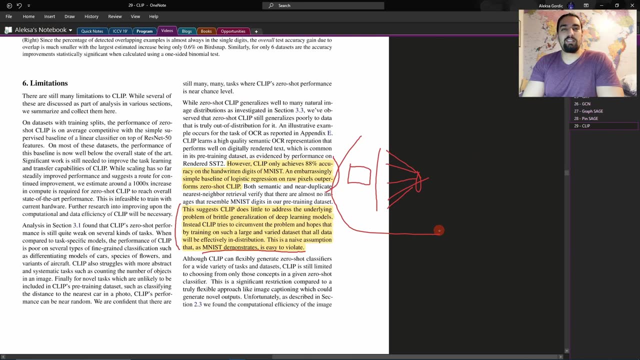 you basically do improve ImageNet performance, but you lose the robustness to other datasets, So you don't want to overfit to ImageNet. basically And finally, they showed some limitations, among them that it's failing on simple datasets such as MNIST, because it never saw those images during training.